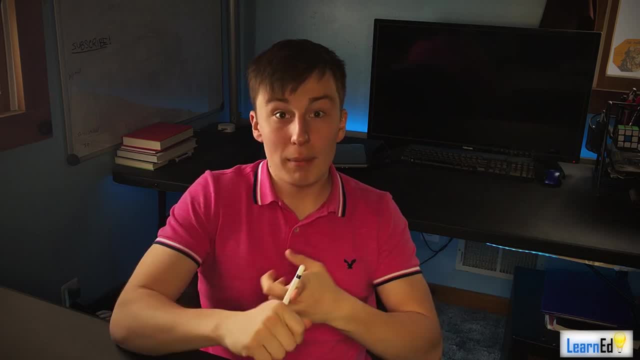 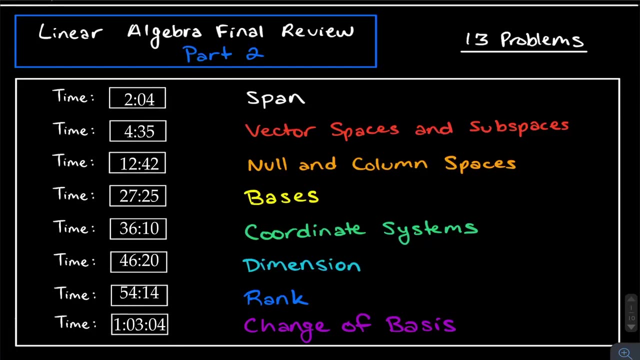 We're trying to hit 1000 subscribers by May, which is actually now next month, So hopefully we are going to be able to do that. Anyways, let's get into this video. So in this video we'll have 13.. 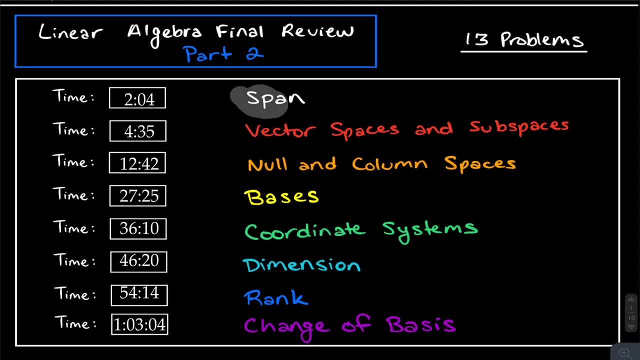 Problems. We will be starting off by talking a little bit about span, just getting comfortable with that concept. There's not going to be any problems included in the full 13 in that section, But I think it's definitely good to review that. span is something you have to deal with. 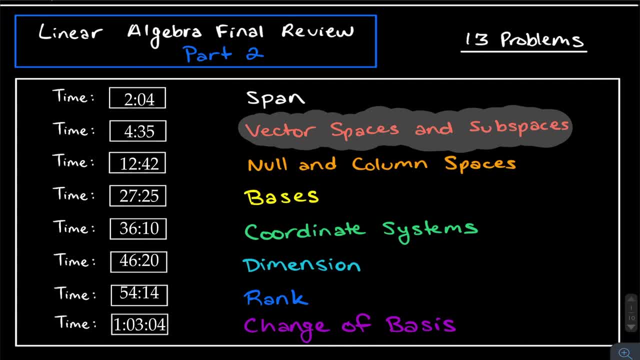 in things like vector spaces and subspaces, which is the next thing, next thing that we'll go over And we'll do a couple problems there. Then we'll move on to null and column spaces, followed by bases. We'll talk about coordinate systems. Okay, 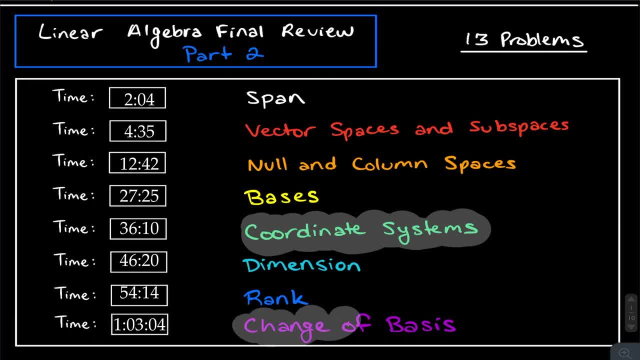 Then we'll talk about dimension and rank, And that will lead us into change of basis. Okay, Now we do have all the timestamps on the left, But if you are trying to jump right to change of basis, what I would recommend is first going and checking out the coordinate systems video. 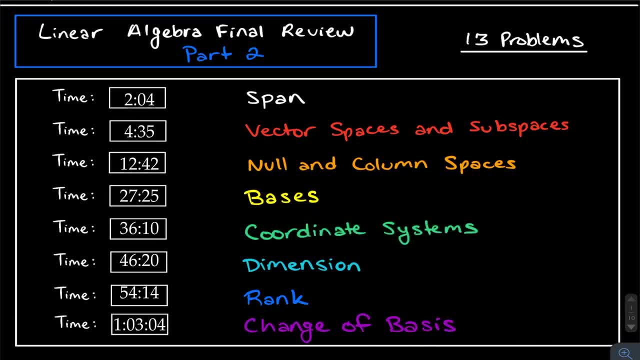 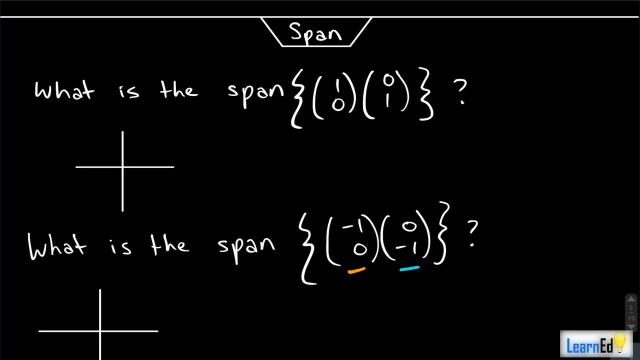 or the coordinate systems problems, because that is kind of the prerequisite to understand change of basis. So if you're not understanding change of basis, you most likely are confused about something in the core. So let's move on to our first section, that being the span section, And we're going to try to find 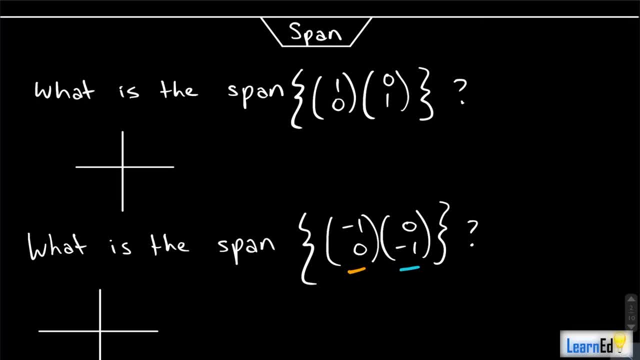 the span of these two vectors: one zero and zero one. Okay, and I'm going to label these guys, and that's the highlighter, not the marker. Here we go. So I'll label these guys. we have one zero and zero one And I'll graph them. one zero is over here. 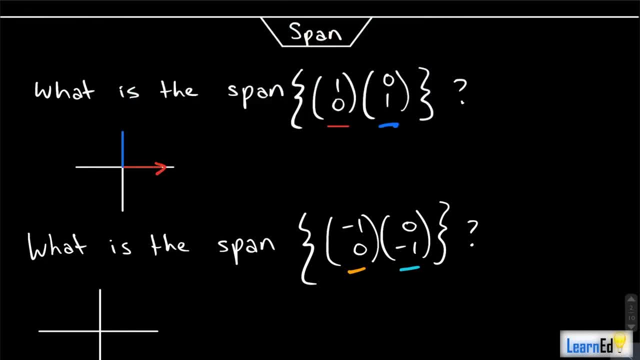 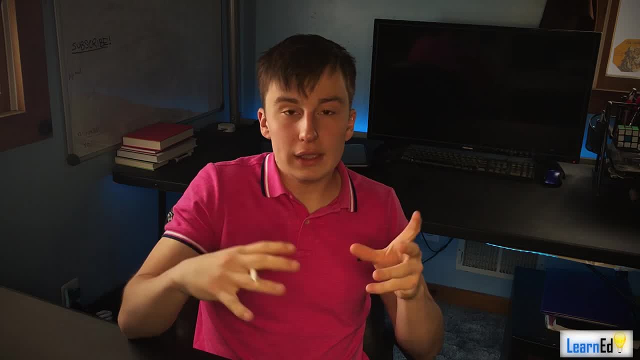 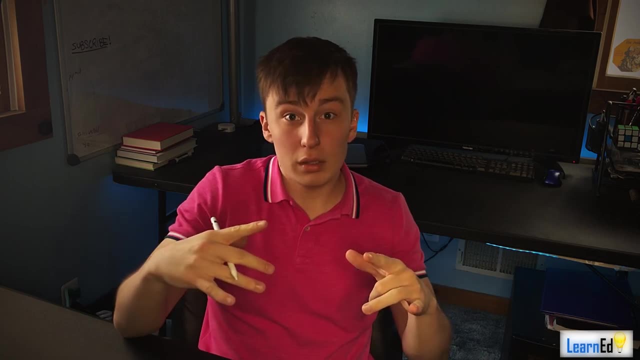 And then zero one is up here. Okay, Now, what these span of vectors are? right, it's kind of the. it's the set of all possible linear combinations of the vectors in the span, Right? So what does that mean? Well, here, right, like, first off, what is a linear combination? Well, an example. 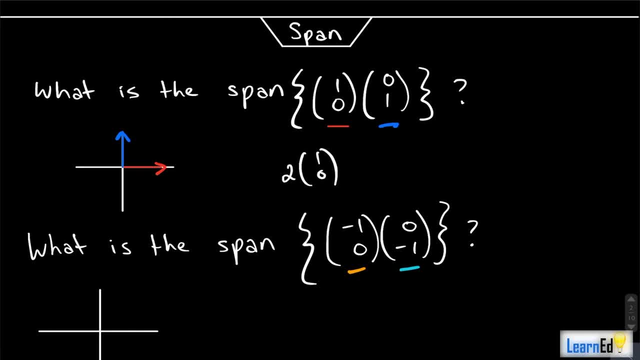 of a linear combination is like two times the vector one zero, plus a linear combination of two times the vector zero, one, right? So that's an example of a linear combination. Now we're saying, okay, what about all the possible linear combinations? we put an A here and a B here, Okay? 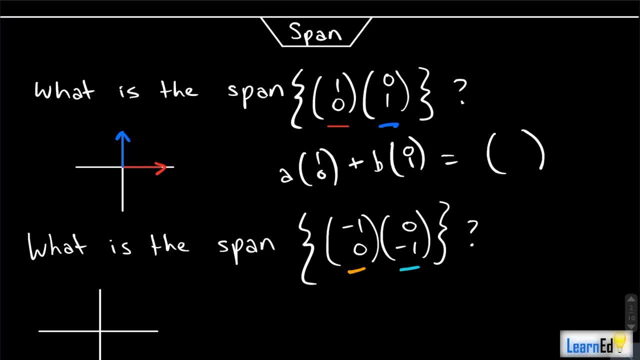 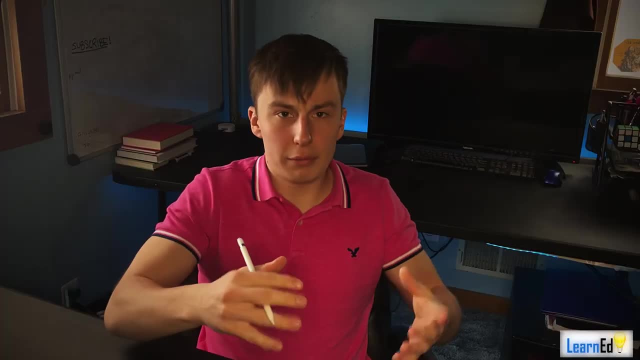 and we're trying to find the set of all these possible linear combinations. What does that represent here? Well, here it's the xy plane. right, You can? you can linearly combine these vectors to give you anything on the xy plane. Okay, you can get three, three, you can get six. 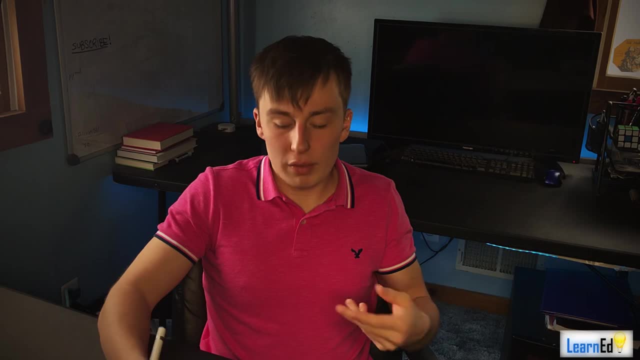 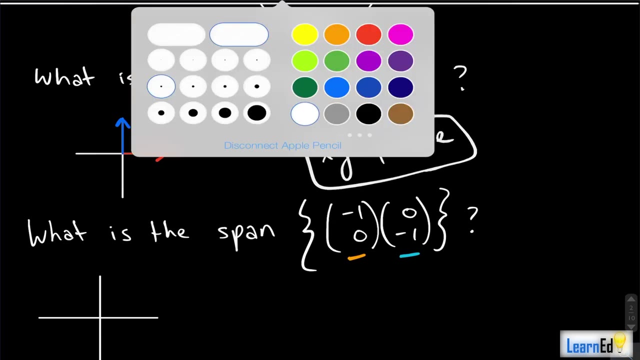 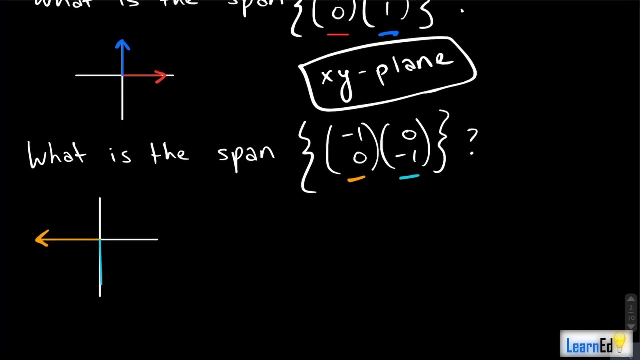 negative two and things like that. Right, So that's the idea of what we're talking about with span. Now we'll try this again With another problem. Here we have an- I already underlined these, So we have negative one, zero, And we have zero negative one. Oops, Okay, so there's. 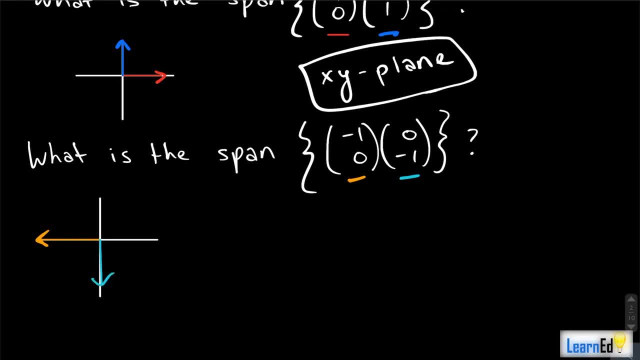 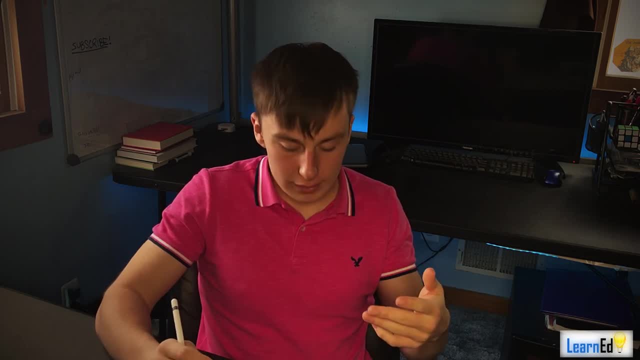 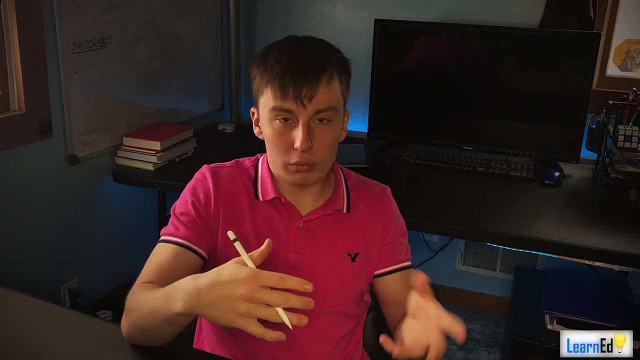 zero, negative one. Now, what's the span of these two vectors? What's the set of all linear combinations of these two vectors? Well, again, you can probably see that these are kind of just the basis vectors rotated right, And so we can, we can, you know. 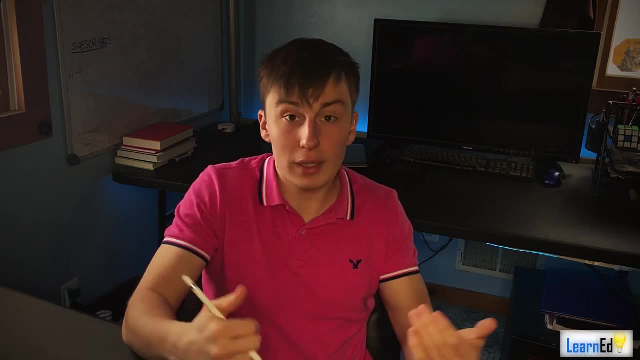 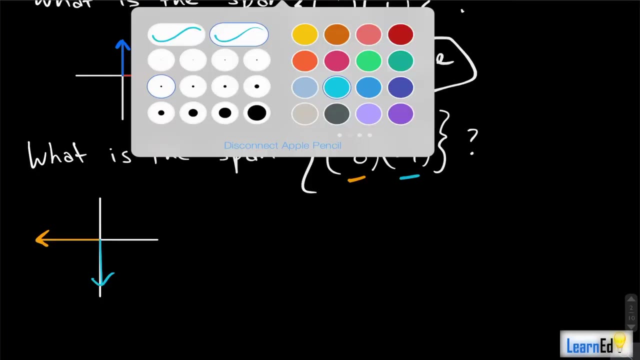 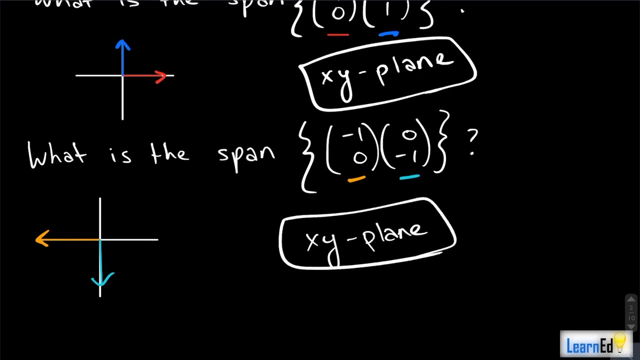 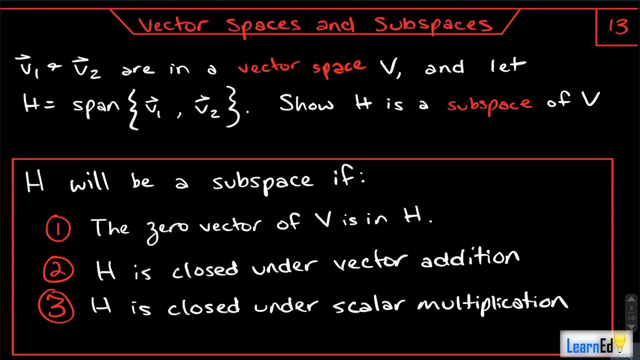 these are basically the same thing as the basis vectors. we can describe the entire xy plane again with these two vectors. Okay, so again, the span of these two vectors is the entire xy plane. Okay, And that's the idea with span. So now we're going to move on to our first question of this. 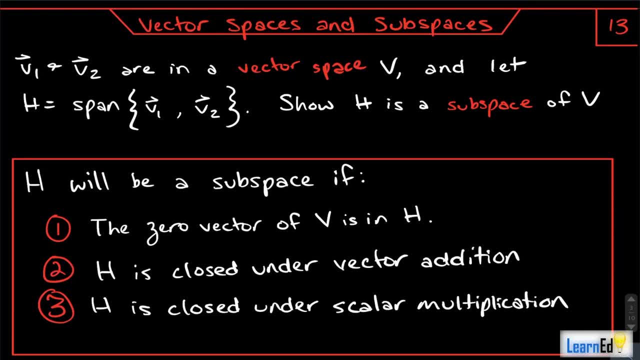 video And that's going to be on vector spaces and subspaces. Okay, now that is labeled as question number 13. Because it's going off of the last, the last video, which was ending on question 12.. And this question is asking: we have two vectors, v one and v two, and they're in a vector space, V. 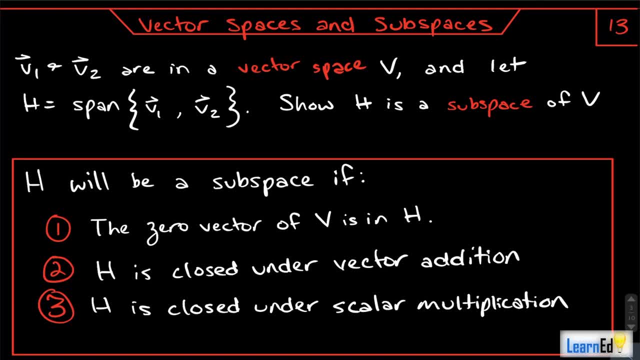 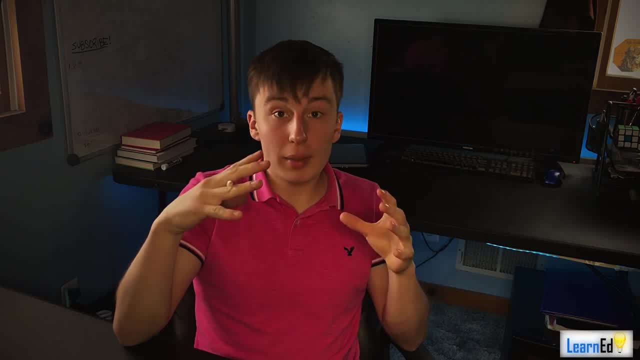 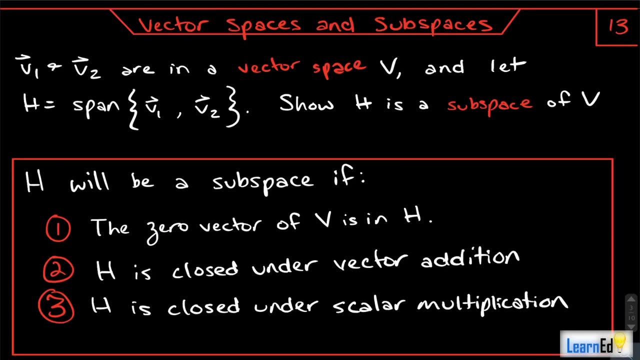 And we're letting h equal the span C, the spans popping up again right, the span of v one and v two. Okay, so H is all the possible linear combinations of v one and v two. That's what that means. And this problem is asking us to show that h is a subspace of v. Okay, 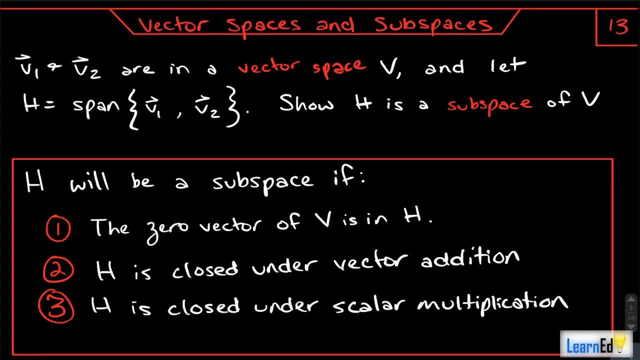 so, before I get into the criteria for subspace, I want to talk about what a vector space and a subspace actually are okay, because that's this is something that I definitely Okay. so, before I get into the criteria for subspace, I want to talk about what a vector space and a subspace actually are Okay, because that's this is something that I definitely. 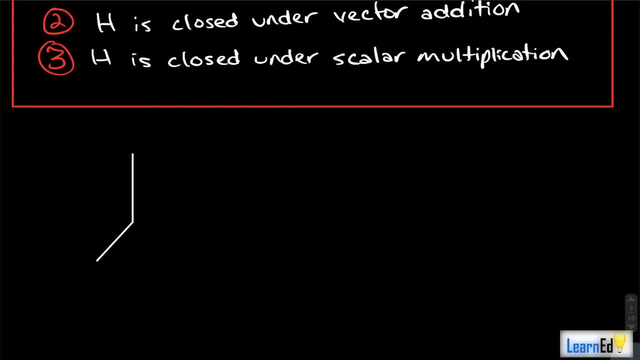 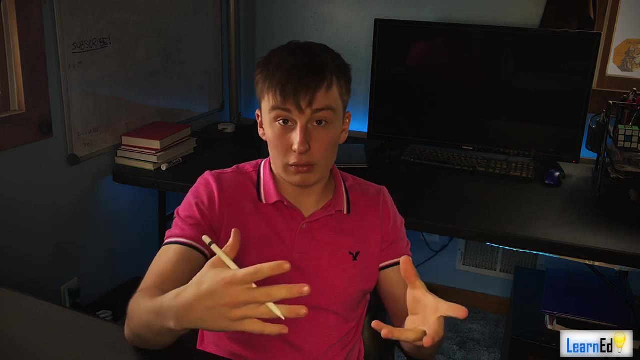 was confused on when i was in linear algebra. okay, so let's take, for example, a vector space: v that's in r3. okay, that's an. r3 is an example of a vector space, because it is a place where vectors can occur. right, that's a very simplistic way of putting it, but you it gets the point across you. 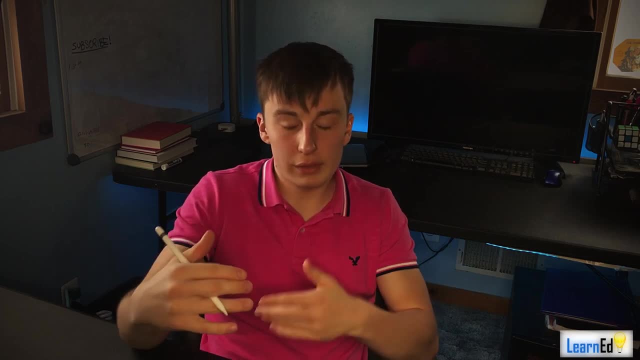 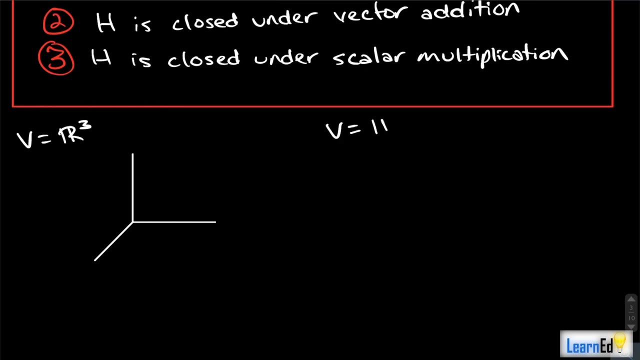 understand what i'm talking about right. r3 is a place that can hold vectors, now a you know. another example would be: you could describe a p2- i don't know how people you can maybe put it like that right. so we're talking about polynomials, which would also be three-dimensional. 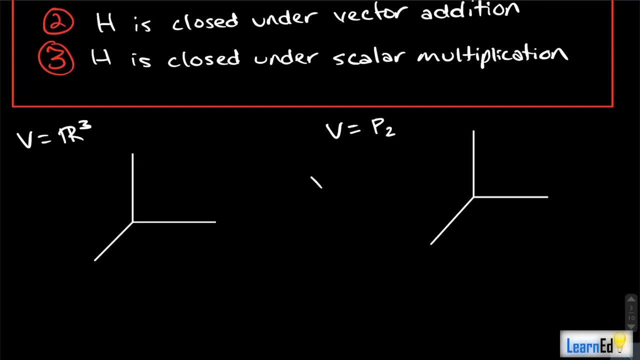 right, this is polynomials up to degree two, so we're kind of talking about like x squared plus x plus one. right, so we have an x squared term, a x term and a constant term. right, so you would have each of those on their own axes. So that's another example of a vector space, okay, And that's definitely one that you end up. 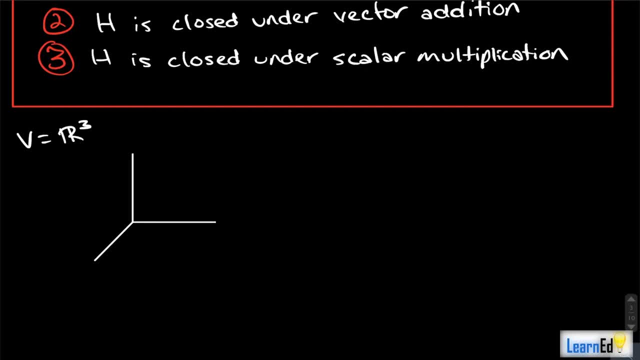 seeing right. The main two are, you know, like an R3, right, Where you have like XYZ or something like that, or you might have like a polynomial space, which is also very common. So we have this vector space R3.. What is a subspace of R3?? Well, if we label these as X1, X2, X3, right R axes. 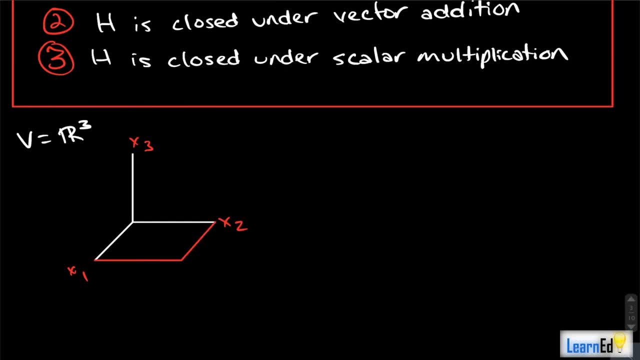 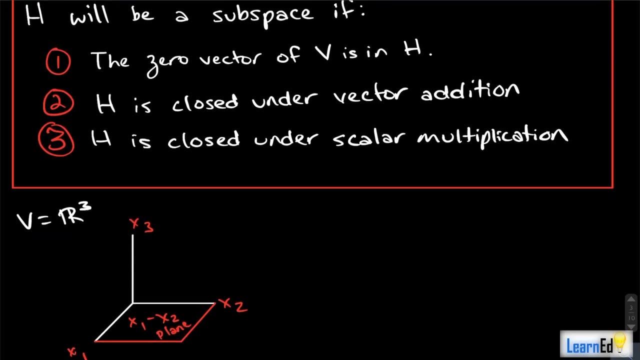 The X1, X2 plane qualifies as a subspace. okay, This is a subspace. okay, And why is this a subspace? Well, basically, you have that the X1, X2 plane qualifies as a subspace. okay, And why is this a subspace? 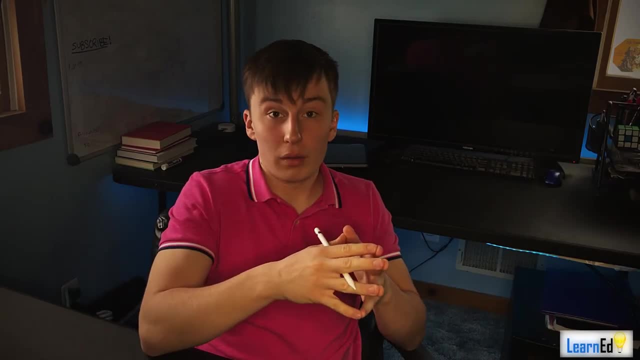 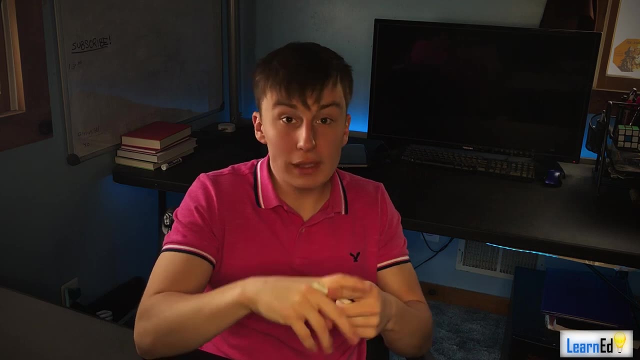 The X1, X2 plane is a subspace because the zero vector okay of R3 is in the X1, X2 plane, right, And the X1, X2 plane is also closed under vector addition. Think about it. There's no Z. 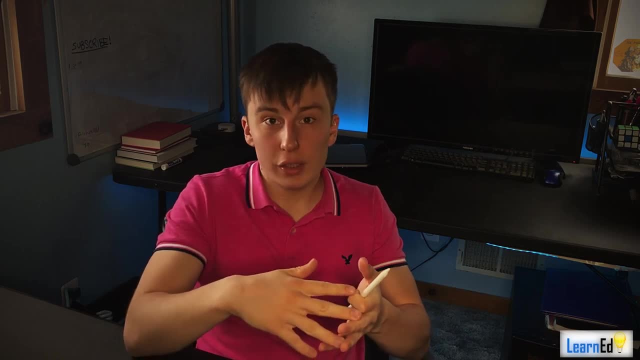 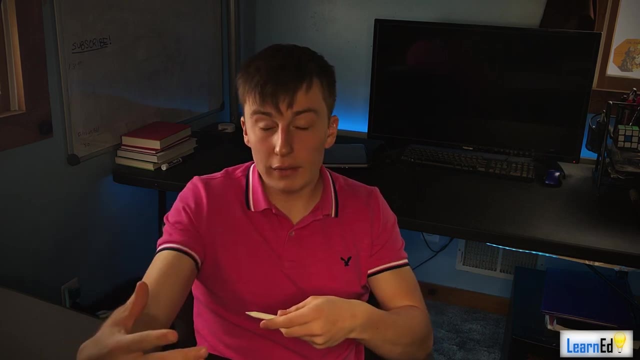 component right, Or there's no X3 component. So if you add two vectors, two random vectors in the X1, X2 plane together, you'll get another vector in the X1, X2 plane. If you do, it's also closed under scalar multiplication, right? That's our third. 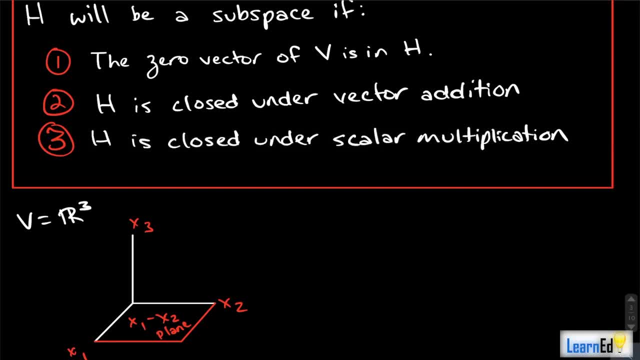 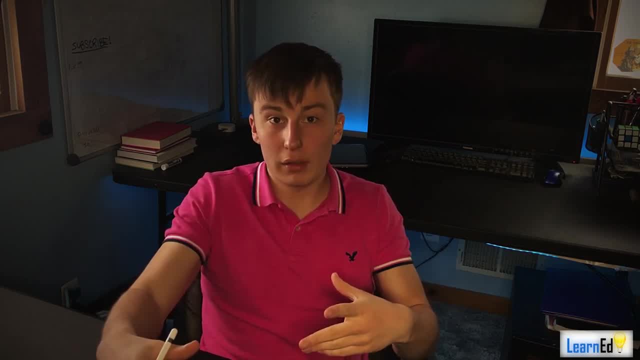 vector. So if you add two vectors to random vectors, you'll get another vector in the X1, X2 plane. point, okay. so if you have some vector in the x1- x2 plane and you multiply it by a constant, you'll get another vector in the x1- x2 plane. and that is the criteria. 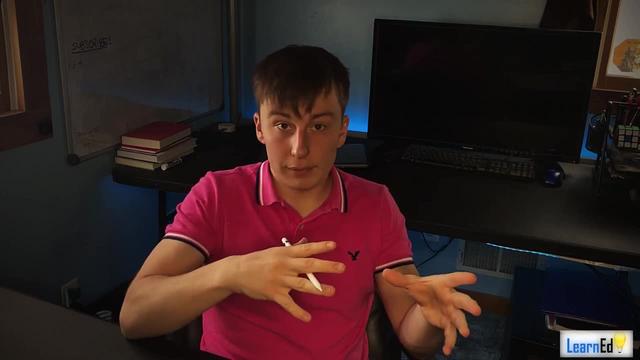 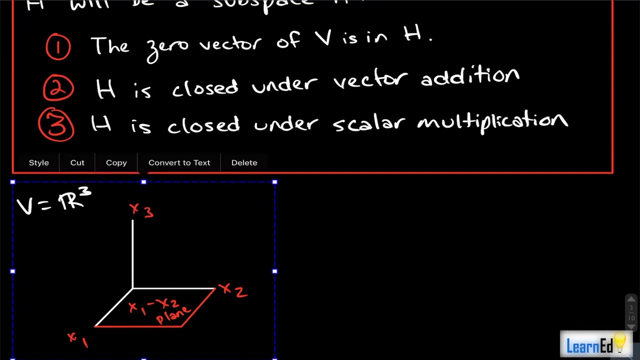 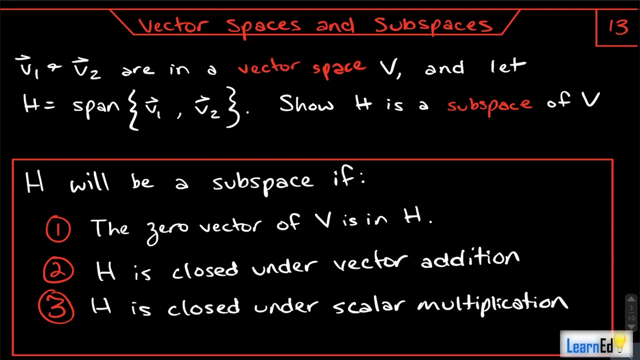 for something to be a subspace of a vector space. okay, so, with that being said, we're able to move on to our actual problem, which is to show the H is a subspace of V, where H is the span of V 1 and V 2. so let's start off with our 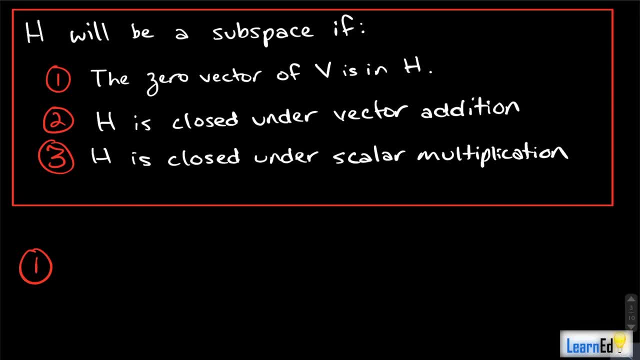 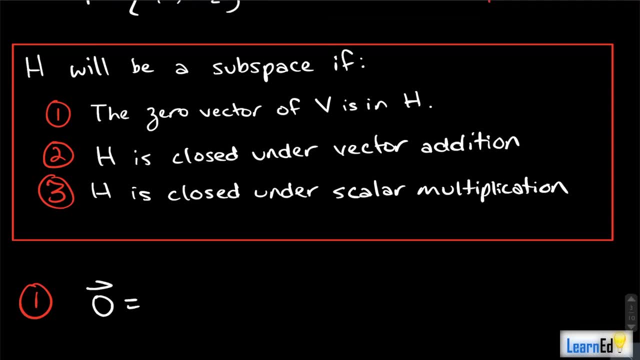 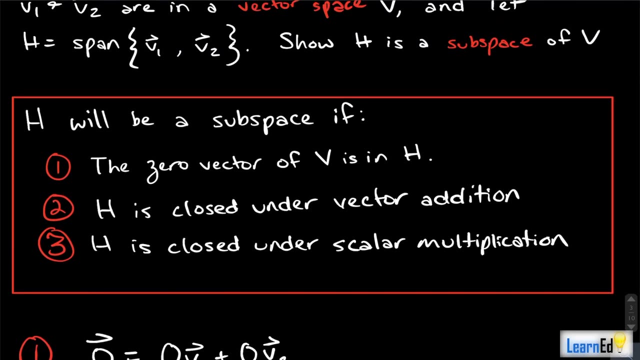 first criteria right, which is that the zero vector of V is an H. well, we can figure that out pretty simply, because we can just multiply 0 times both vectors, right? that works, because H is the span of V 1 and V 2, right? so it's all the. 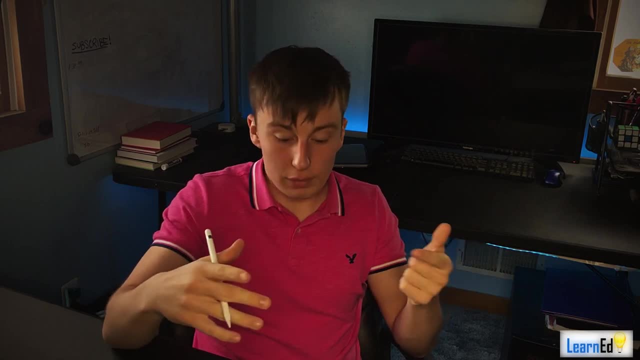 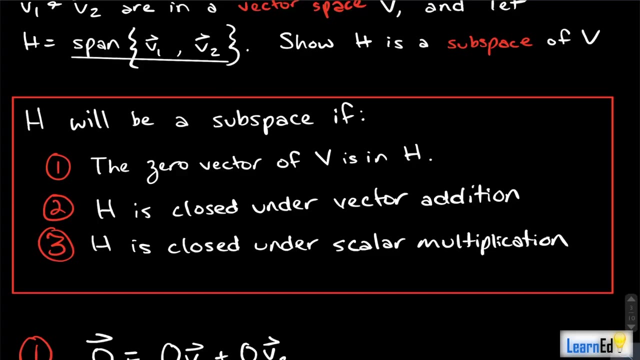 problem is that we can just multiply 0 times both vectors. right, that works, because H is the span of V 1 and V 2, right, so it's all the problem. possible linear combinations. that includes when, V what? when you have a 0 as the, the coefficient in front of V 1 and V 2, right, so that works. now what? 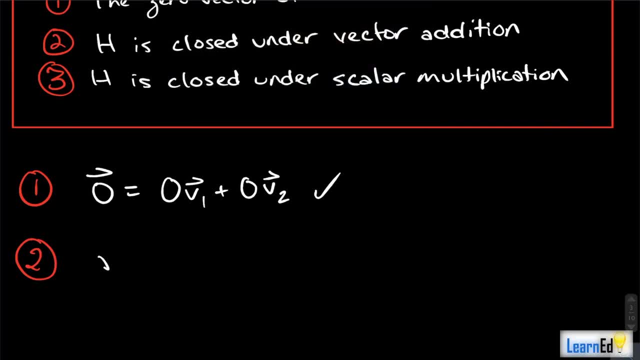 about being closed under vector addition. well, let's pick two arbitrary vectors and to ensure this, what we're going to do is define two new vectors, a and B. okay, make that look a little nicer. and these are just going to be linear combinations of V 1 and V 2. okay, now to give you a. 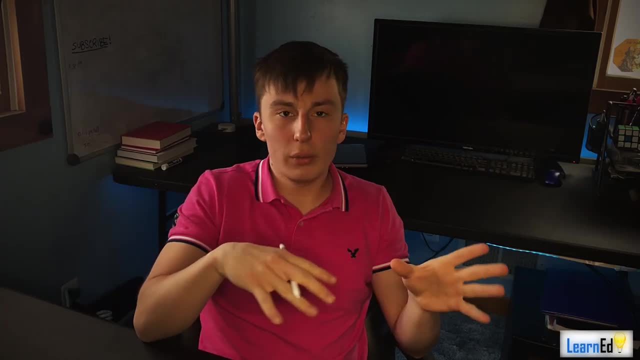 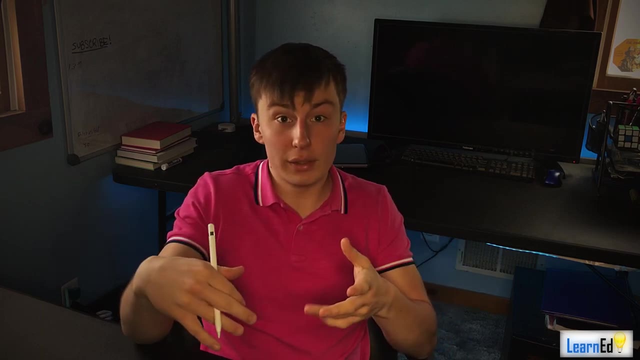 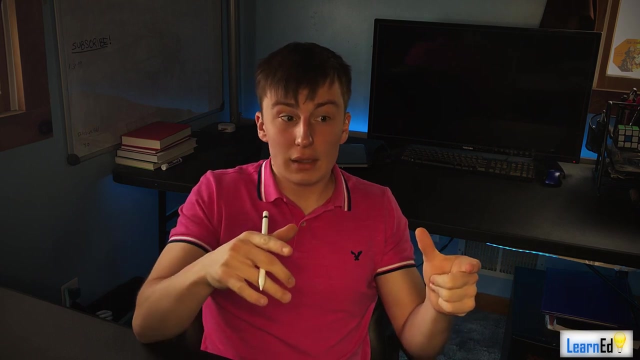 reason, you know. why are we? why are we including, like the s1, s2, the t1, t2? why are we doing two new vectors? why are we not just adding V 1 and V 2 together? right, we're doing this in order to more easily show that we can take any vectors in the span of V 1, V 2, right we? 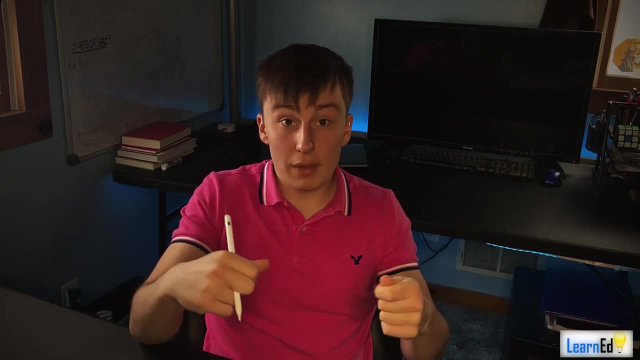 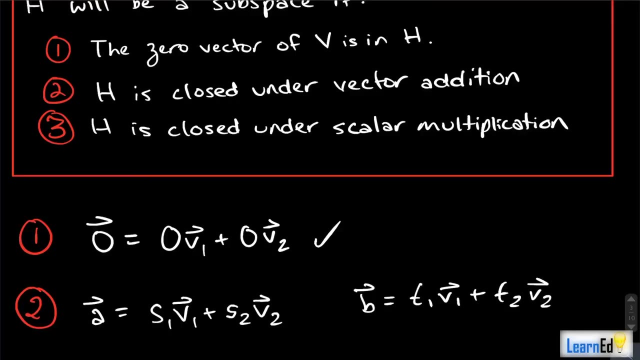 can take any vectors in in this span and we can add them together and get another vector that's in the span of V 1 and V 2. all right, if you think about it, it starts to make sense, right. a and b could be any vectors in V 1 and V 2. 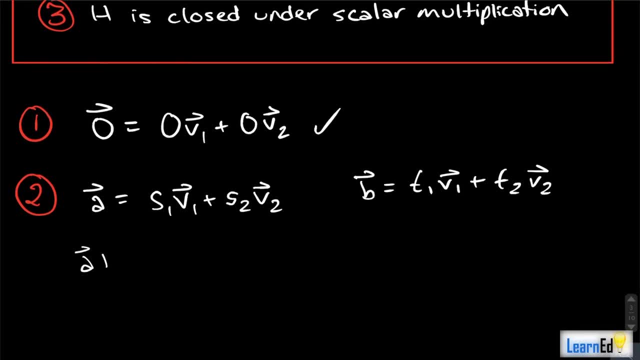 okay, it's just an easier way to show that. so if we add these two vectors together, a plus b, we get s1, v1 plus s2, v2 plus t1, v1 plus t2, v2, which we can simplify to be s1 plus t1 times, v1 plus s2 plus t2 times. 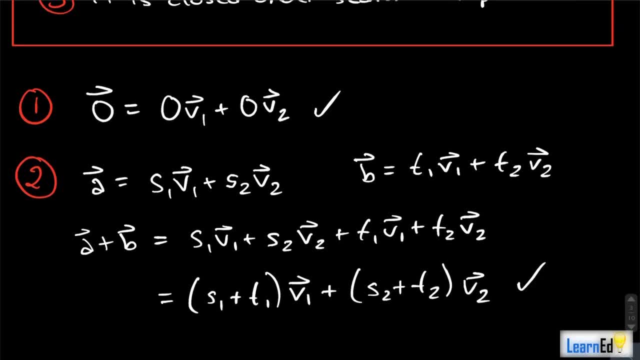 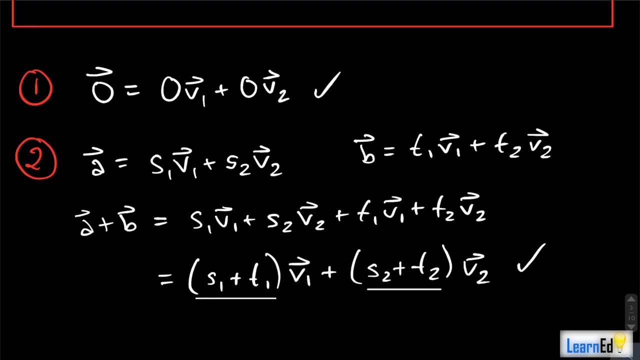 v2. okay, now this checks off. but why this checks off? because s1 plus t1- right, these are both constants. you add them together, you get another constant. same thing happens for s2 plus t2- right, you get a constant. so you get a linear combination of v1 and v2 as your answer. 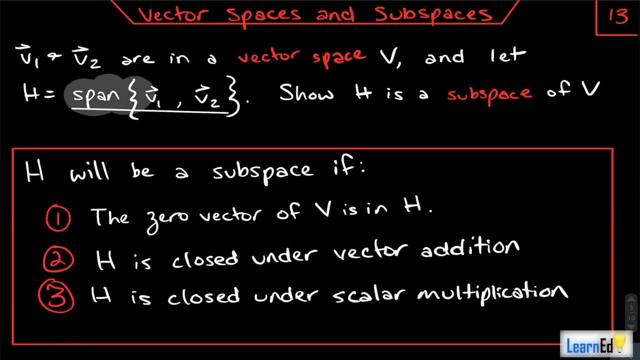 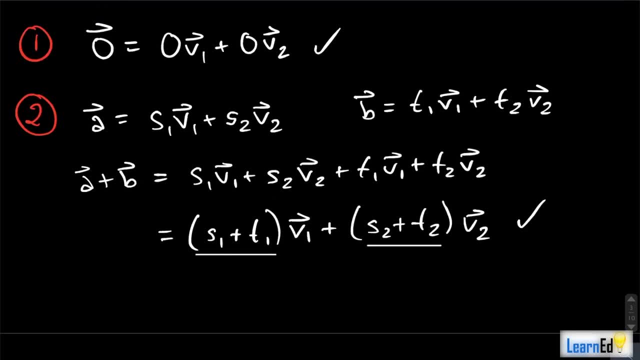 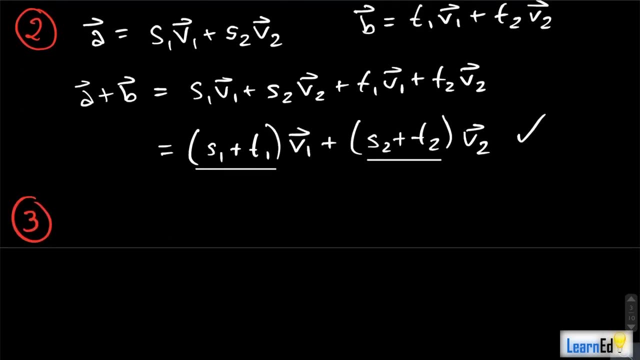 right, which makes sense because that's in the span of v1 and v2. so that works right. h is closed under vector addition and we can move on to our last criteria, which is to prove that h is closed under scalar multiplication. so let's just multiply. 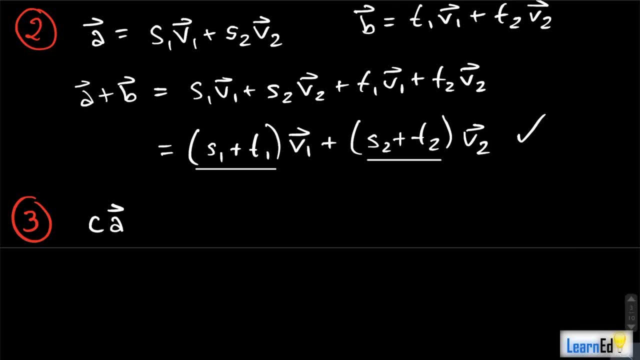 a. we'll multiply the vector a by some constant c. what do we get? well, we get c times s1 v1 plus s2 v2, which we can write as c times s1 v1 plus c times s2 v2 off. why? because c? s1 is still a constant, c s2 is still a constant, all right, and you're multiplying. 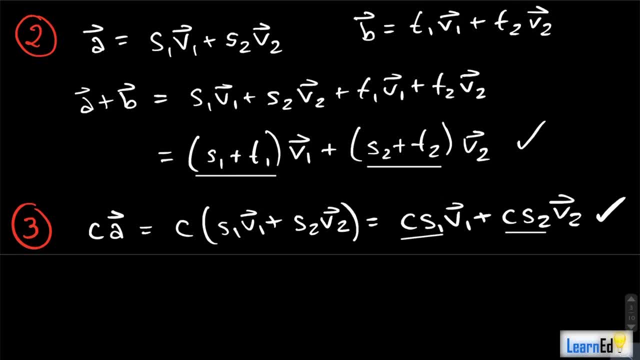 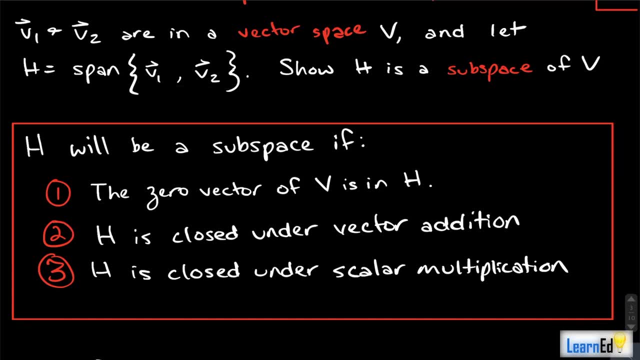 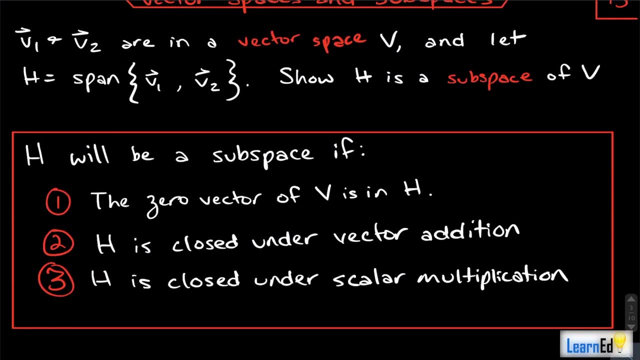 that in on v1, v2, that's just a linear combination of those two vectors and that would be in the span, right, because that's the definition of what the span of of these two vectors means, right? so, since all all these three criteria are met, we know that h is a subspace of V. okay, so H is a subspace of. 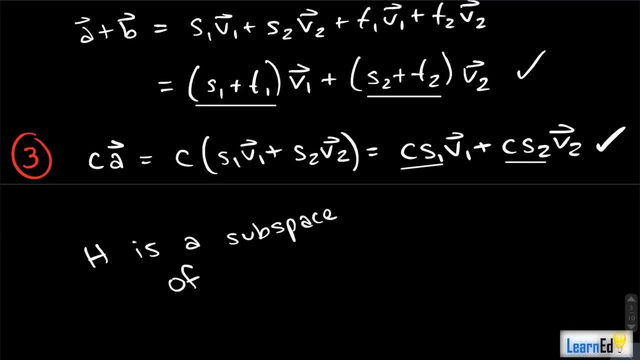 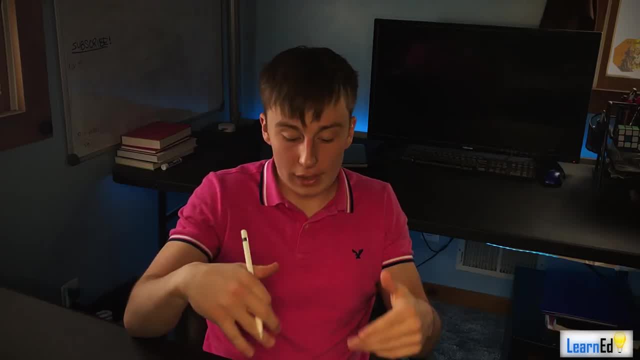 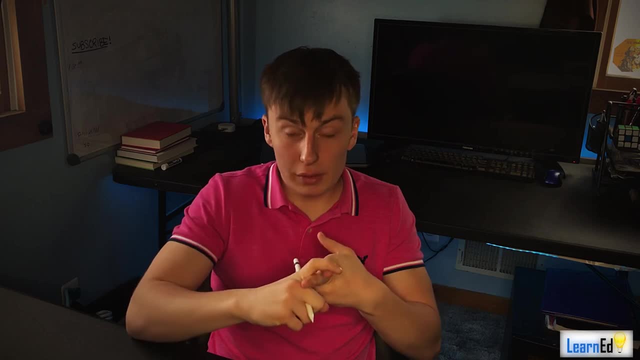 V. okay, and that is not how I would write that on a test. how, on a test, I would just say H is a subspace of V because the zero vector of V is an H. H is closed under a vector addition and H is closed under scalar multiplication. that's how I would write that out. you would write out the three. 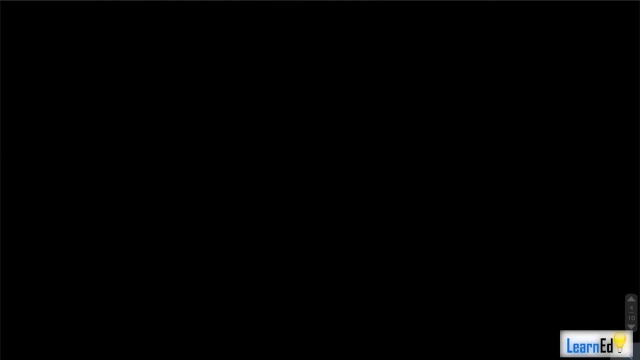 criteria in your answer. I just want to move on to the next problem. so now we're going to move on to our next problem, which is on null spaces and column spaces. okay, this is problem 14 and it's asking to find the null space of a. 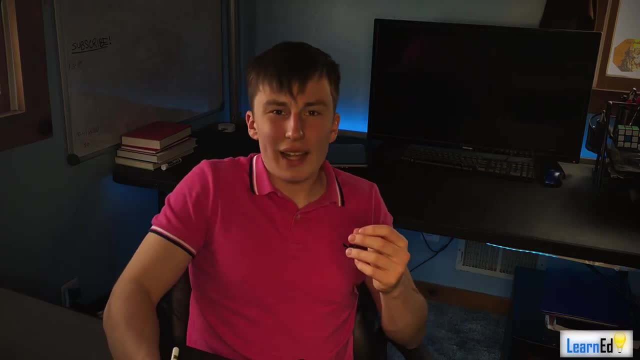 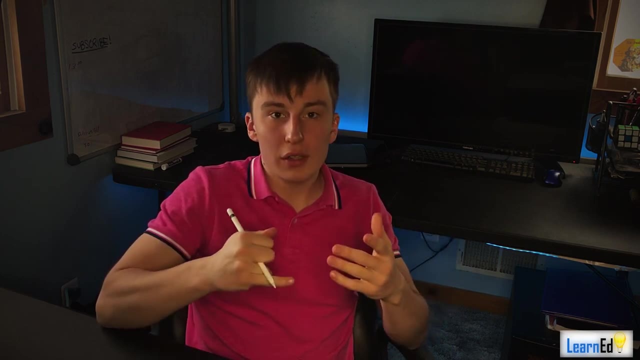 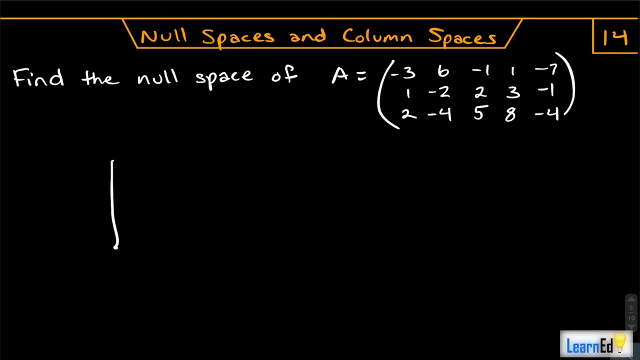 which is a 3x5 matrix. now, what actually is a null space? okay, that's probably the initial question that you should be asking, because if you know what a null space is, you'll understand more of how to find it. okay, the null space. to describe the null space, let's just say that we have a 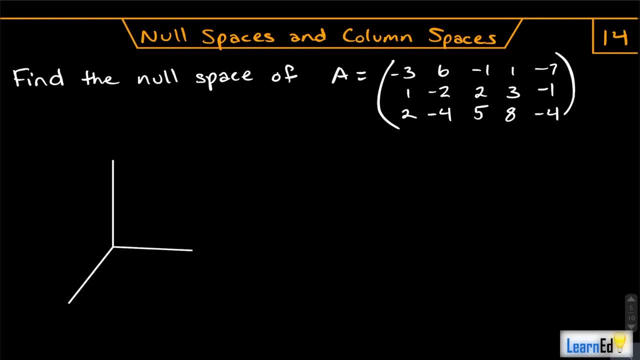 linear transformation that's transforming vectors from R3, okay, and it's transforming them again into R3. we'll keep it simple here. okay, and let's say that we have this line of vectors here, okay, so it's a line of vectors that just connect to this line, right? so these vectors describe that line, and let's say that when we do. 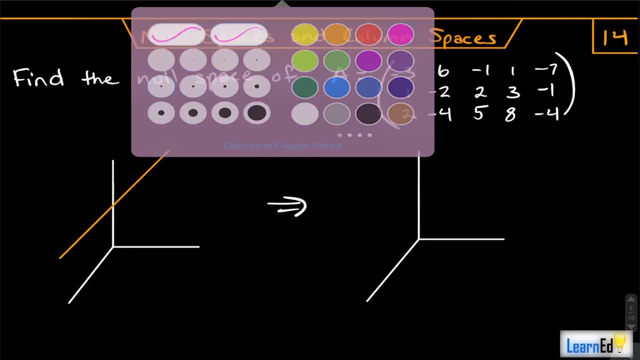 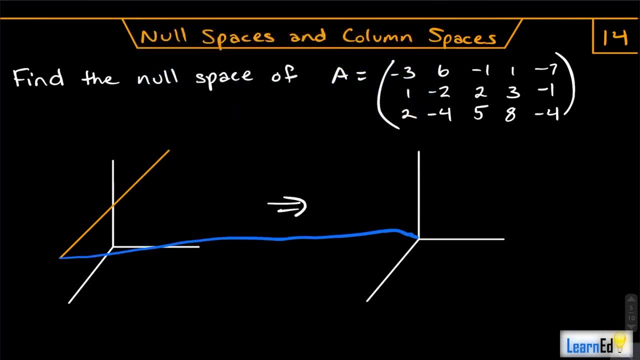 our linear transformation. okay, what color goes good with the orange? let's go blue, okay. so when we do our linear transformation, all of the vectors on that line go to zero. okay, they all become zero. okay. so the null space, okay, of this transformation Matrix. okay, so null of a is. 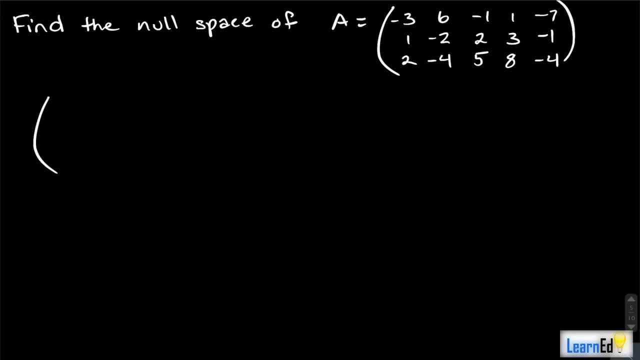 so how we're going to find this actually is: we're going to have to row reduce here, and and so I'm going to start off by just swapping rows. okay, because I want to get that one in the first pivot. okay, because that's just going to be a lot easier to deal with. 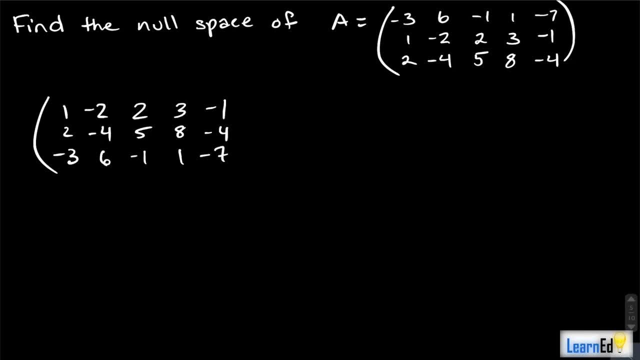 okay. so I've finished swapping Rose and what we're going to do now is we're going to augment this Matrix with, with zeros, and we're going to row reduce, because what we're trying to find here, okay, is we are trying to find the vectors right, the, the span of vectors that will go. 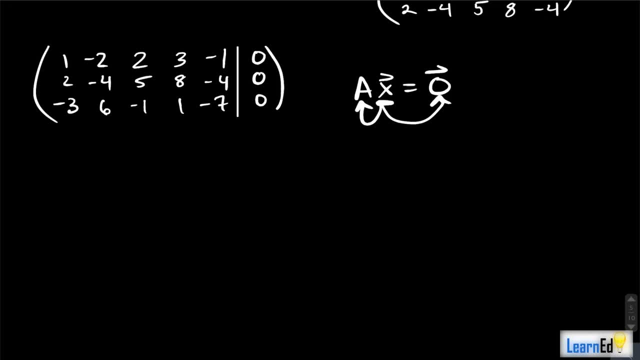 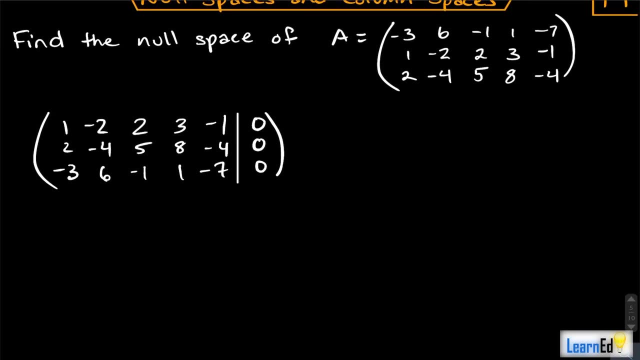 to zero. when the linear transformation is applied, okay, that's find the vectors right- okay. so when the linear transformation is applied, okay, that's why we're doing this. so we're reducing here. I want to get first off, I want to keep the first row the same and these zeros, no matter what we do, these zeros will stay zeros because you. 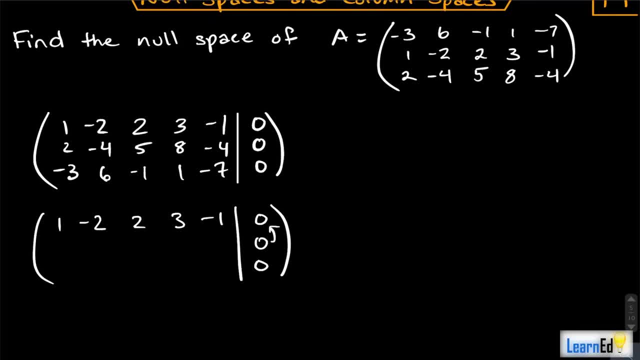 can't do. you can't multiply a zero by anything and add it and have it be anything other than zero, right? so what we're gonna do here is we're gonna make these two things zeros. we're gonna make the the entries in the first column under the pivot zero, and to do that in the second row. 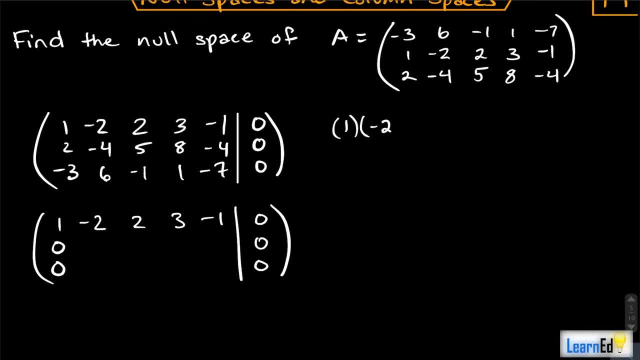 we had to multiply the one by negative two. when we got negative two off of that, we added to the entry in that row and we get zero. so that gives us our zero here. now we'll do that for the other entries across the first row. so we'll start off with that negative 2 multiply. 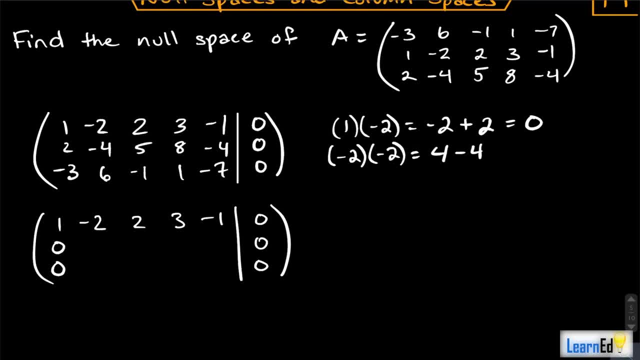 by negative 2 get 4. we subtract by the 4 that's already in the second row and we get 0. so we get a 0 here. we can do that for the 2 in the first row. we get negative 4, we add 5, we get 1. we can do 3 times: negative 2: get negative 6, we add. 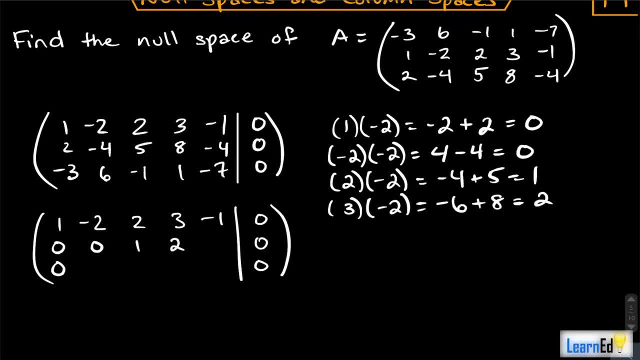 8, we get 2. and then, lastly, we have a negative 1 times negative 2. we get to subtract 4, we get negative 2. okay, I'm assuming that you guys are, you know, comfortable with row reducing, so I am trying to go a little bit quicker all. 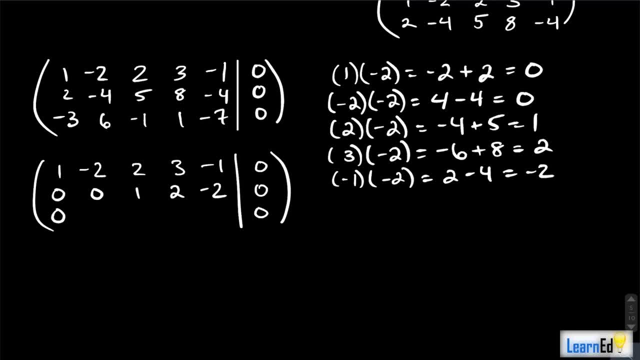 right, so I'm going to go ahead and do that, and then I'm going to go ahead, and I'm going to go ahead and do that, and then I'm going to go ahead and do that. right? so now for the third row. we have to multiply by 3 and add, so we can do. 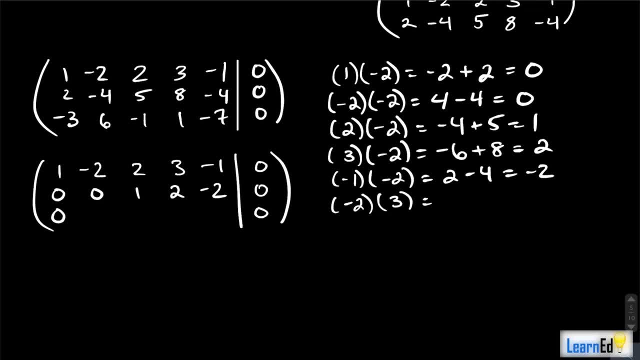 negative. 2 times 3 is negative. 6 plus 6 is 0, we'll have a. 2 times 3 is 6 minus 1 is 5. we'll have a. 3 times 3 is 9 plus 1 is 10, and then: 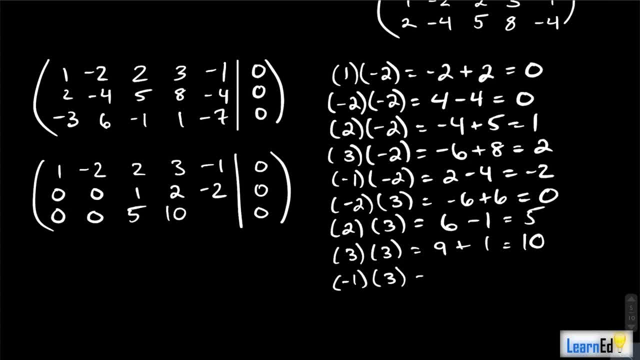 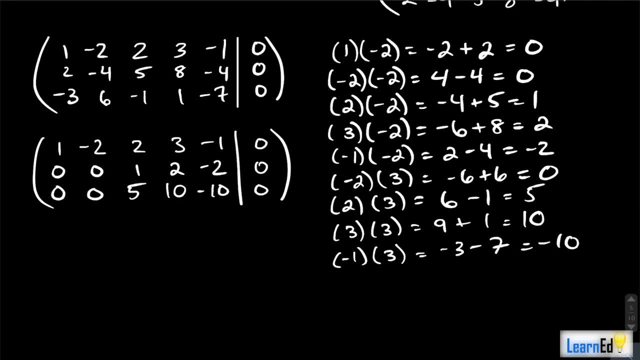 we have a negative 1 times 3 is negative. 3 minus 7 is negative 10. okay now, as you can see, this third row is a scalar multiple of the second row, so what we're going to do is just 0 the third row out, right. 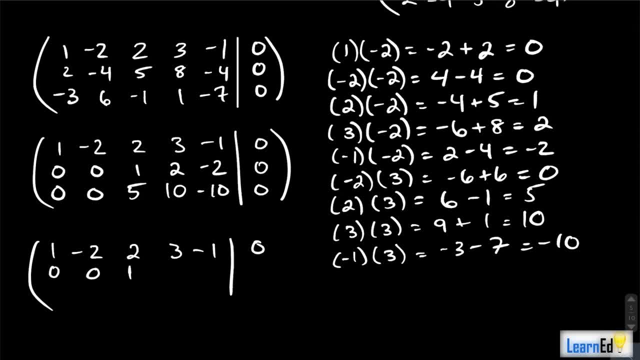 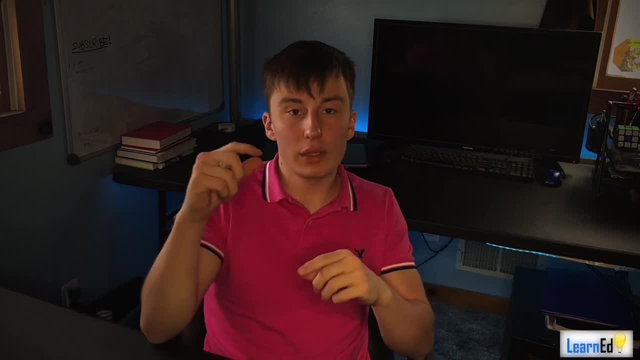 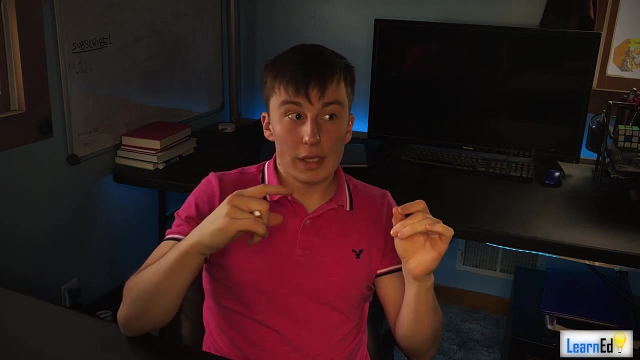 you okay, and now that we've done that, we actually only have one more step left, and that's to 0 out. we have two pivots at this point. we have two nonzero rows left, and so we have two pivots. now what we have to do is just get the nonzero. 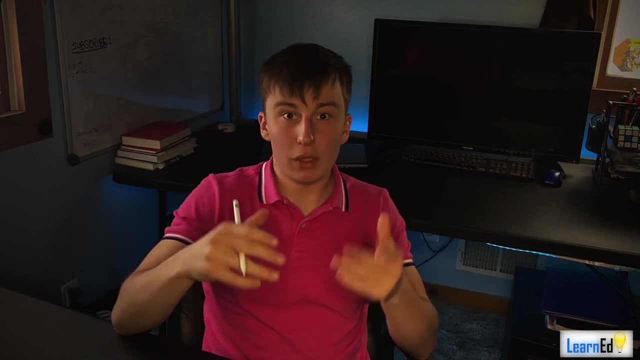 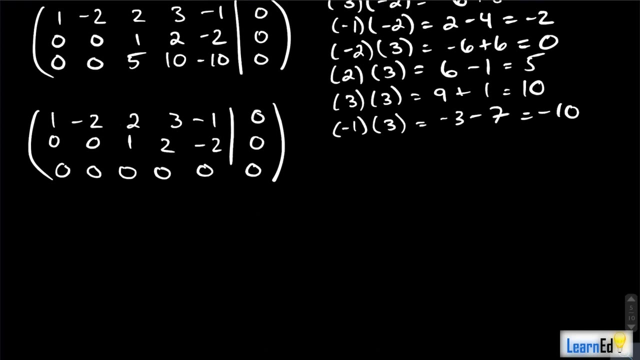 entry above the second pivot to be 0, and then we're done row reducing. So we're going to do that Okay, and we can actually go and create our span. this is that entry that we have to deal with because this is our pivot: 1 negative, 2, 0 and, by the way, I know that 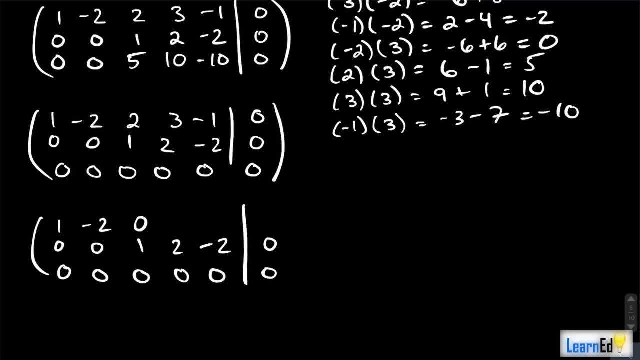 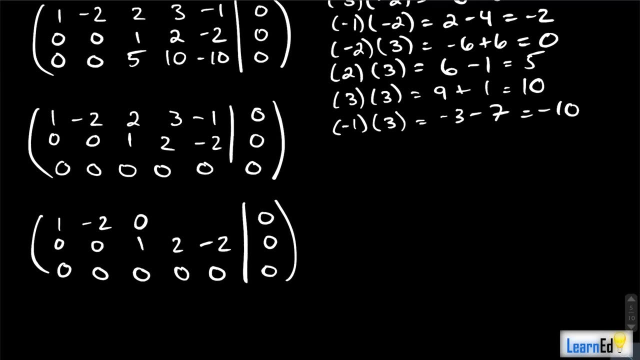 that these two entries will stay as 1 and negative 2, because these are zeros and when you do any transformation, the zeros won't make a difference, right? so to get this thing to be 0, we had to multiply the 1 by negative 2 and add, so we can apply that for the rest of the entries we have. 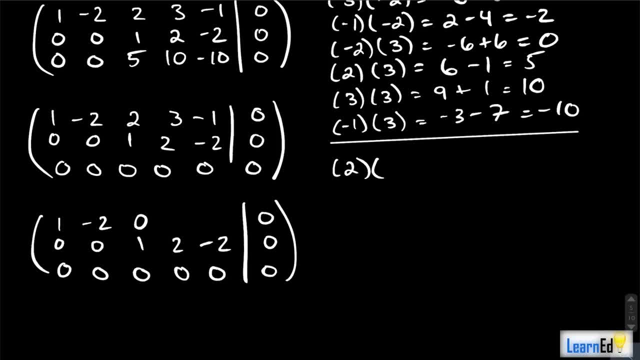 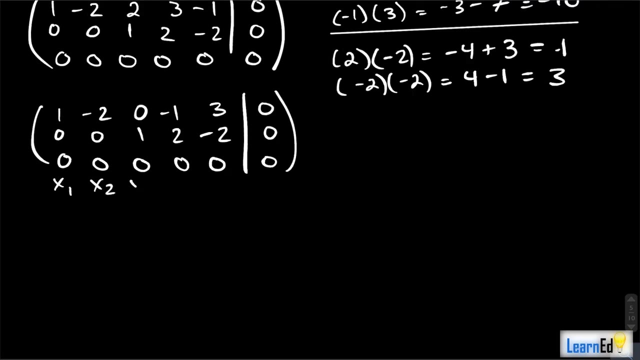 a 2. this 2 times a negative. 2 get a negative 4. we add on to 3, we get negative 1. then we have a negative 2 times negative 2, we get 4. we subtract 1, we get 3. let's call this column x1, we'll call that x2, x3, x4 and x5. okay, and we know. 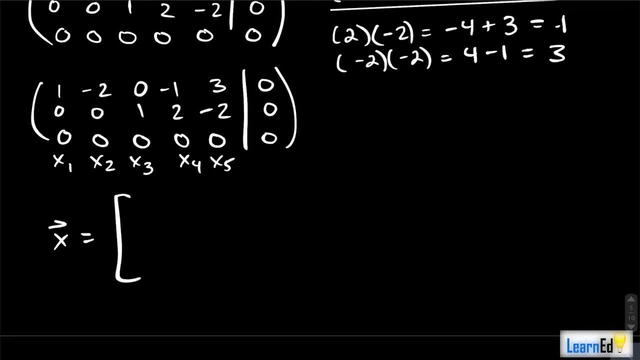 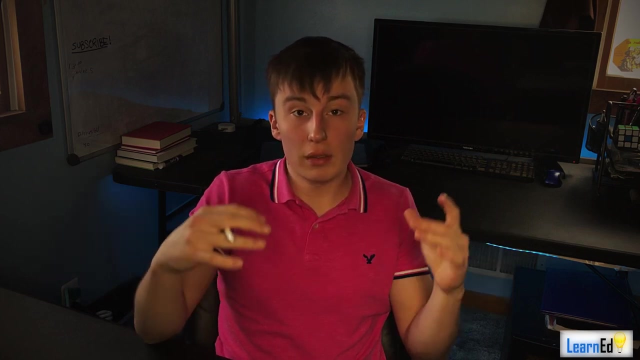 that this solution vector, this X is equal to these vectors, are represented as a column vector, right? so what is x1? well, x1, first off, it's not a free vector variable, right? our non-free variables are x1 and x3. so those are going to be. 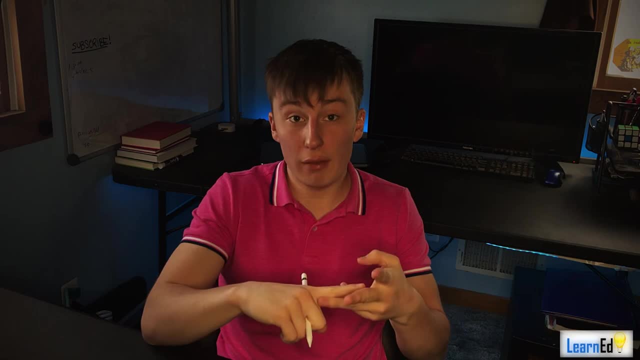 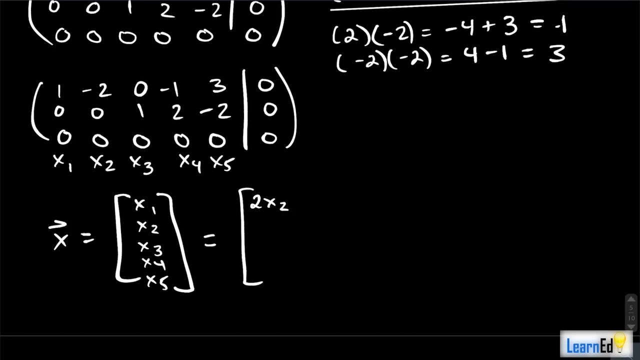 described in terms of the free variables, which is x2, x4 and x5. right, so x1 is it going to be equal to 2, x2? right, we flip the signs of all of them, because they'll get added or subtracted to the other side. we'll have plus x4 and then we'll 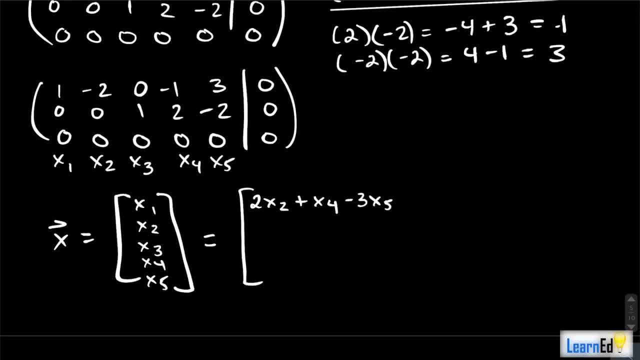 have minus 3 x5. for x2, that's a free variable, so we're just going to write it as such. for x3, that is a non-free variable. okay, so it'll be equal to negative 2x4 plus 2x5, and then. 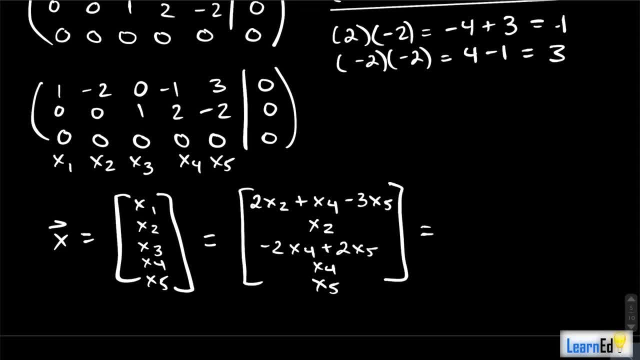 x4 and x5 are free, so we just write their own values down. so we're going to break this up and write this as x2 times 2. 1 and x2 is not present in these vectors and these and these guys right here, so 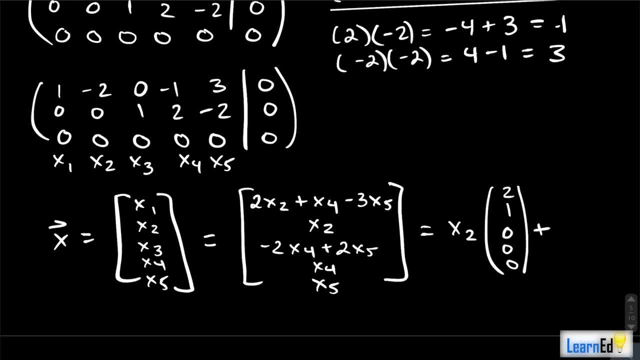 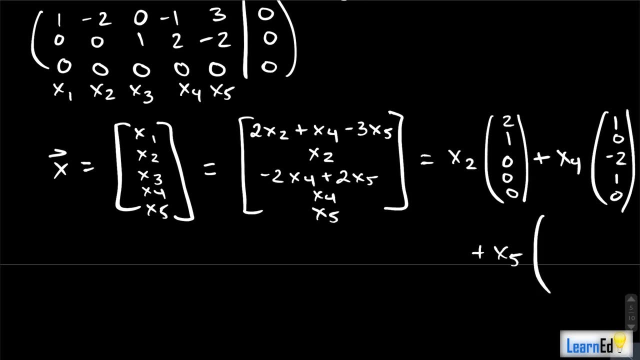 we'll just put them as zeros, right, because x2 doesn't appear there, and we'll do the same for x to the 4 or x4, so we'll get 1: 0 negative, 2, 1, 0, and then we'll do the same for x5- negative, 3, 0, 2, 0, 1 right. and where I'm getting all those? 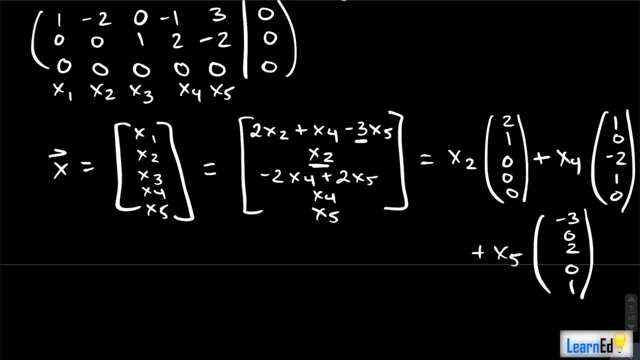 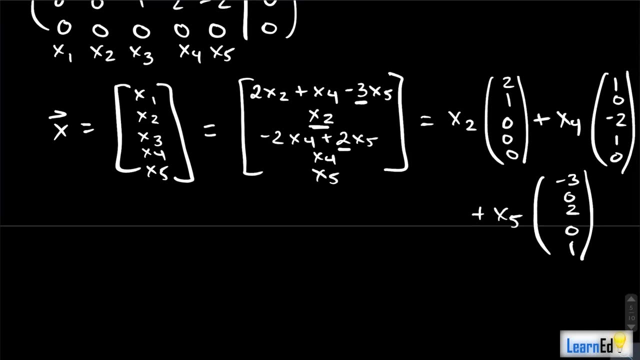 numbers from: for x5 negative 3 right here. there's no x5 here. there's a 2 there of x5, so that's the two there. there's no x5 here and there's one x5 here. okay, so that's where those come from. now, the span of these vectors that we just found. 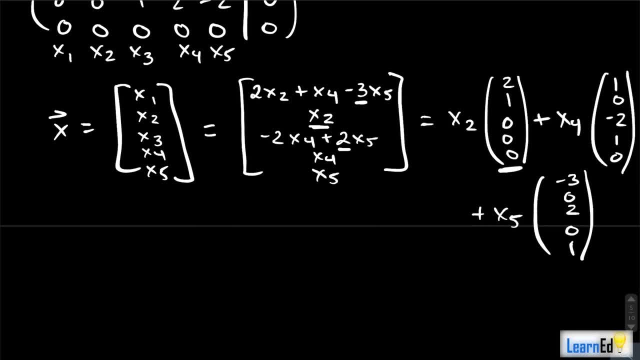 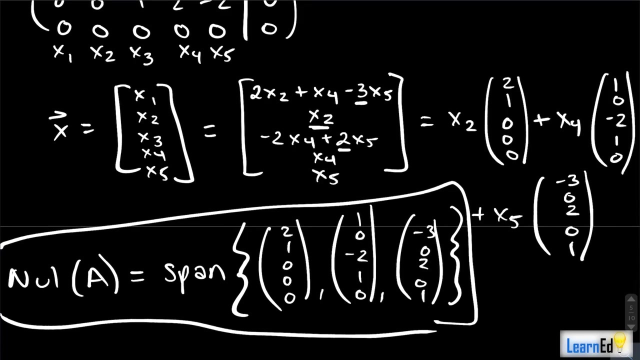 this, this one, this one and this one, that's our null space. right, because the linear combination, okay, the linear combination, these vectors, okay, any linear combination will go to zero when you apply the transformation. okay, and we describe that that space, okay, that space in our three, it doesn't have to be a line, it could be a plane, it could be the. 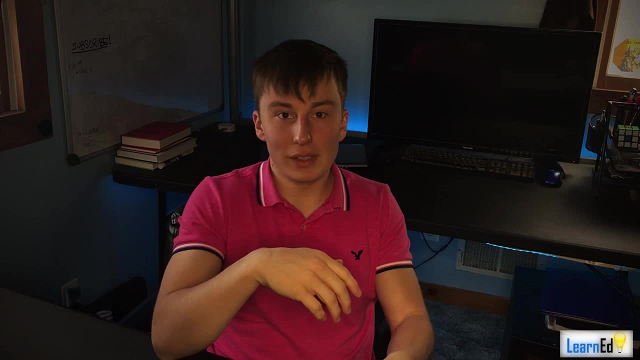 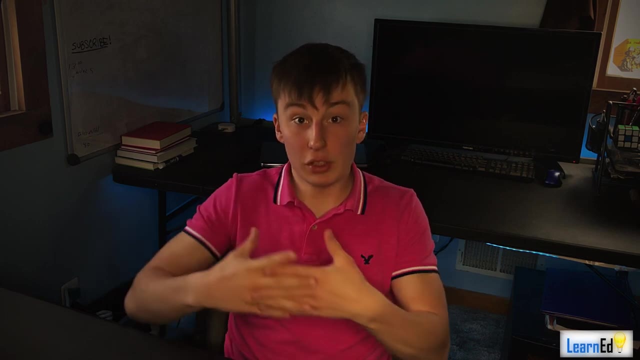 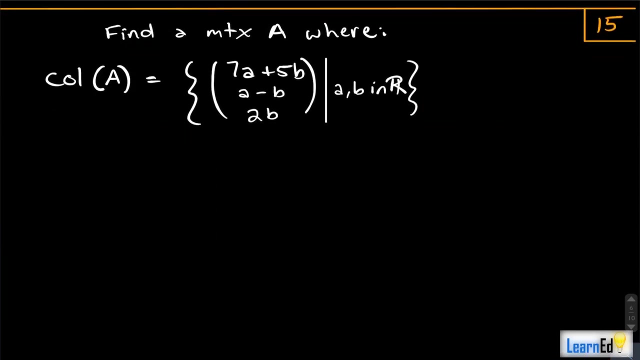 entire r3, maybe I don't know like, I'm just kind of putting some examples out there, right, and this entire space goes to zero. okay, so we describe it with a span. that's the null space. so now, moving on to problem 15, we're talking about the 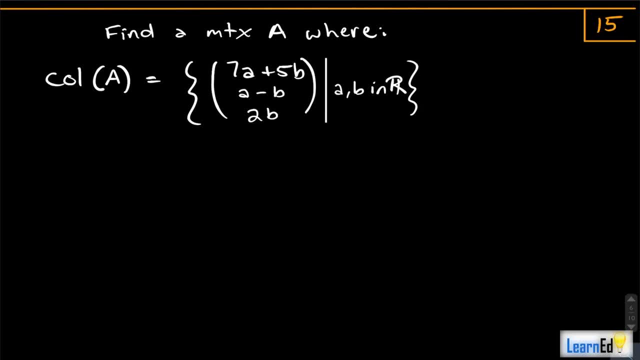 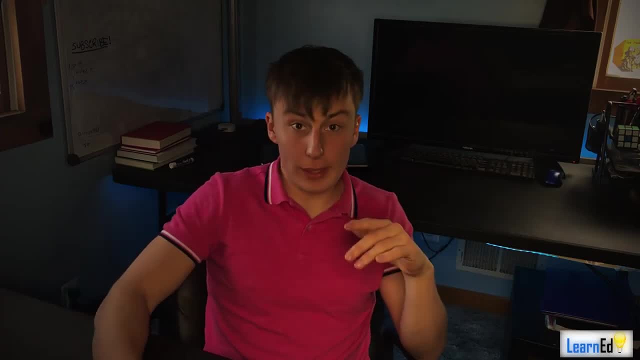 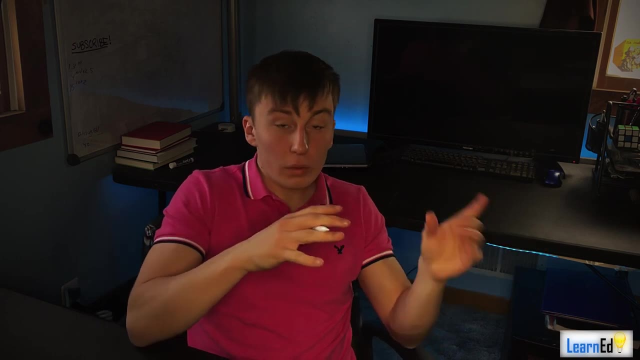 column space and we want to find a matrix a where the column space of a is this mess, okay. so we have to understand what a column space is and we have to understand what a column space is, and we have to understand what a column space actually is. right, the null space of a, okay, is the. 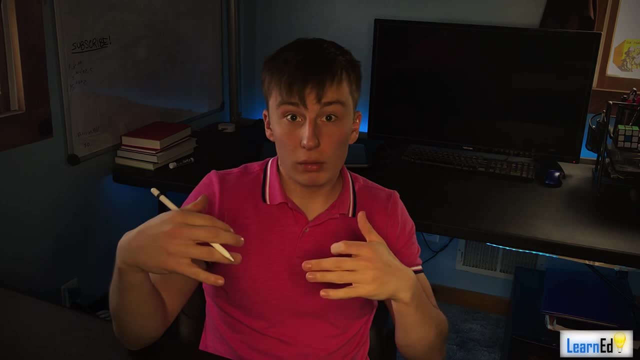 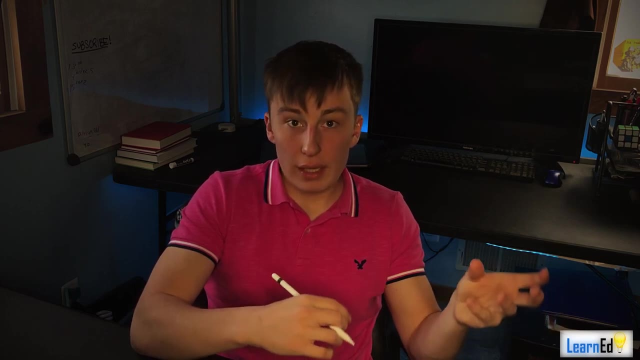 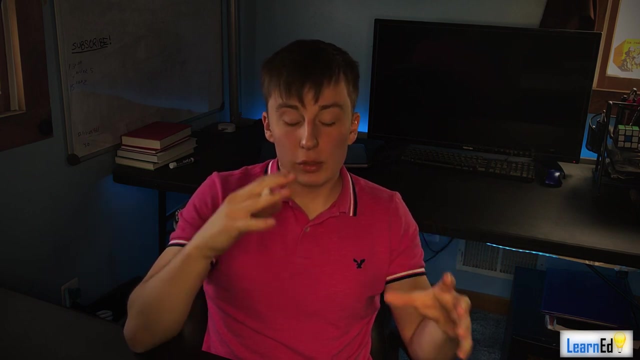 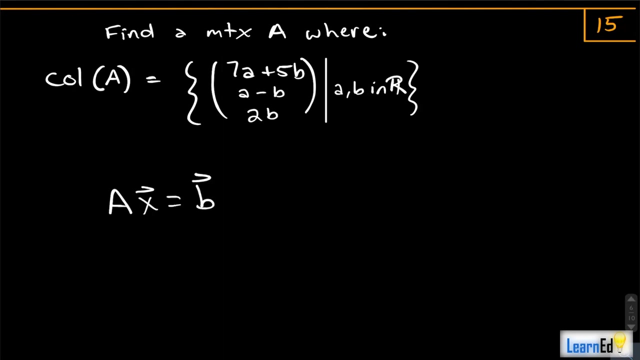 set of all vectors that go to zero when you linearly transform them with that matrix a. okay, the column space of a is all of the possible linear combinations of a. okay, so that, and to describe that right, let's say we have the matrix equation ax equals B. let's say we have an. 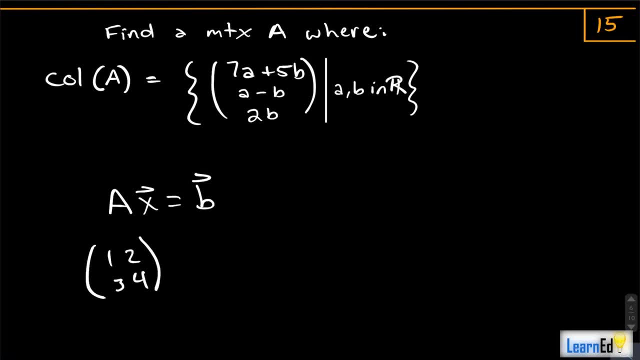 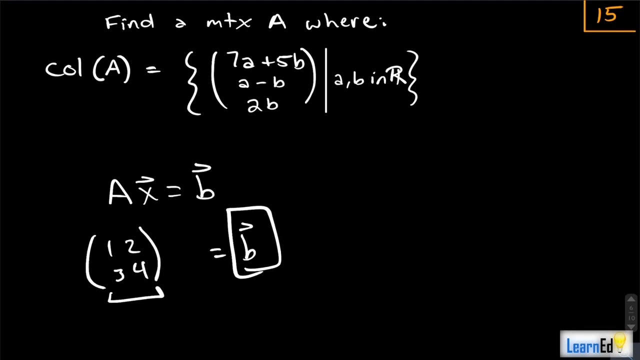 a, that's one, two, three, four, okay, the column space of a. okay is basically represented by all the possible B's that you can get here. right, because it's represented by all the possible linear combinations of a right. and well, what do? what do we mean here? why does that make sense? well, when you multiply that, 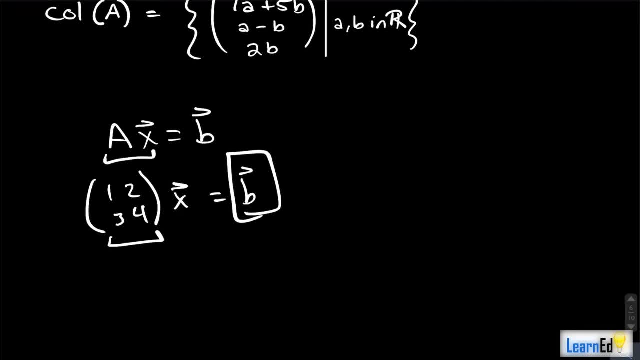 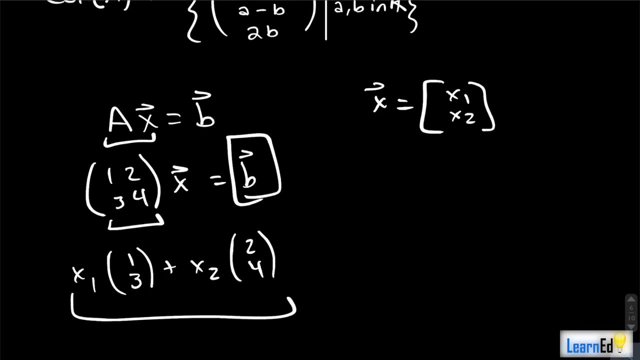 When you perform this operation, AX, you get, let's say the X is X1, X2, right. So you get X1 times 1, 3 plus X2 times 2, 4, right. This here is all of the possible linear combinations of these two vectors, right. 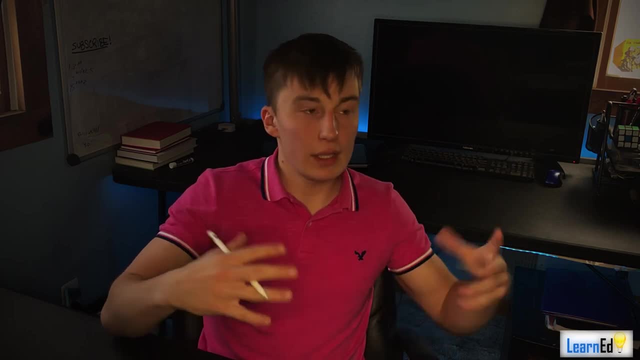 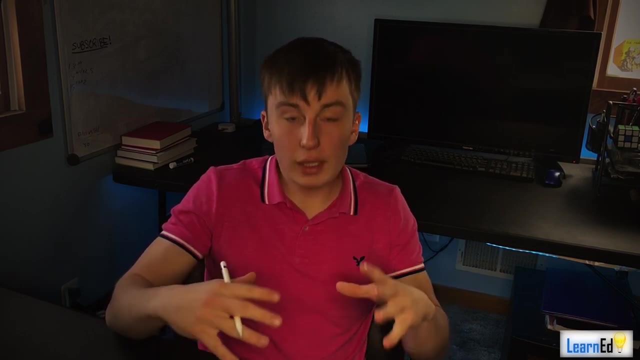 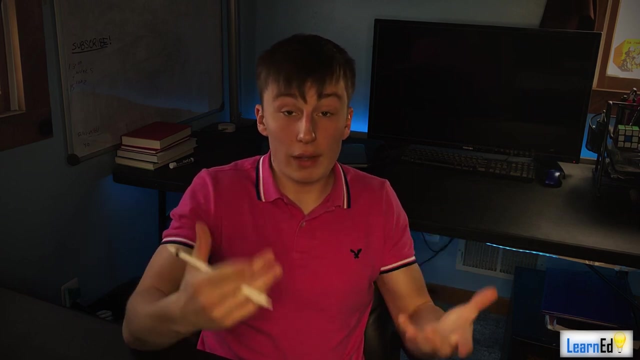 Because we can put any X in there. okay, So that gives us like infinite freedom, right, We can get all the possible linear combinations, okay. So basically, how we represent the column space is by a span of the columns of A right. 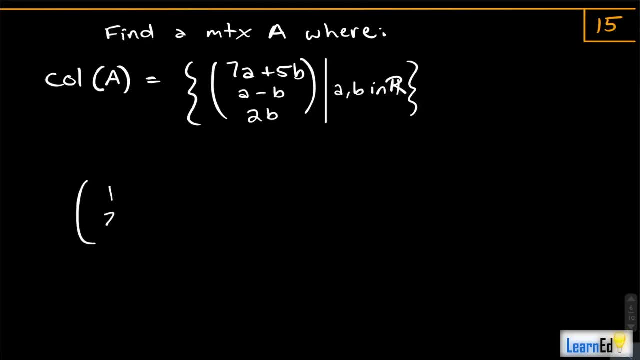 So if we have a matrix- 1,, 2,, 3,, 4,- okay- And we say that's matrix, let's get away from A. Let's say this is B. The column space of B equals the span of 1,, 2, and 3,, 4, okay. 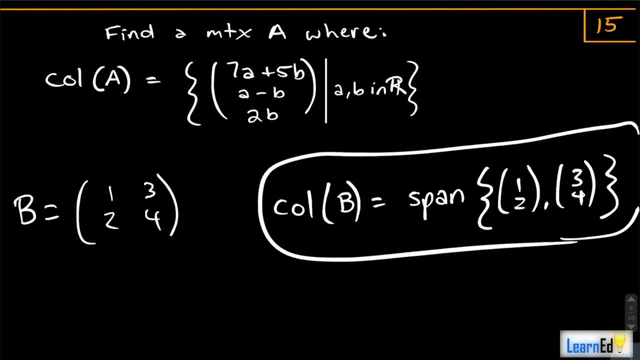 That is what we mean with column space. Okay, so it's all the possible Bs that you can get. all right. Now this, this doesn't look like. you know. we're already defining the column space. We're already saying what the column space actually is. 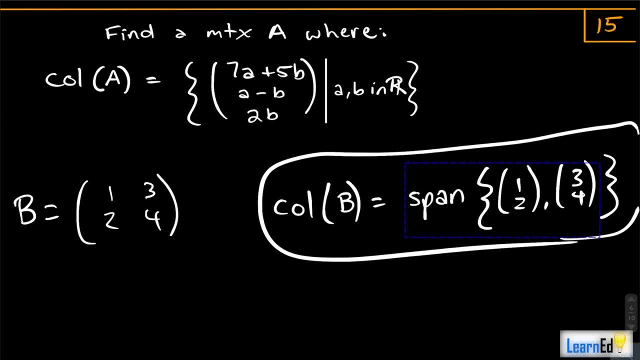 But before you've seen that I had the column space defined as a span. Well, here this is kind of like a span, worked out a little bit, Okay, and now I've got to go erase this stuff again. okay, Hang on erasing, erasing, erasing, good. 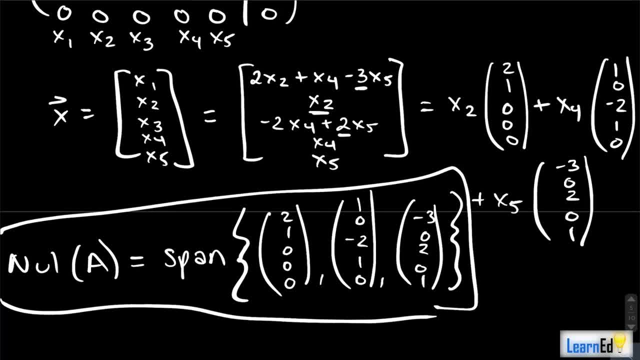 So in the last problem we had the x vector described similarly to this, okay, But then we broke it up and formed a span, right. So this is kind of like an alternate form. That's kind of how you can think about it, right? 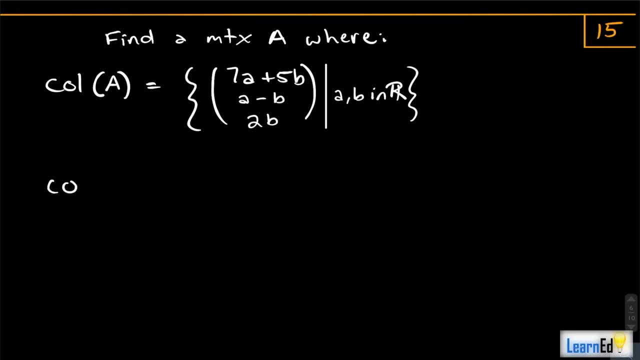 Because we can break it up and say that the column space of A equals A times 7, 1, 0, plus B times 5, negative 1, 2,. right, This is just how many times B appears in each row, okay? 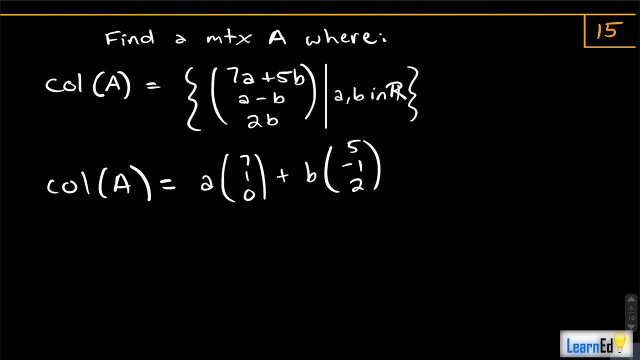 And this is how many times A appears in each row. So we can now write the column space of A as the span Of these two vectors, Right, And maybe, if that didn't make sense, why we did that in the last problem, it's because 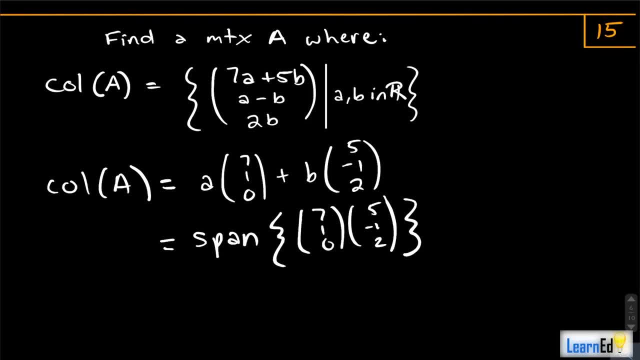 A and B here could be anything right. They could be any value. They could be 1,, 2,, 3,, 4,, 5, anything. So we can write that as a span. That's how we can illustrate and eliminate those variables. 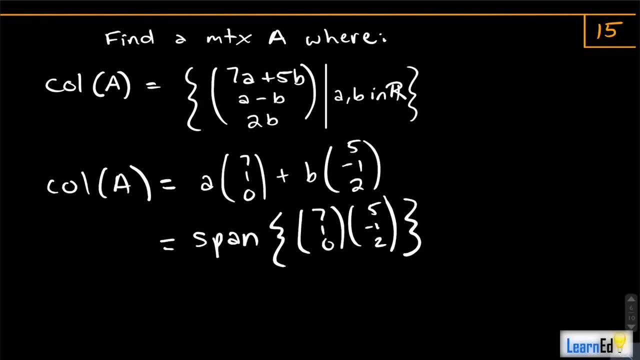 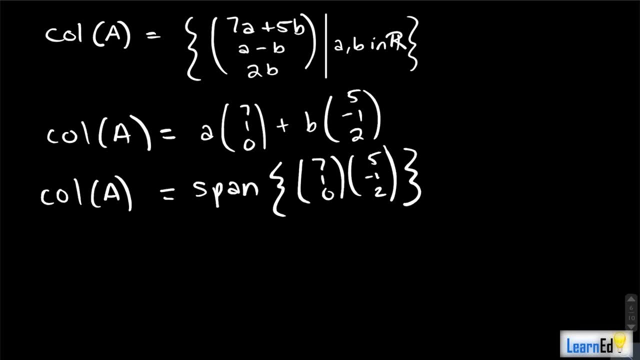 Okay, so that's why we're doing this. Hopefully that starts to make a lot more sense to you. Remember how I said that the column space of A is the span of A. It's the span of the columns of A. So if it's the span of the columns of A, if those two vectors are the columns of A, 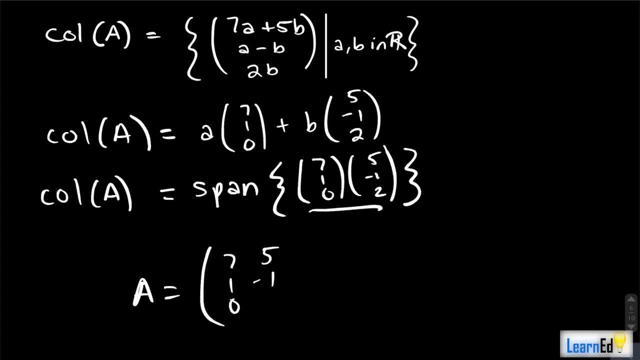 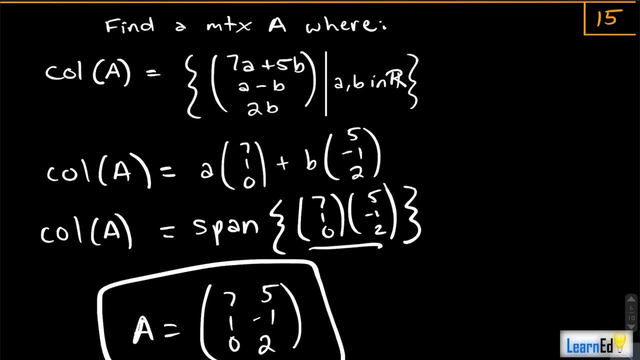 we can just now write this as 7, 1,, 0,, 5, negative, 1,, 2, and be done Right, That was the idea with this problem, So hopefully that makes a lot more sense now. 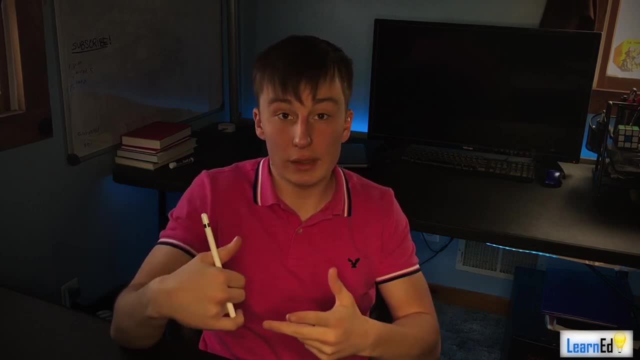 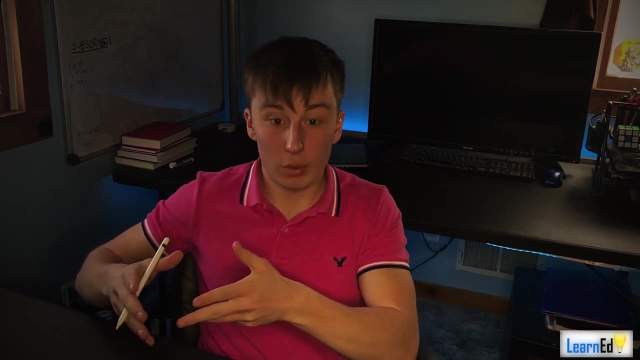 We're talking about what the column space of A actually is. right, It's the span of all the possible linear combinations of A, Giving you every single B vector that you need. Giving you every single B vector that you could get, Okay. 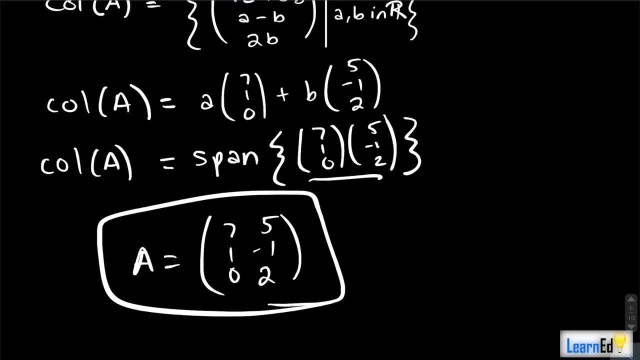 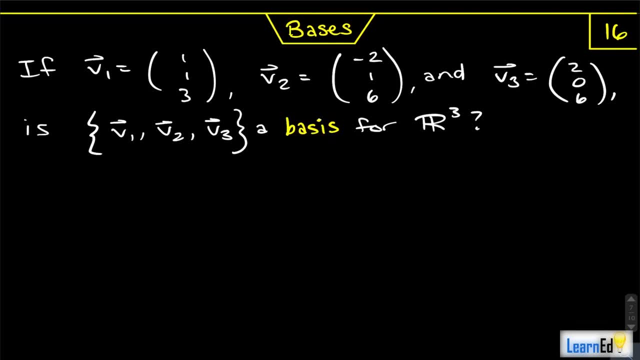 That's what this span, that's what this column space is telling you. So, moving on to problem 16, on bases, We have that if V1 is 1, 1, 3.. V2 is negative, 2, 1, 6.. 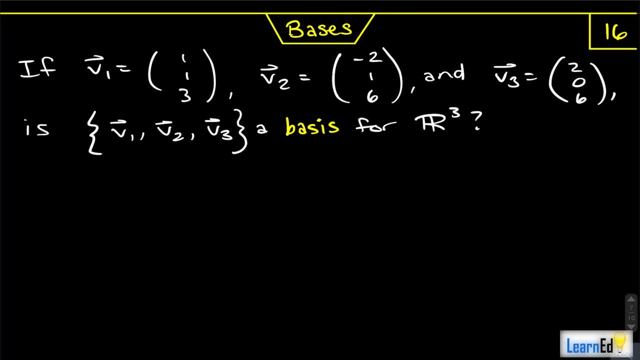 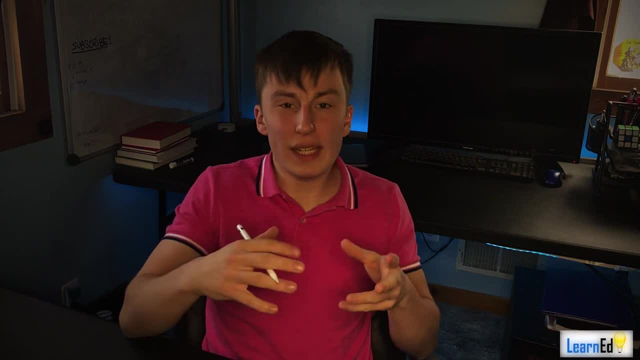 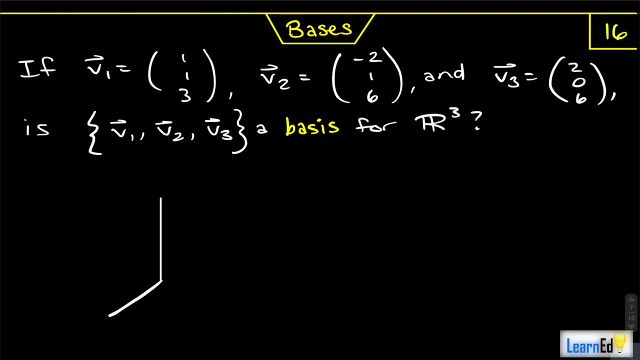 And V3 is 2, 0, 6.. Is V1, V2, V3 a basis for R3?? Okay, So first we have to talk about what is a basis Right For R3.. Well, an example of a basis for R3 is just the standard basis. 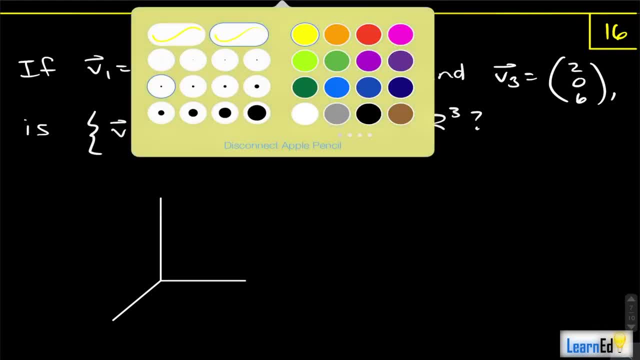 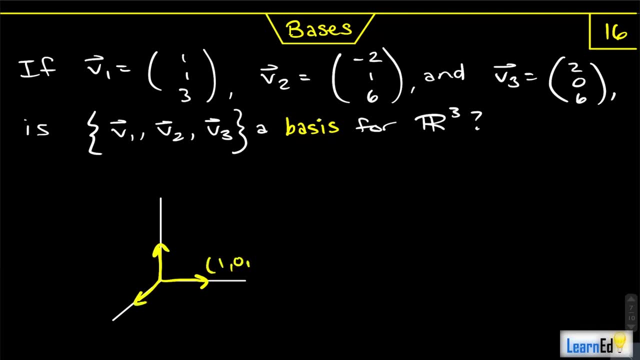 Right, We can just use that And basically let's kind of just write that out real quick here. Okay, It's the vectors We have. you know that point 1, 0, 0.. We have 0, 0, 1.. 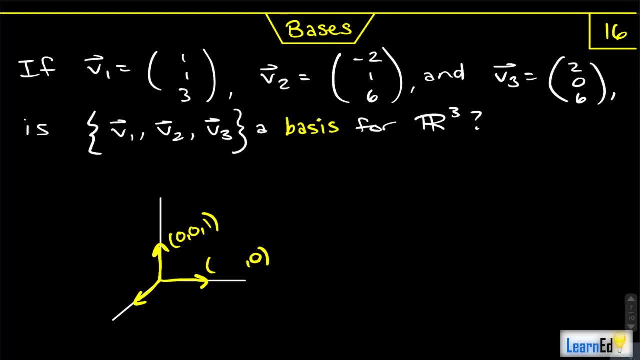 And we have, and that's actually. I usually draw that as the y-axis, So I'll do that And then say: this is 1, 0, 0.. Okay, These vectors form a basis for R3. Why? 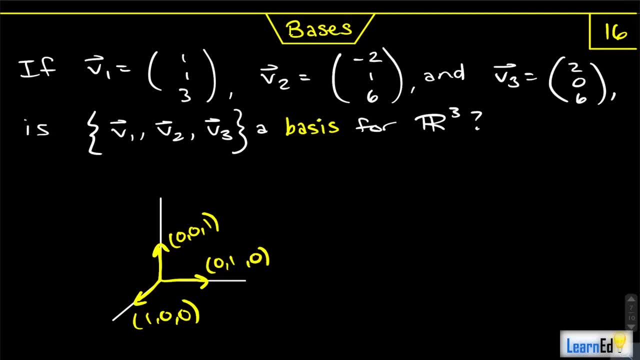 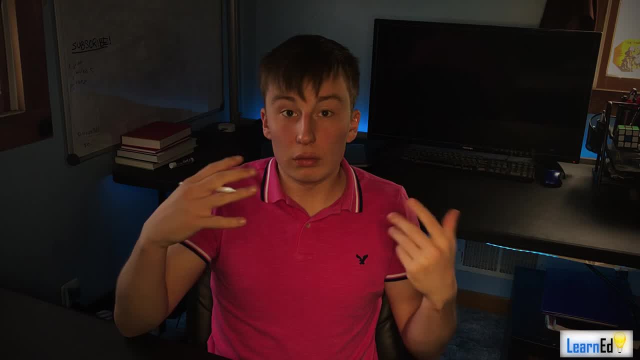 Because they span R3.. Right, You can take any linear combination, Okay, And if you take all possible linear combinations, they can describe any point on R3. Or in R3, rather Okay. So that's the idea of a basis. 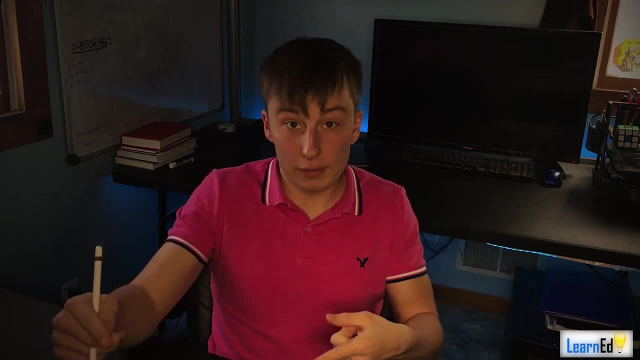 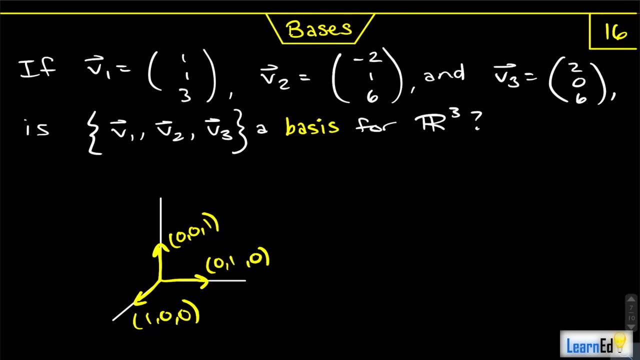 They span R3.. So they're a basis for R3.. Okay So, And basically what that means is you can use them as building blocks in a way. Okay, Maybe that's another way to think about it. So I'm just trying to give you alternative ways. 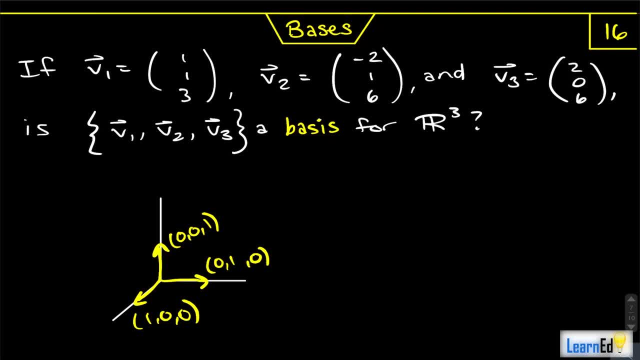 Now here's the idea: If we put those vectors into a matrix, Right? So we have 1, 0, 0. 0, 1, 0. 0, 0, 1.. They are linearly independent. 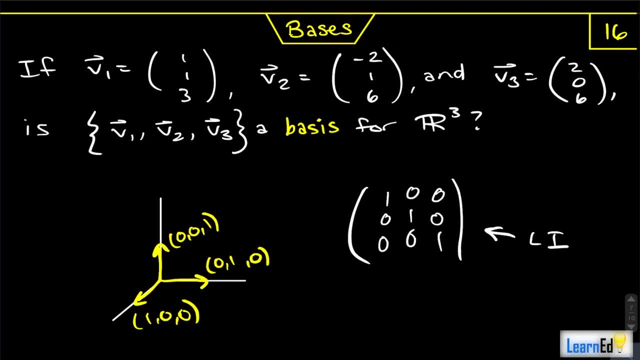 And that is characteristic of any three vectors that will be a basis for R3. They will have to be linearly independent. If they're not Right, Let's say we had 1, 0, 0.. 0, 1, 0. 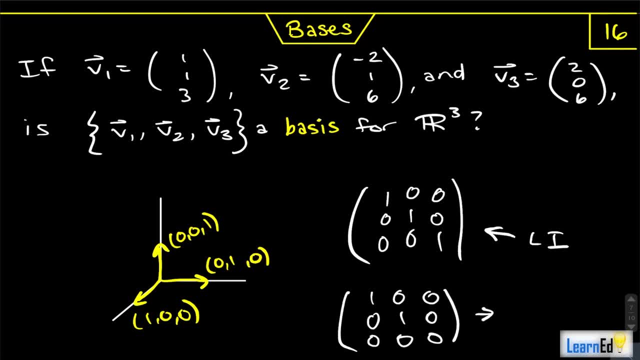 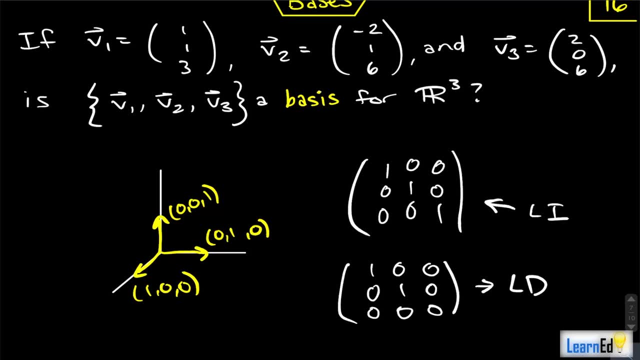 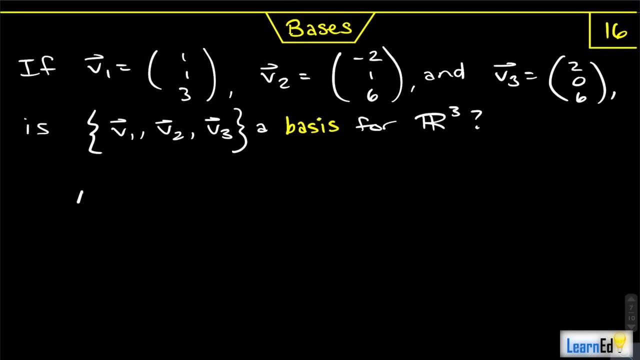 And then this column got zeroed out. Okay, This would be linearly dependent, And so it would not be a basis. Okay, So that's the idea here. So what we do? We put these three vectors: 1, 1, 3.. 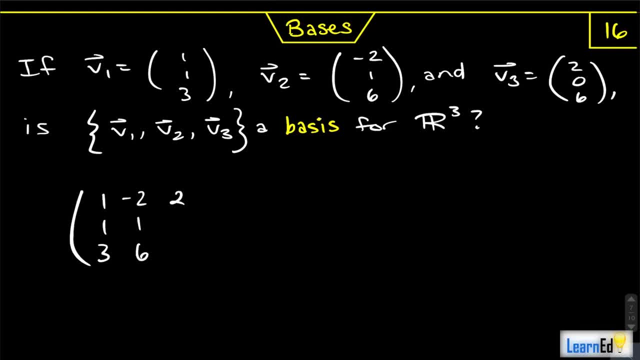 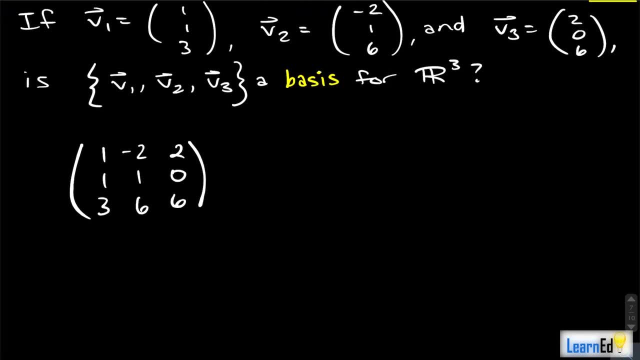 Negative: 2, 1, 6.. And 2, 0, 6.. We're going to put them in a matrix And row reduce, Okay. So first off, We can see here that it would be best to scale down the third row to 1,, 2, 2.. 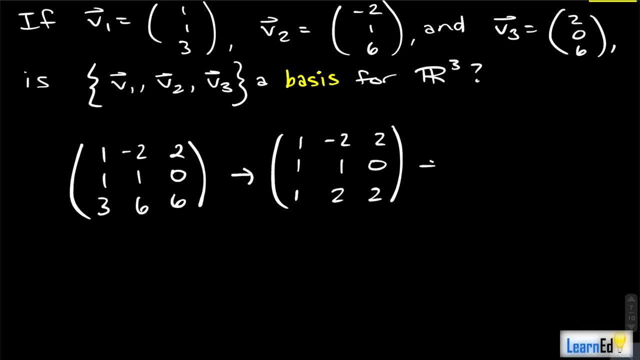 Right, We can divide by 3.. And then we can more easily row reduce by just zeroing out the pivots below, Or, sorry, The entries below the first pivot. Okay, And we'll keep the first row here To get this entry to be zero. 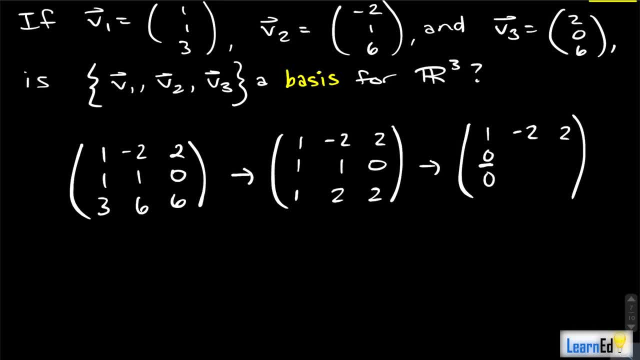 We just had to multiply by negative 1 and add, And the same thing for the third column. So multiplying negative 2 by negative 1. We get 2.. We add 1.. We get 3.. On the same token, 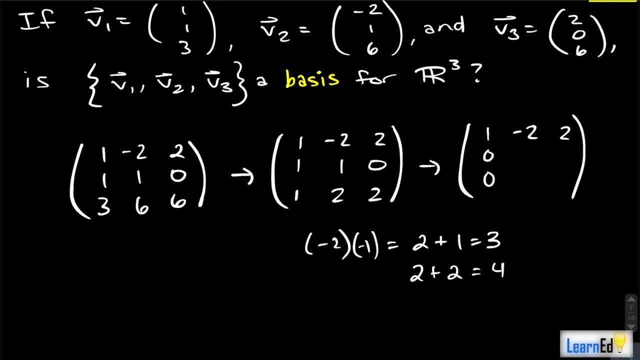 If we added 2., We would get 4.. So we know that right here it's going to be 3.. Here it's going to be a 4.. For 2 times negative 1. We get negative 2.. 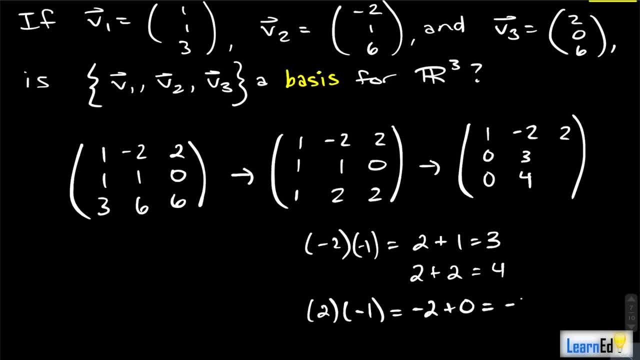 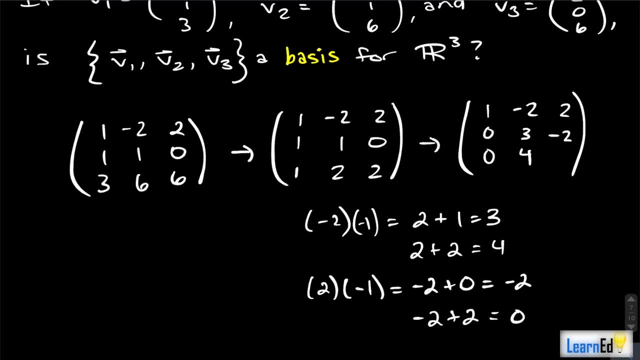 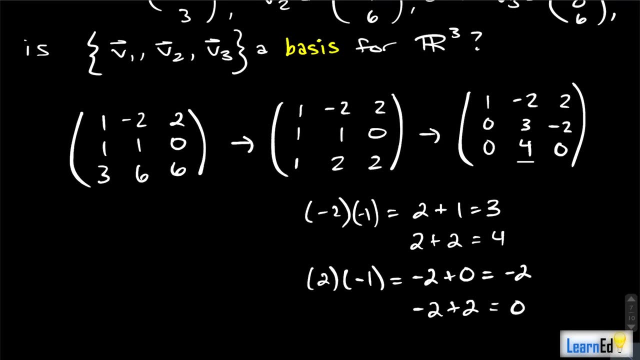 And we add 0 to get negative 2.. And if we add to this 2. Negative 2 plus 2 is 0. So we get a negative 2 and a 0.. If you zero out this entry Here, 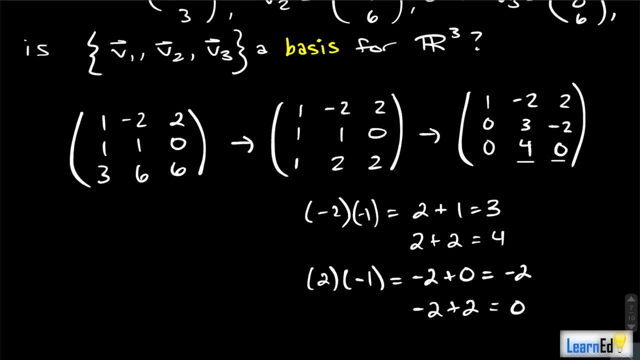 Okay, Then you'll actually get a non-zero entry here. So this isn't All. hope is not lost yet. This still could be linearly independent. Okay, I would get this to row echelon form Before you make any decisions. 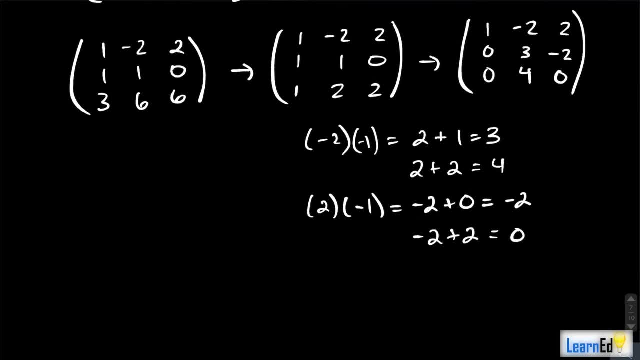 Okay, This is not yet in row echelon form, So what I'm actually going to do, And even to further prove this here, Let's prove this in another way. I can swap rows here And I'll scale down 0,, 4,, 0.. 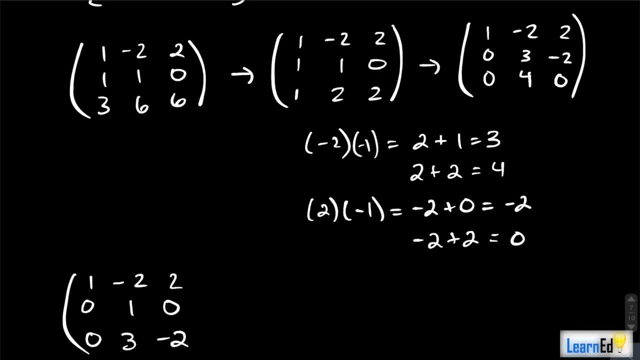 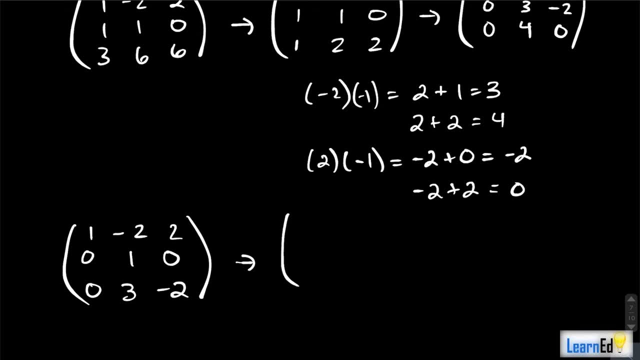 To get 0, 1, 0.. And voila, I made a row swap And I no longer have a zero entry here, So there's another way that I could have done it. Okay, So The last thing that I have to do here. 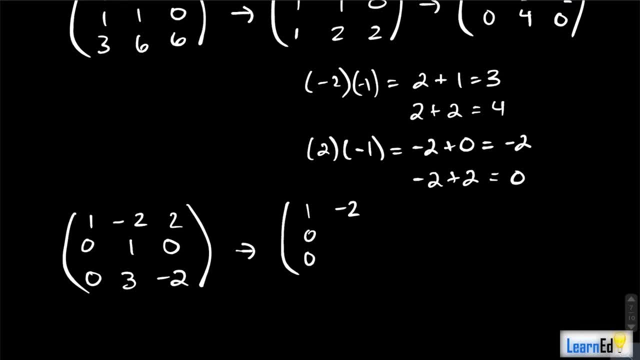 To get this into row echelon form Right, So we can see if this is linearly independent Or dependent. We can zero out this entry here. How we do it? We multiply by negative 3 and add: Okay, We multiply row 2 by negative 3.. 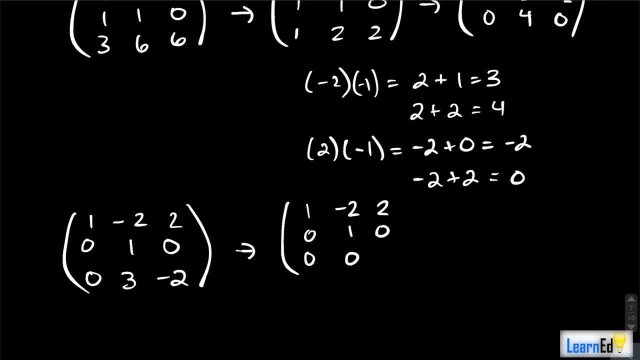 We add on to row 3. If we do that to this entry here, We would still end up getting negative 2. Because this is a zero, So it doesn't do anything, And we end up with 0, 0, 1.. 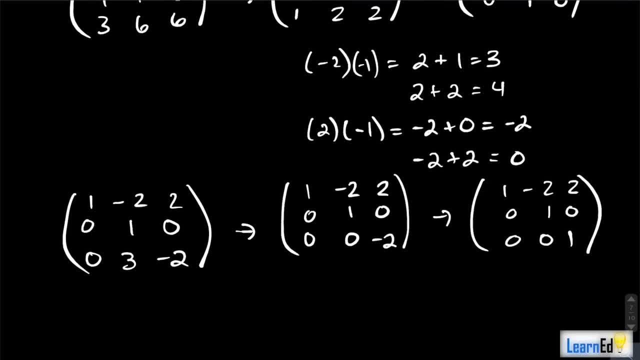 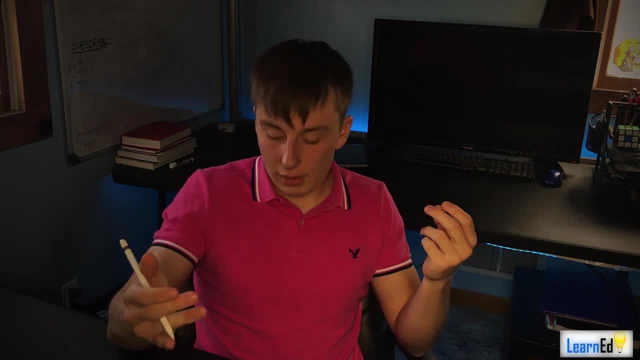 We can scale that down And we have a linearly independent matrix. Now you can put this into reduced row echelon form. It honestly doesn't matter at this point And it's kind of whatever makes you feel better. I always put these in reduced row echelon form. 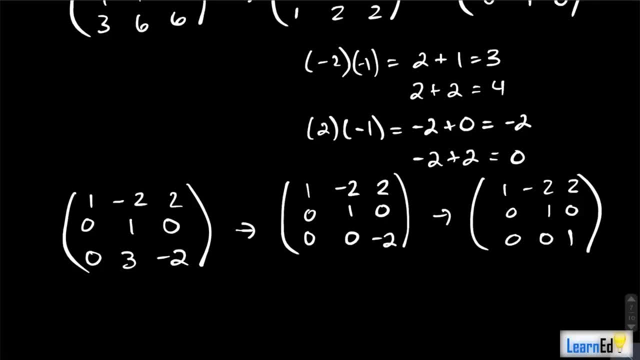 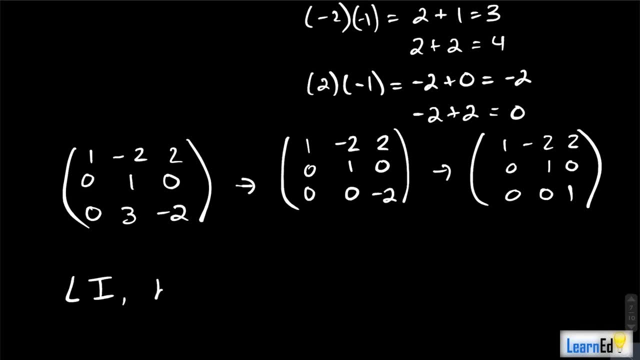 Because it just made me feel a little more comfortable, Right, But from this you can literally just say this is linearly independent. Therefore, you can say that V1,, V2, V3 is a basis for R3. Okay, 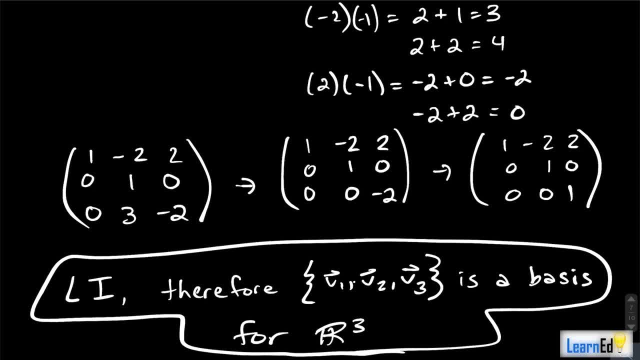 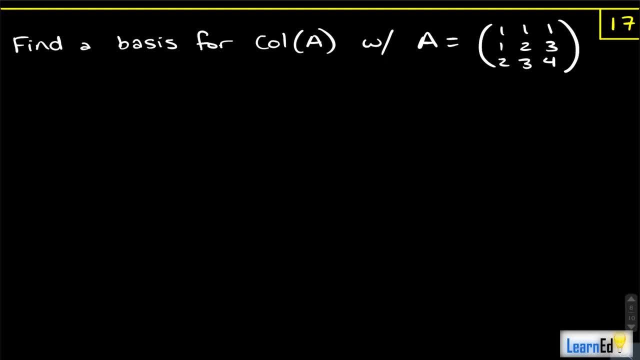 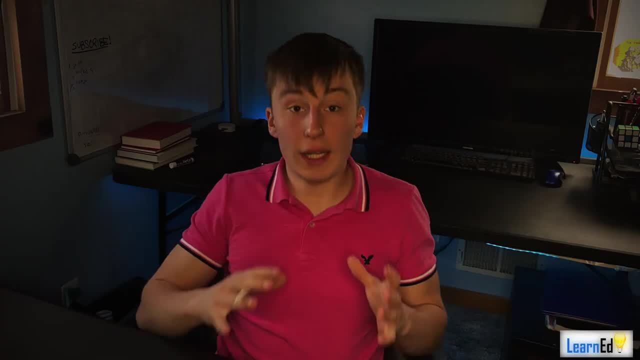 And that does it for problem 16.. So, moving on to our next basis problem here, Number 17 is asking us to find a basis for the column space of A, With A being a 3 by 3 matrix. Okay, So we now want to find a basis for the column space. 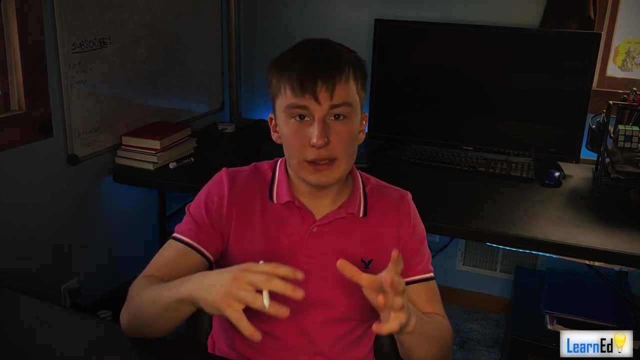 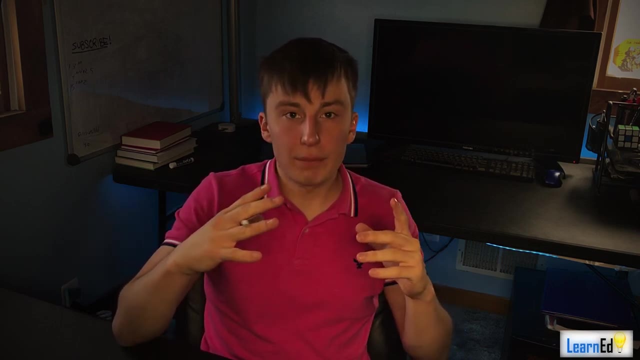 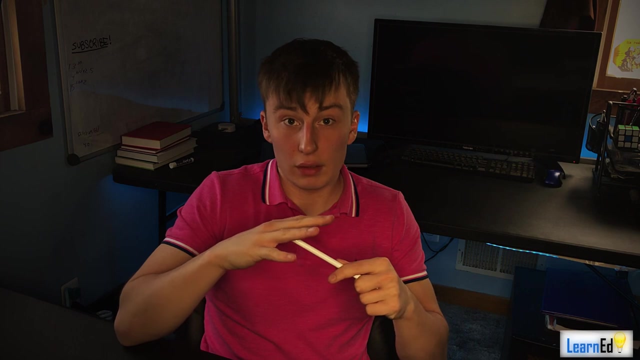 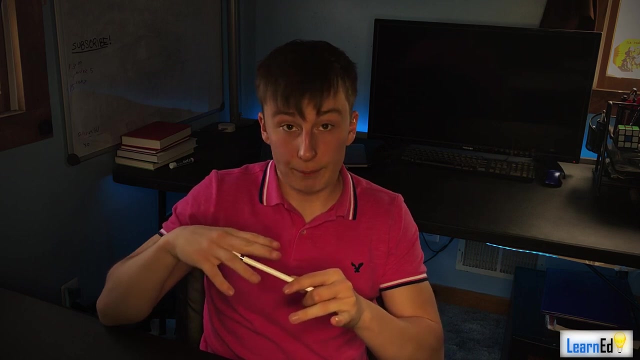 Okay. So basically what this means is that maybe one of these vectors, Okay In A one of these column vectors- are useless. Right, Remember what the column space of A actually is. Okay, The column space of A is all the possible linear combinations of the columns of A. 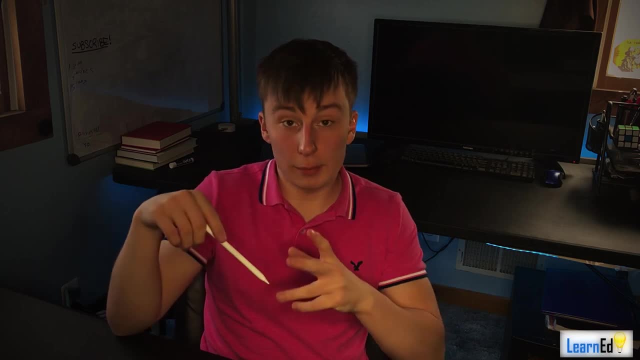 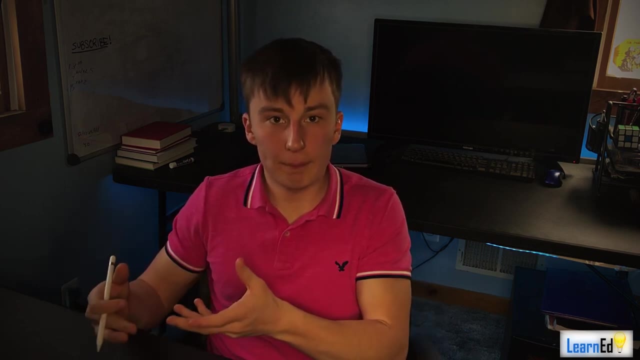 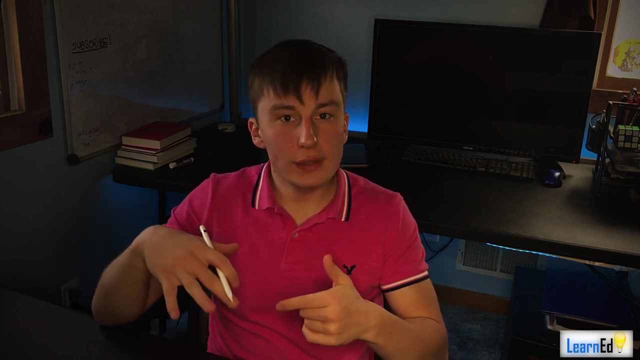 Right, All the possible linear combinations of the columns of A. So it's basically all the possible values of B of the vector B Right And the matrix equation AX equals B, So maybe we can still describe the column space of A without using one of these vectors. 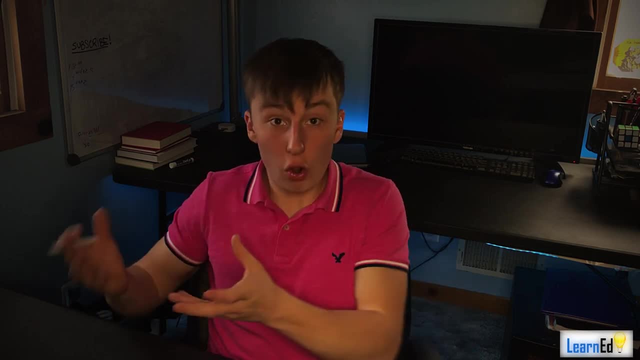 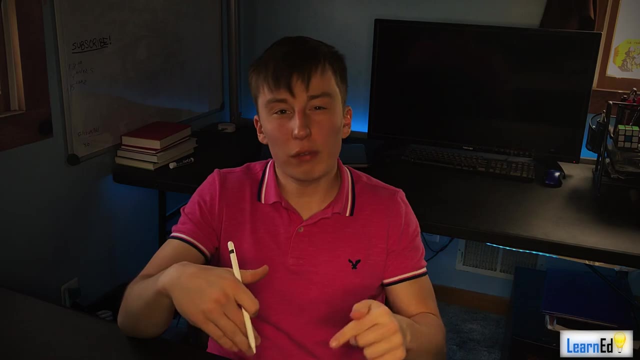 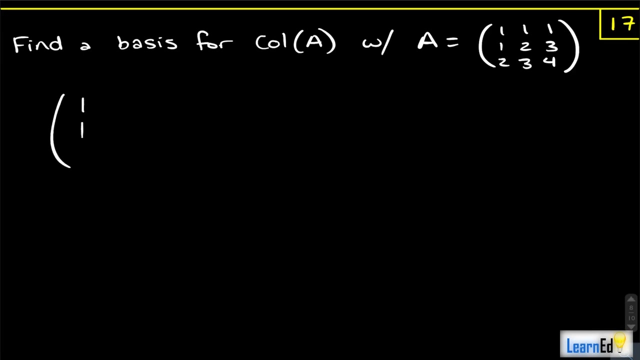 Right, Because maybe we can still attain all of these possible B vectors with just two of these column vectors of A. That's what we're finding here, So all we have to do is row, reduce this And see: well, is this linearly dependent? 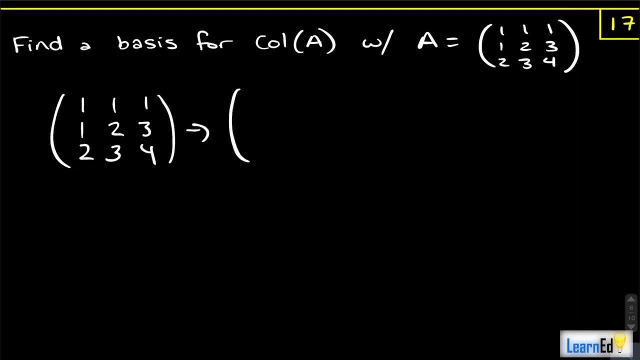 Right. So basically the same exact process as the last problem. So we zero out the entries under the first pivot And we do that first by: we multiply the first column by negative one and add. Okay, So we multiply the first row by negative one and add. 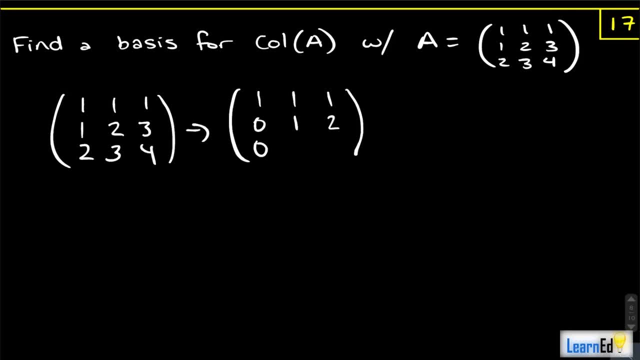 And so we get a one and a two here, Okay. And then we multiply the first row by negative two and add to get the third row- Okay, And that will zero out the third row, And so you have something that's linearly dependent. 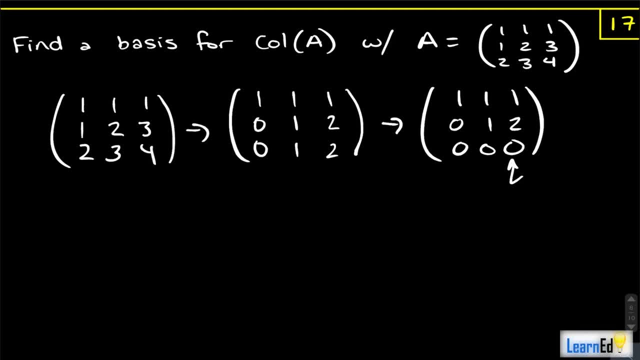 So what you can do is you can take this and see. you can see that this vector is garbage, Right, Because it's linearly dependent, Right, So you could say garbage Okay And throw it out, It doesn't matter anymore. 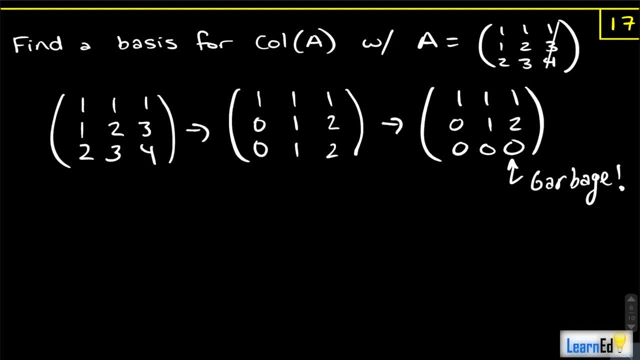 So we can just cross this vector out And we can describe, we can say that the basis for column A, column space of A, is equal to, and we'll just have one, one, two and one, two, three. 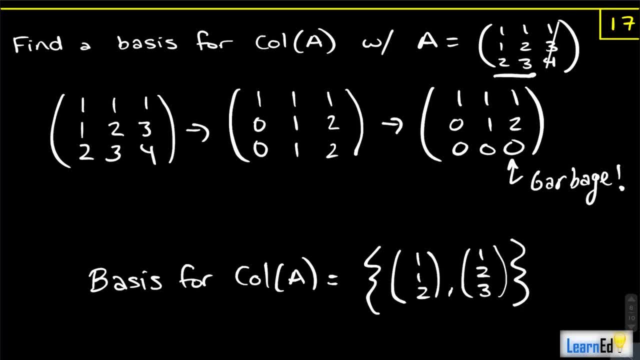 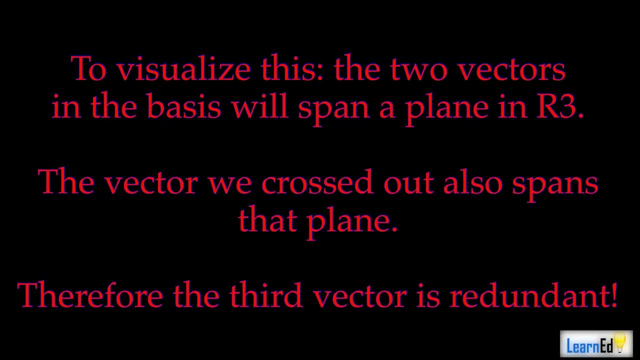 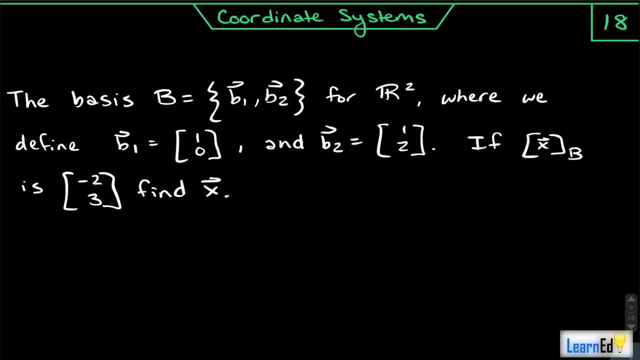 Okay, And those are the original vectors, Right? So what we did here was we just found that the third vector here was useless. Okay, So this is the answer to problem 17.. All right, So let's move on to problem 18, which is on coordinate systems. 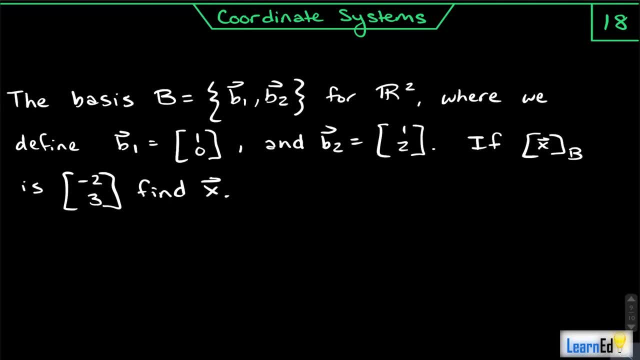 And we're given that the basis B is B1, B2 for R squared, where we define B1 as one zero and B2 as one, two, And it's asking if the coordinate vector relative to B is negative, two, three. 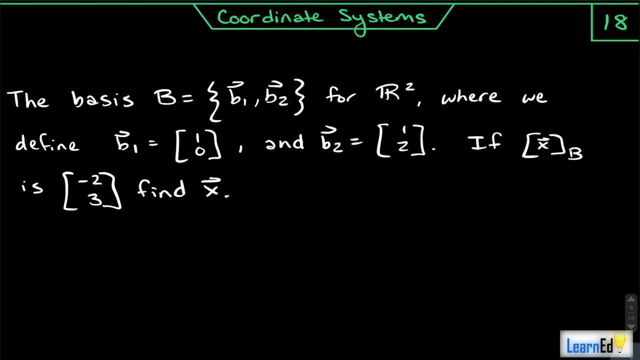 It wants us to find X, Okay. So what I think really would have helped me when I was in linear algebra was knowing that whenever we were given a basis- and this is something I don't think I fully understood- We're given a basis without anything here. 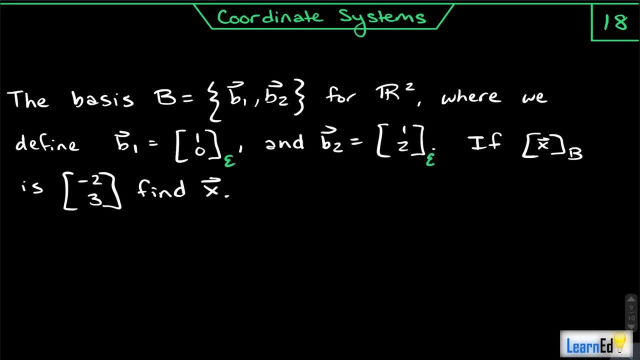 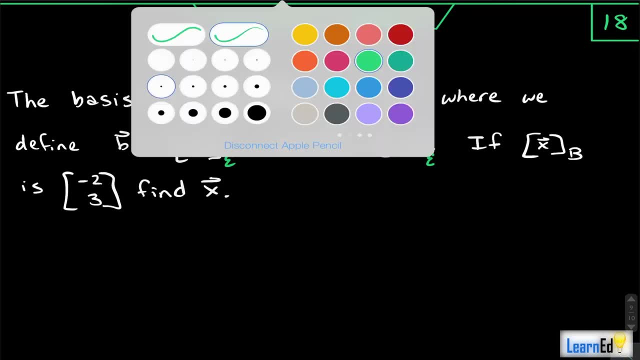 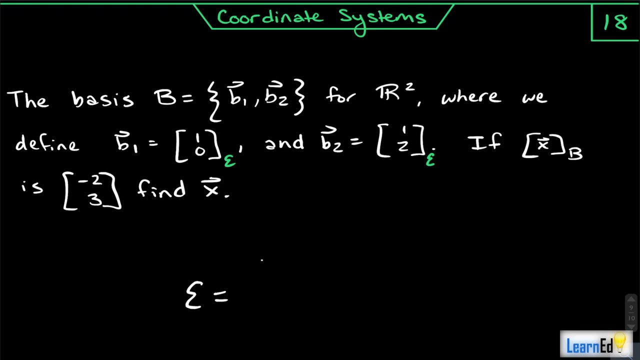 Okay, This is relative to E. So this is basically saying: okay, here's what B1 and B2 are relative to your standard basis. Right, This is what this E means. Now, what is the standard basis? Well, the standard basis for R2 is one, zero, zero one. 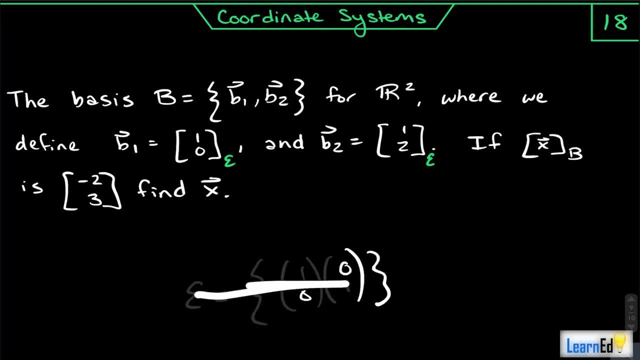 Right, It's our regular standard basis, Right? So our regular graph paper has the standard basis Okay, And it's saying: if X of B is negative, two, three, then what's X relative to E? Right To the standard basis. 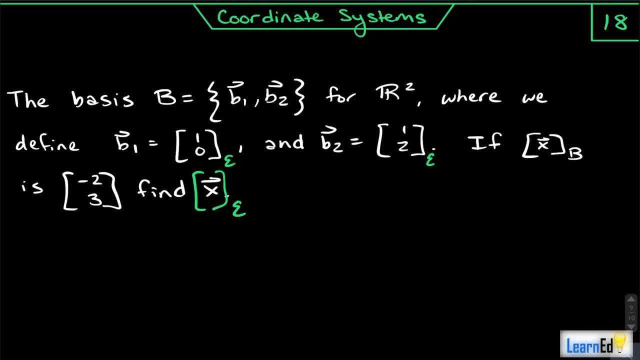 That's what we're trying to find here, Okay, So that's how you need to image this. It gives us what X relative to B is. We need to find X relative to E, Okay, So that, I think, would make the problem a lot easier to look at. 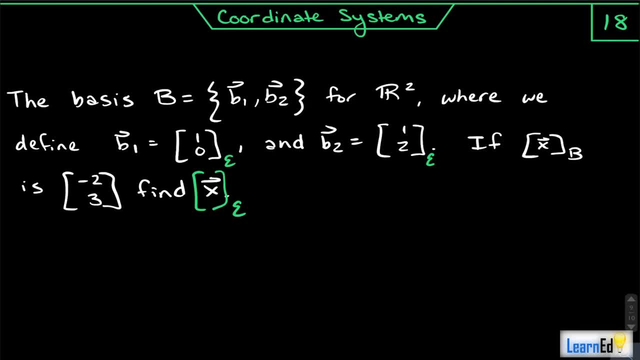 All right, But it's kind of just implied that when you don't have anything there, it's relative to E. Now be careful that that doesn't apply for this here, because you can see, here context matters, because it's saying, if X relative to B, is this: 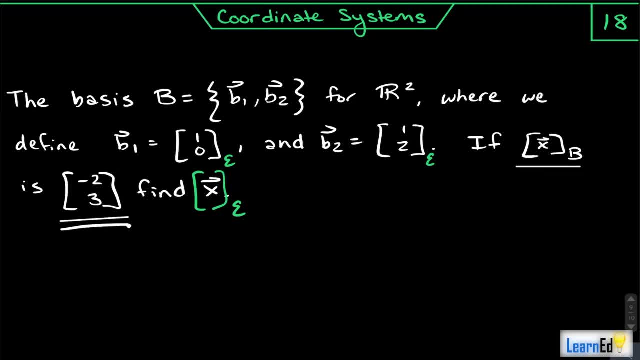 So this is relative to B Right. So this is moving negative two in the B1 direction and three in the B2 direction. So that's what this means. It's not relative to E, or else we'd already have our answer. 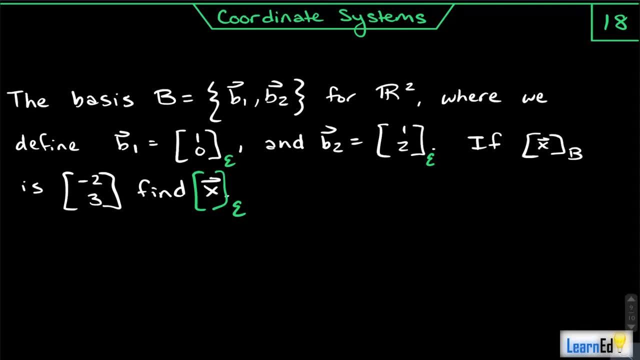 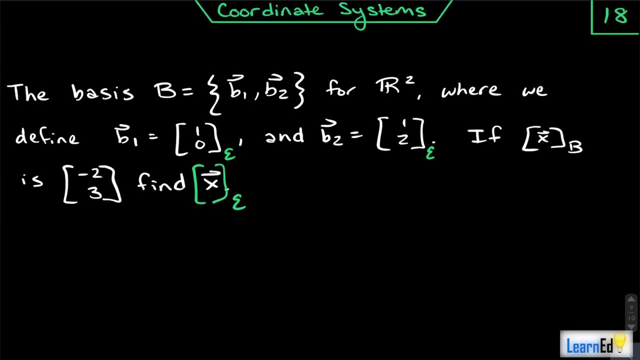 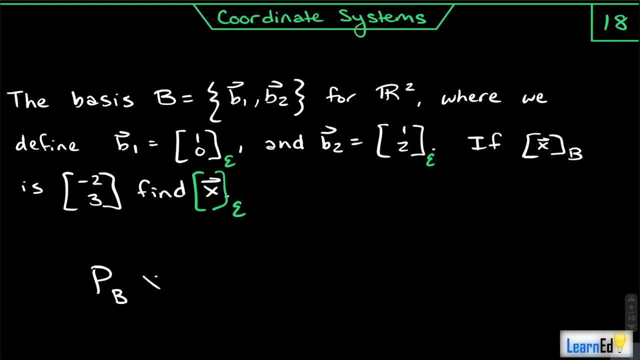 Right, Because this is what we're trying to find- is X relative to E. Okay, So actually going into this here, how do we encounter a problem like this? Well, what we do is we have this formula. We have this formula: PB times X relative to B equals X. 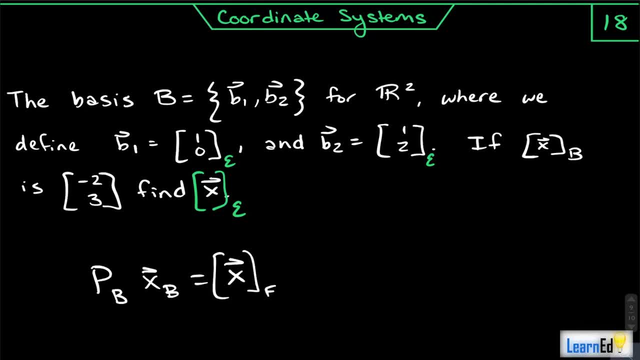 And again, this is relative to E, Right Or well. they usually write it within like an epsilon looking thing. Okay, So that's the formula that you need to be using here, But I need you to understand where this comes from, because you're going to have a lot of 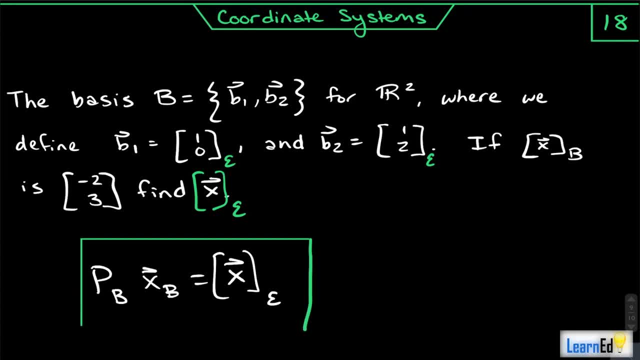 things to remember for this test. Okay, So it's not going to help you at all for me to just say: okay, here's the formula, Now go use it. The idea here is that this change of coordinates matrix PB a better way of writing this, and. 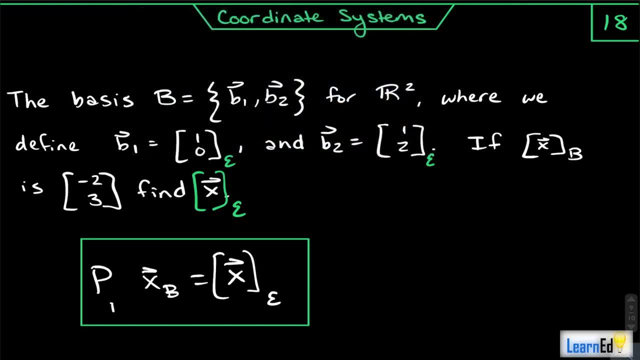 I will write it in the change of basis section- is it's going to transform a vector with a relative to B to a vector relative to the standard basis. That's its job And basically the intuition behind that is that you were given this formula. 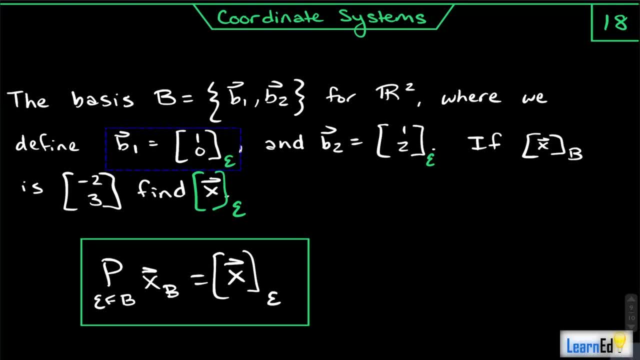 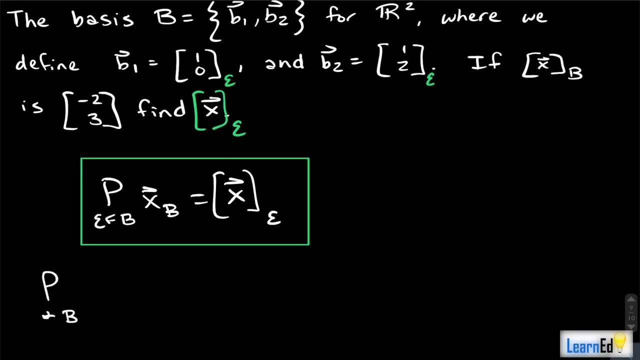 Now, how we're able to do that here is that we were given our B1 and B2 vectors relative to E, Right? So if we put this thing in a matrix, right, So let's say P going from B to E, And yeah, that's just how the arrow is. 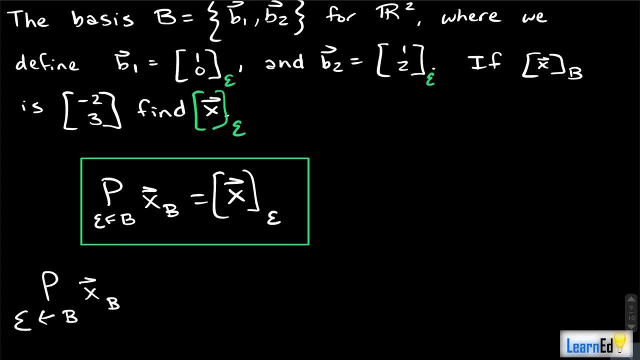 It's kind of weird, Right, I know We say that this is equal to. The matrix becomes 1, 0, 1, 2.. Okay, Now you have two vectors that will take something relative to B and convert it to something. 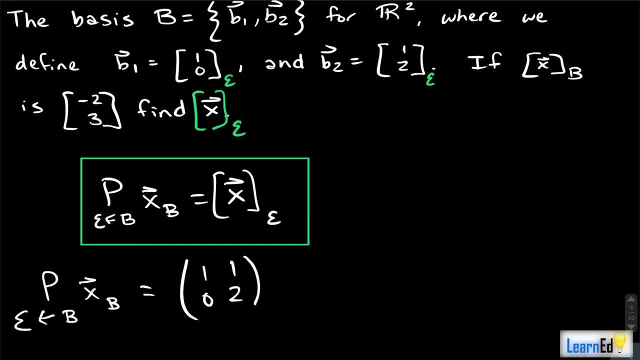 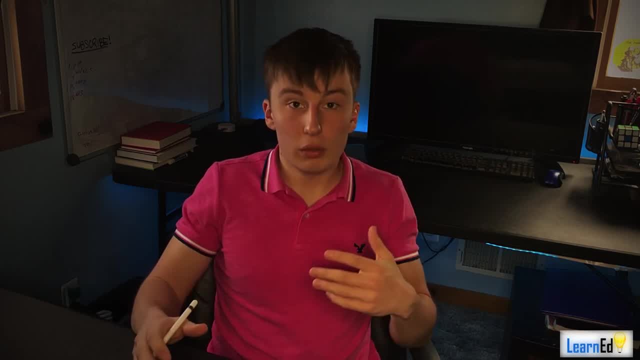 relative to E. Okay, So that's why these are so nice. If you had your two standard basis vectors being described as B1 and B2. Right, Or as relative to your basis B, then it would be flipped Right. 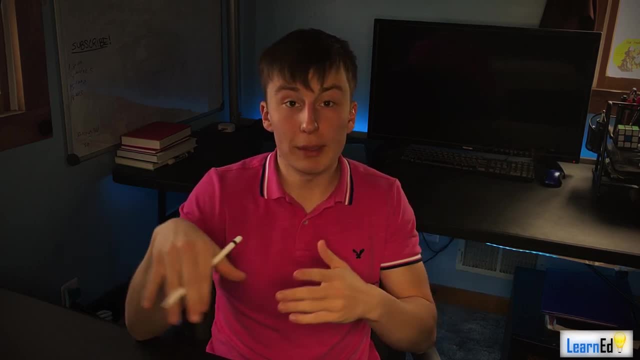 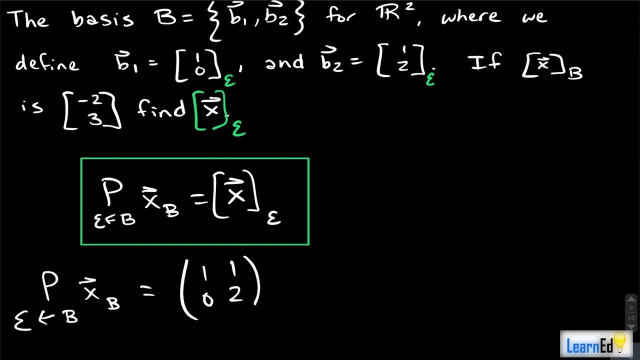 Then it would be the change of coordinates matrix from the, From the standard basis, to basis B. Okay, So, anyways, we're going to multiply this by XB, which we know to be negative, 2, 3.. And that's how we're going to get X relative to E. So we get negative 2 times 1, 0 plus. 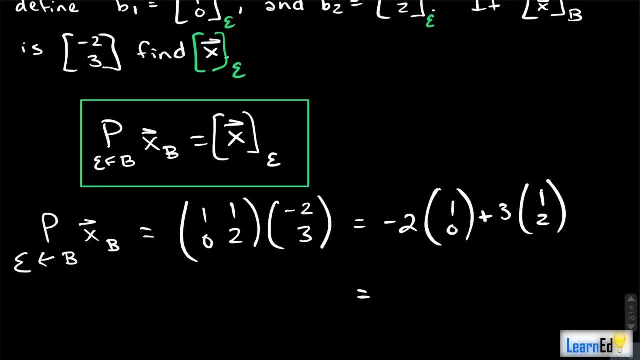 a 3 times 1, 2.. Okay, We know that that is negative 2, 0 plus 3 times 6,, which gives us a 1, 6.. And that right there, Right, there is X relative to E. Okay. 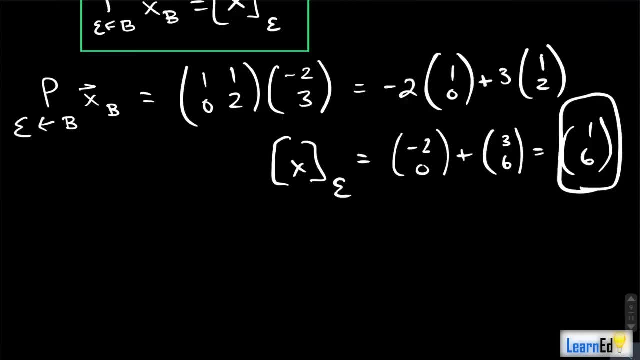 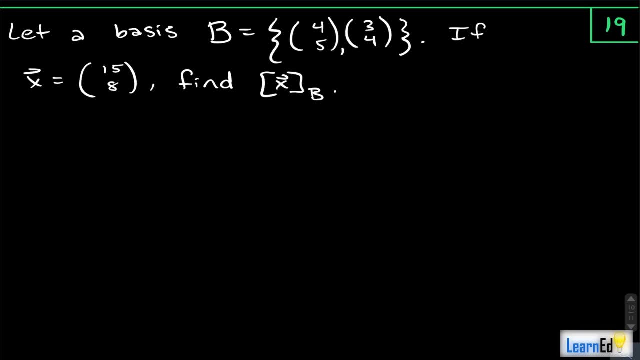 So that's how you do something like that. So moving on to problem 19.. This problem says: let a basis B equal 4,, 5,, 3,, 4.. If X equals 15,, 8, then we want to find the coordinate vector of X relative to B. 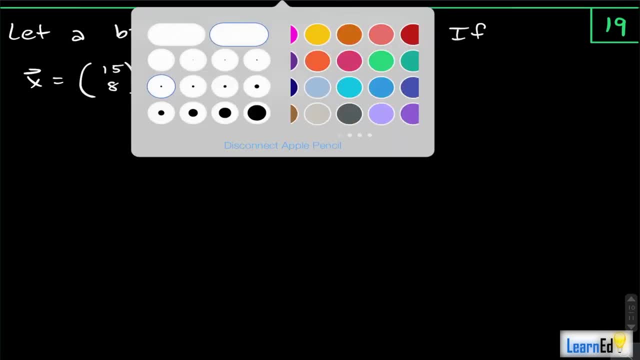 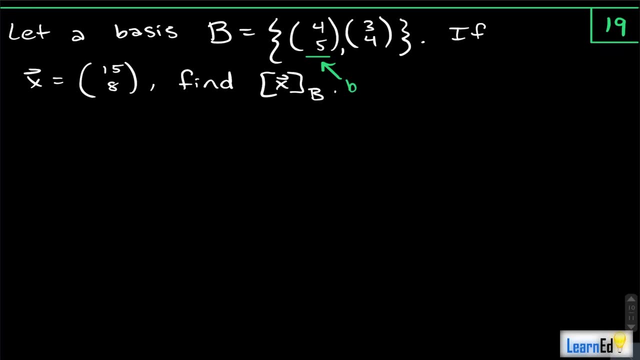 This is actually the exact same problem as we previously had, except for you know well, actually. let's start with the similarities first. This is still B1. And this is B2. And both of these vectors are relative to E again. 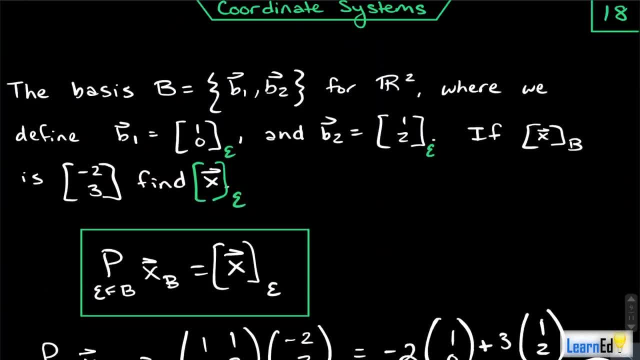 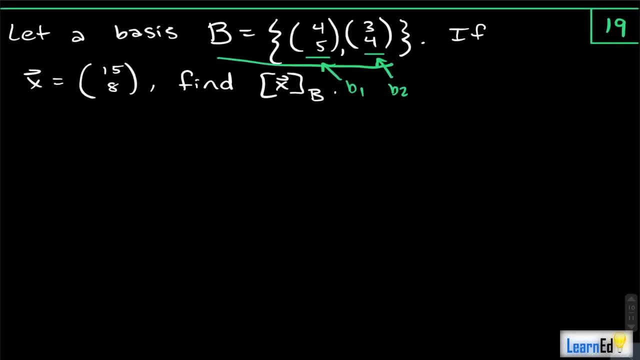 Right, They're relative to the standard basis. You can write it just as we wrote it in the last problem: Right, If these are relative to E, you write it like. you write the whole basis like this: Okay, And we're given. now we're given X relative to E, And that's the difference here. 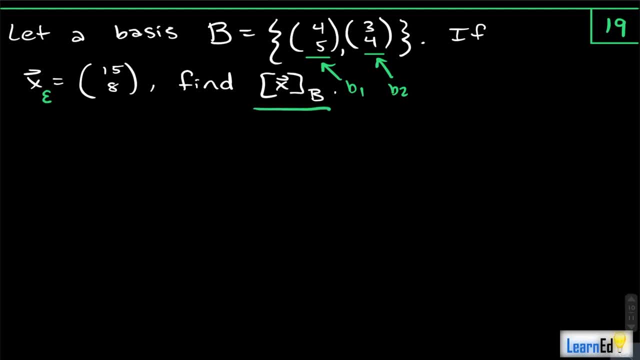 We're given X relative to E, We need to find X relative to B. So, writing out our formula, here We have P from B to E. Right, That's how we can write our change of coordinates matrix. And we multiply that by some, we have some, some vector, some coordinate vector. 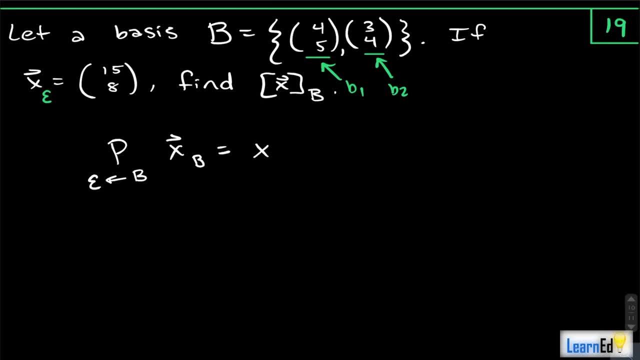 God, Some coordinate vector relative to B And that's equal to some coordinate vector relative to E. Okay, What we can do here to you know, make this a little nicer. First off, we could actually just augment this change of coordinates matrix with XE. 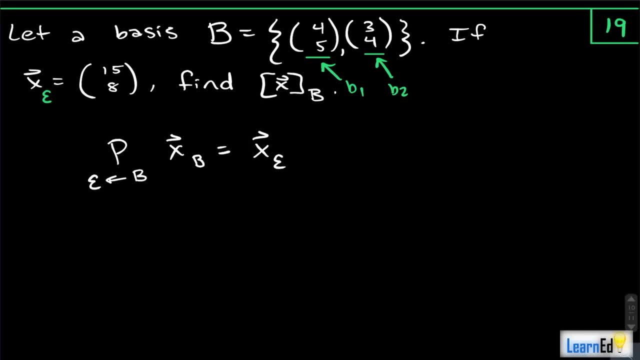 Right And then solve for XB. that way We could absolutely do that Right, But how we can also also do it and I'll show you this way: If we multiply this by P to the B to the E- inverse: 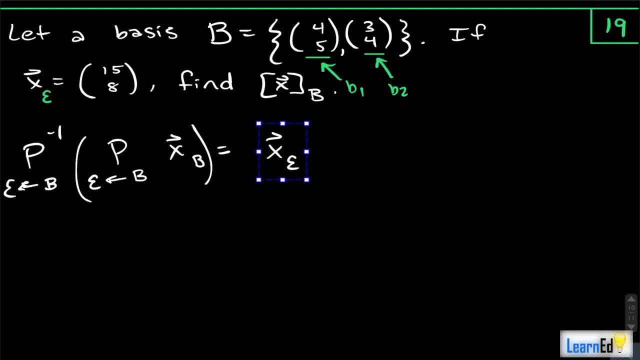 Okay, And we multiply this side by the same exact thing, We can come up with another equation Which will actually make a lot of sense, And I'll show you why. Okay, And this actually leads into the change of basis stuff a little bit. 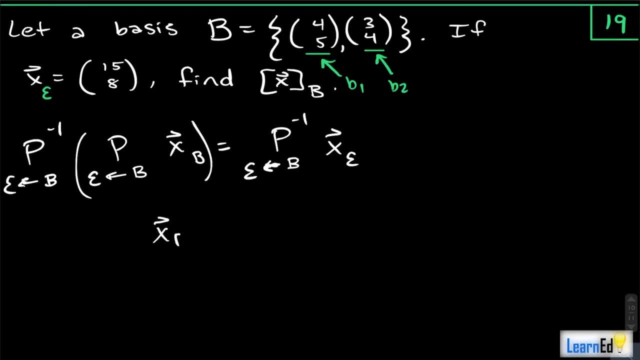 So I'm kind of working ahead, But you'll see here that this is XB Right, Because this becomes the identity And this is equal to the P inverse of BE times, XE. Okay, Now here's what's interesting. 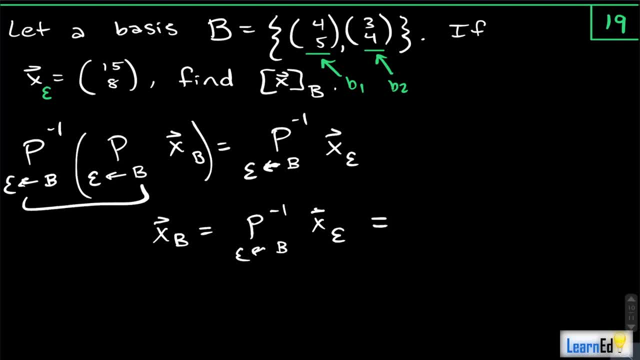 And here's what we'll talk about in change of basis, Which what I'll mention. Okay, This thing, And it makes sense to actually write it as P from E to B Rather than P inverse from P to E. Right, 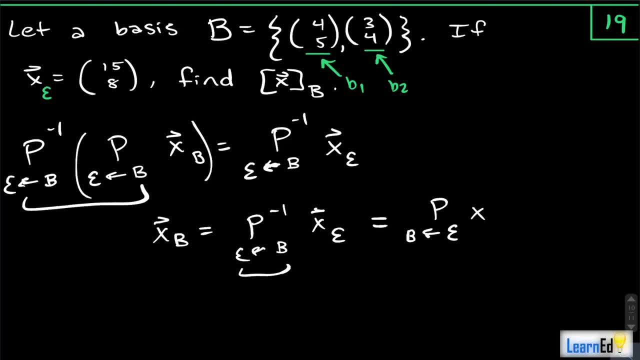 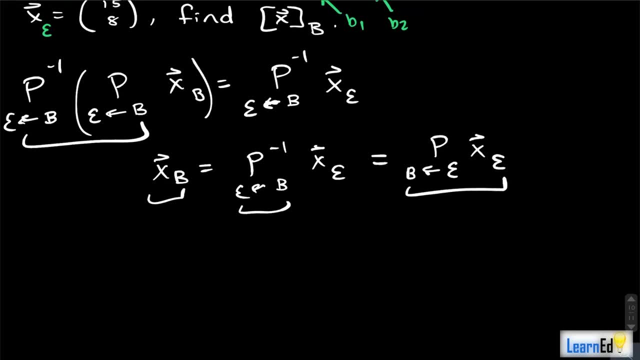 They're the same thing, But if we write it like this, Well, this is the exact same equation. This is kind of arbitrary, As you know, as the equation that we had before Of PB to E, XB equals XE. 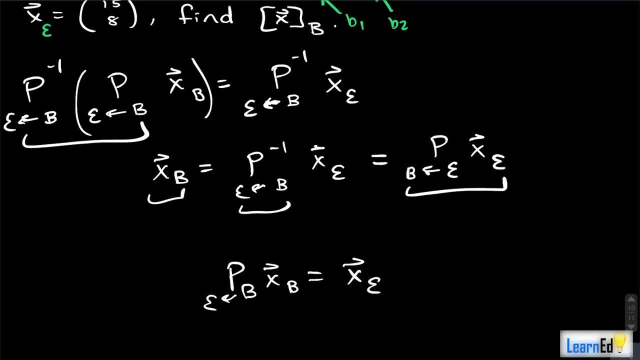 If you just flip around the E's and the B's here, You get this exact equation With these two things. Okay, So it's actually a nicer way of writing it, But so you end up getting that if you invert the change of coordinate matrix from B to E. 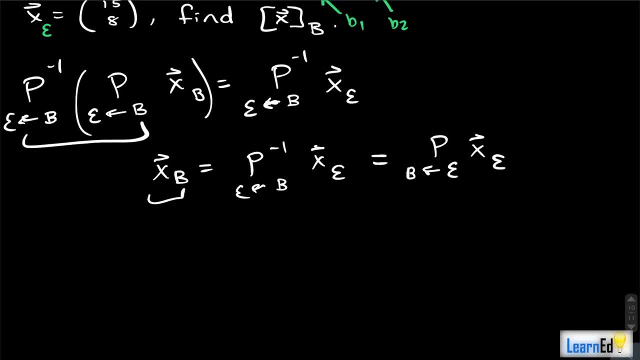 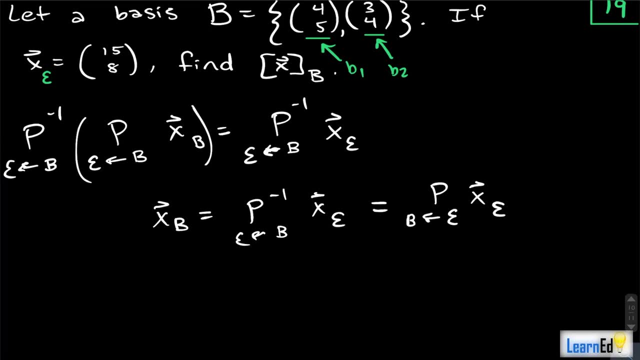 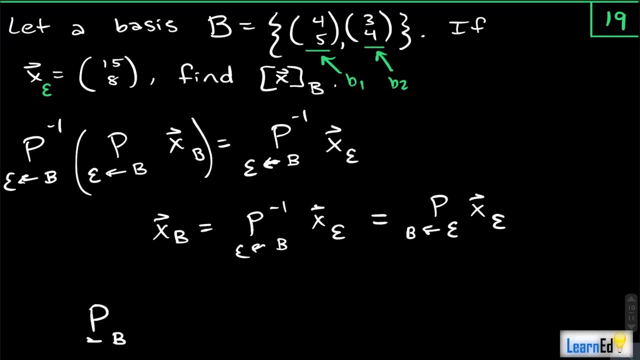 You get the change of coordinate matrix from E to B, And that's the idea from this. Sorry if that was a little disorganized, I got a little too excited, I think So. anyways, P from B to E equals 4534.. 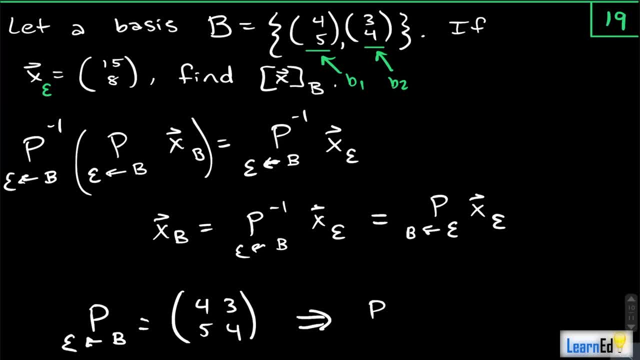 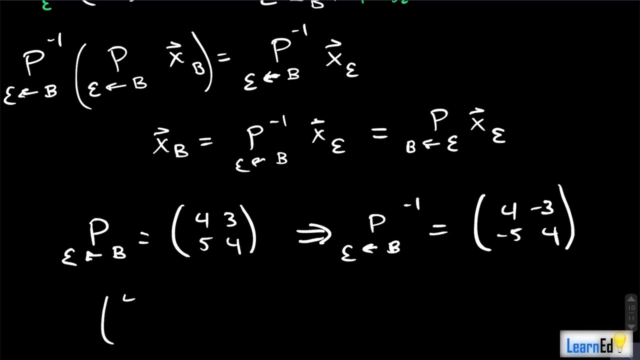 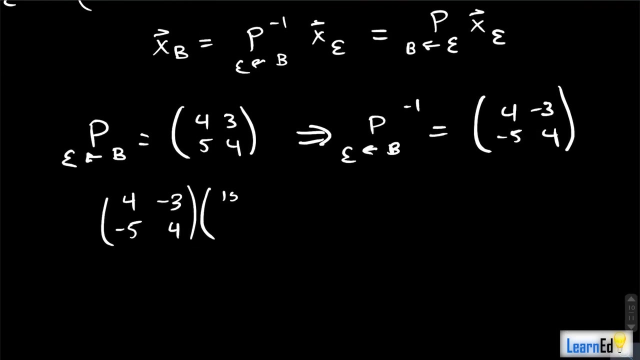 So PB to the E inverse equals, We still have those fours And we just negate the kind of reverse diagonal. Okay, And so now we have that matrix, We can multiply it By XE, Which we know to be 158.. 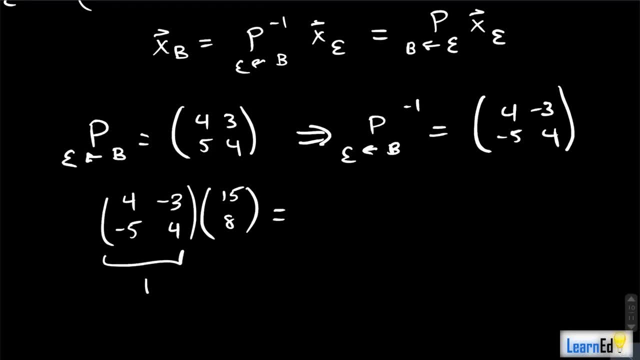 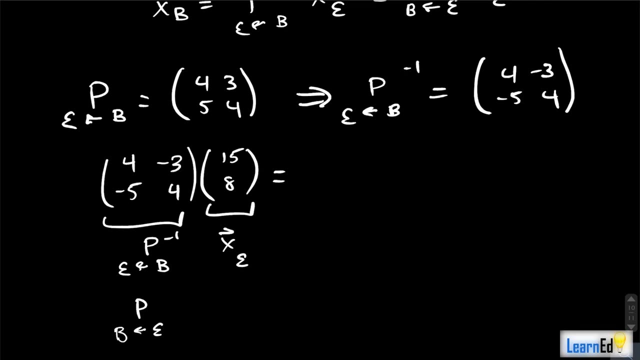 Okay, And so this is P from B to E, inverse, And this is XE. Okay, You can also write this as P from E to B. Alright, And now we're going to get what XB actually is. So we have 15.. 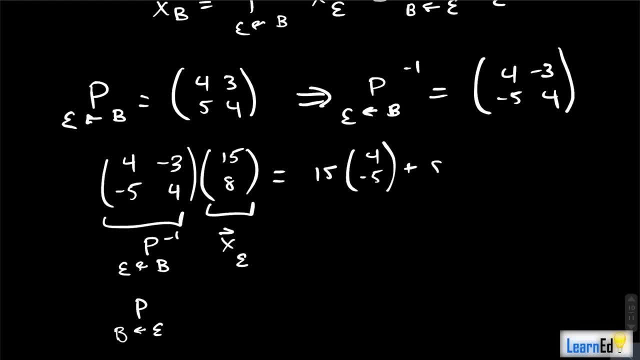 Times 4, negative 5.. And we're adding 8 times negative 3, 4.. And alright, Well, let's see what we can get here. Well, first off, this will be a 60, negative 75.. 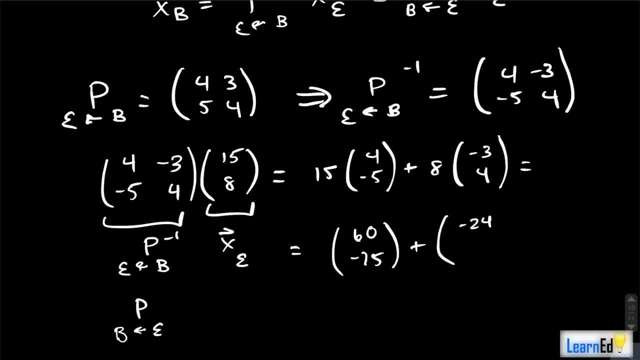 And then we have plus. This becomes a negative 24.. And a 32.. And now we just got to add these things together. Okay, So we end up getting a 36 here, And right here this is going to be: a 75 minus 32 is 43.. 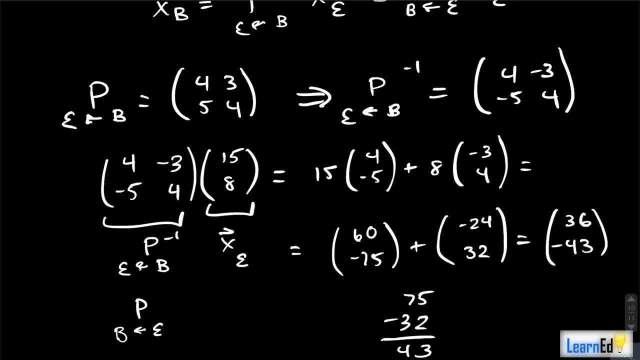 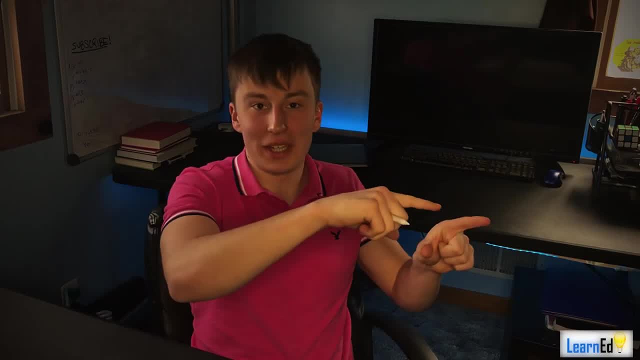 And we make that negative. That's actually how I- I'm sure that's how you guys think too, But like that's how I got through having like larger negative numbers And then like having to add a number to it or something like that. 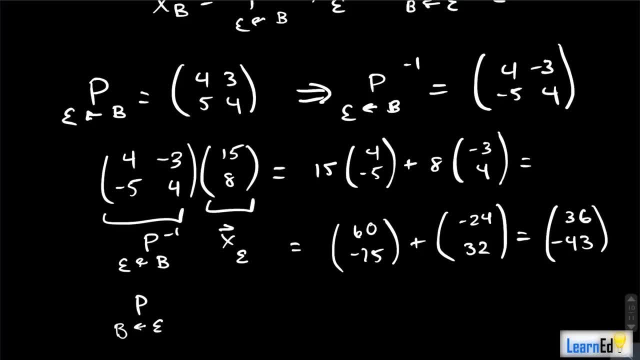 Like that's how I actually did that back in like grade school. So, anyways, Enough about my life story. That is the end, The answer to this problem. Alright, So for problem 20, we're going to shift our focus to dimension. 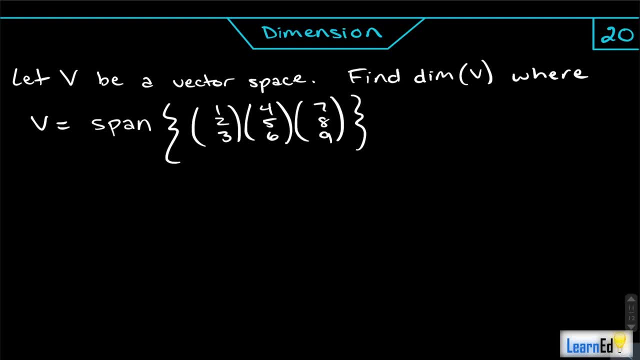 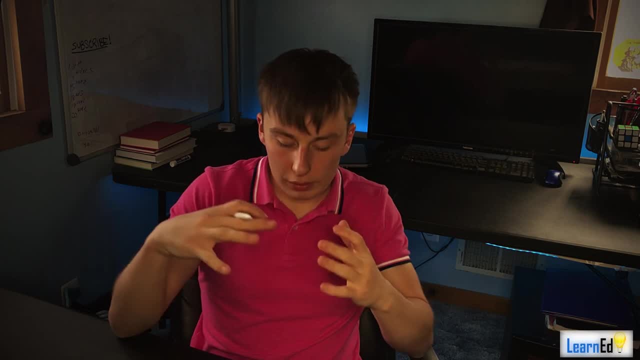 This problem says: let V be a vector space And find the dimension of V, where V is the span of 3 vectors. So to better understand this concept here: Just because we have the span of 3 vectors does not mean that we are now talking about. 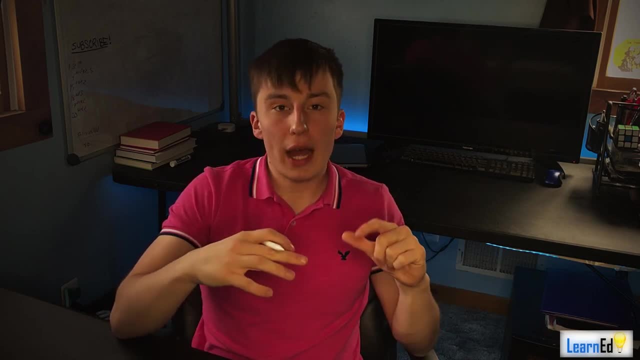 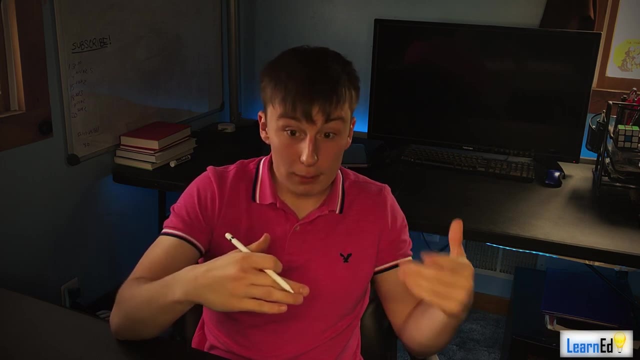 a 3-dimensional problem. We are talking about a 3-dimensional space. We could have the span of 3 linearly independent vectors. Okay, And that will definitely be 3-dimensional, But if these are linearly dependent, these vectors, 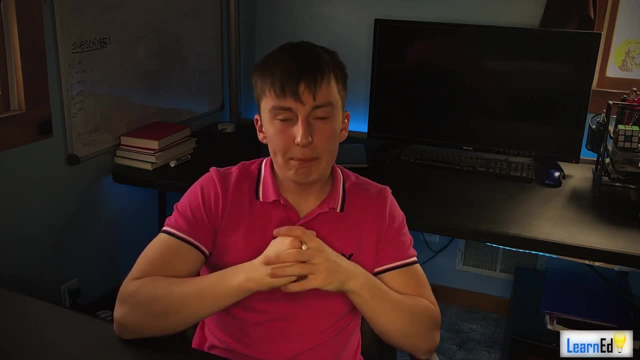 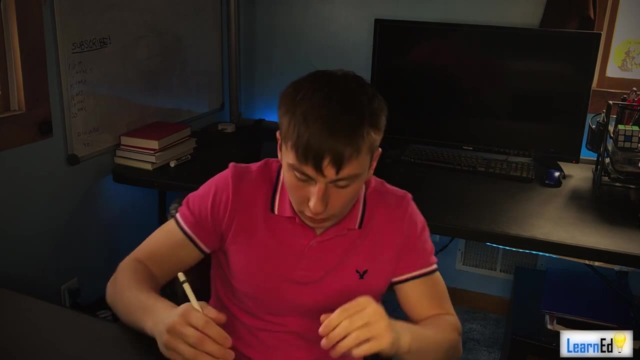 Okay, And we're taking the span of that. So let's say we have something like 1, 0, 0,, 2, 0, 0, and 3, 0, 0.. Right, Let me actually write that down so you can see what I'm saying. 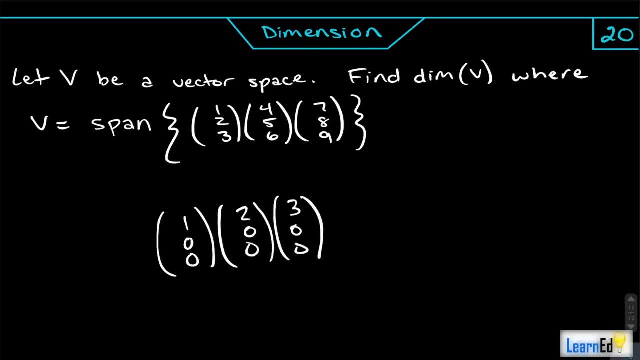 Okay, If we have the span of these 3 vectors, these 2 vectors are redundant, Right? We're still going to be spanning just a line, Right, And that's all that this is going to be. This will just be a line. 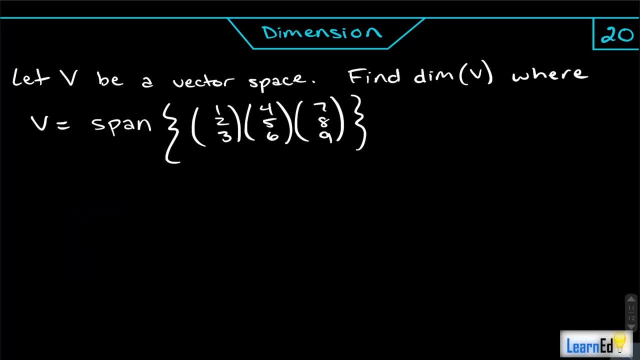 This will not be 3-dimensional, This will be 1-dimensional, in fact. Okay, So the span of these 3 vectors could be a line, It could be a plane And, of course, it could be all of our 3.. 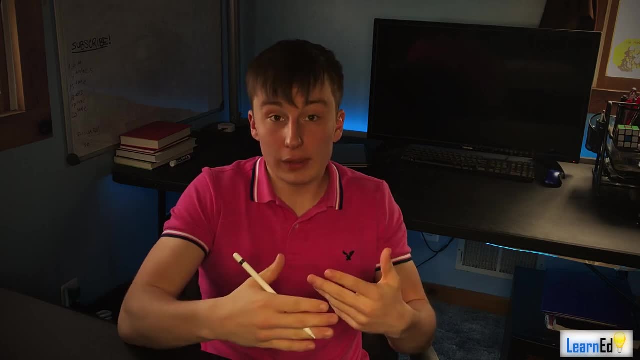 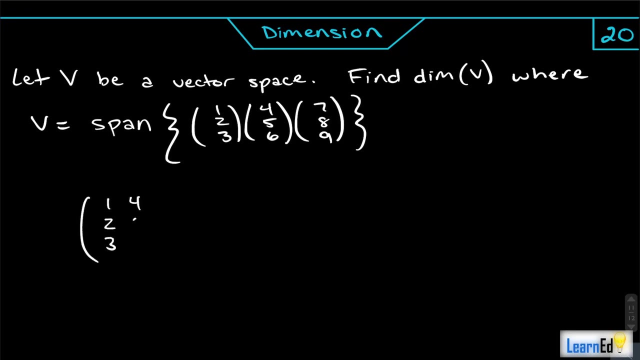 But we need to figure that out by row reducing here. Okay, So we need to see if these guys are linearly independent or if they're dependent. And if they're linearly dependent, to what degree are they linearly dependent? So we're going to go through the first step of row reduction. 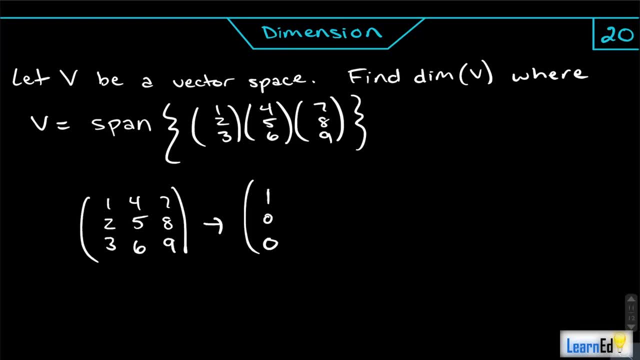 Here just zeroing out the entries under the first pivot. And to do that, Okay, Well, we had to multiply the first row by negative 2 and add on to the second row. Okay, So that gives us negative 8, and then plus 5 is going to be negative 3.. 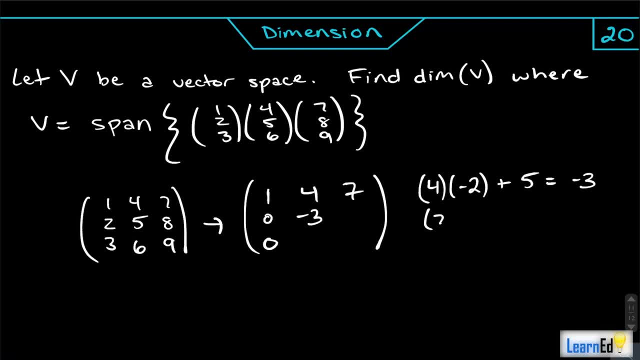 Doing the same exact thing. we have a 7 times negative. 2 gives us negative 14 plus 8 gives us negative 6.. Then we have we move on from getting our third row to be zeroed out in the first column. 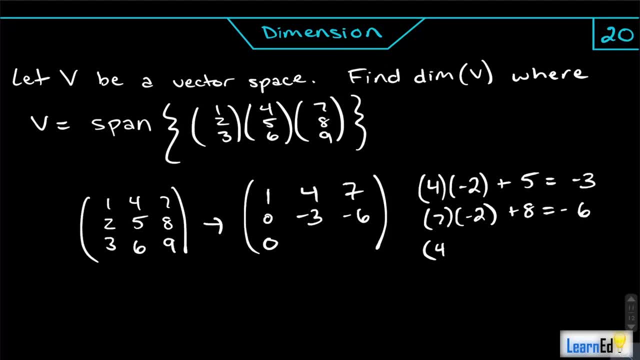 We have to multiply by negative 3.. So we do have a 4 times negative. 3 is negative. 12 plus a 6 is going to give us negative 6.. And we have a 7 times negative. 3 is negative. 21 plus 9 is going to give us negative 12.. 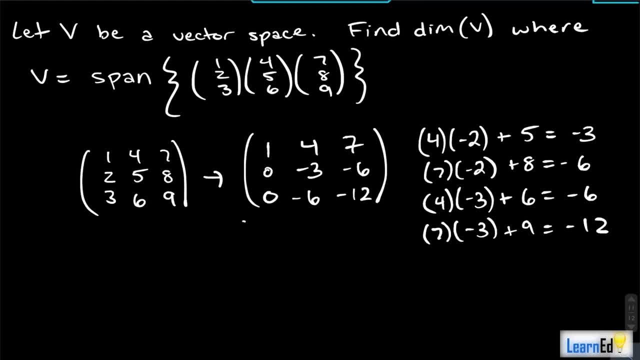 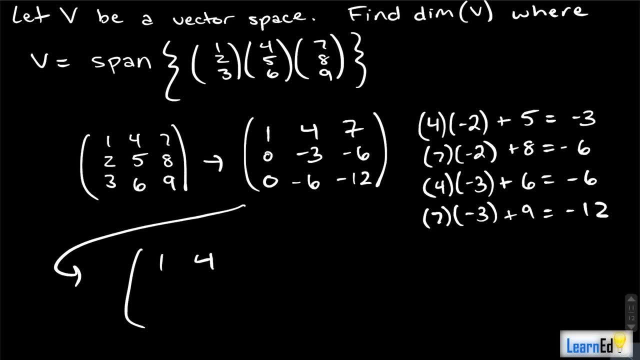 Now, here you can see that the second row is a scalar multiple of the. the third row is a scalar multiple of the second row. Of course, vice versa, but to make things easier, what we'll do is, first off, we'll 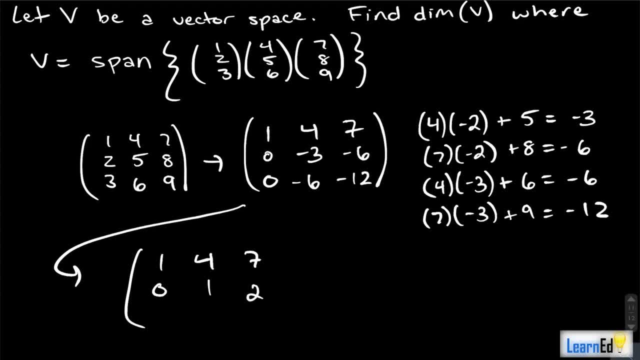 reduce this second row to make it look a little nicer, Just because I want to do that, And then we'll zero out the third row. Here we now have something in row echelon form. Okay, We have our two pivots. 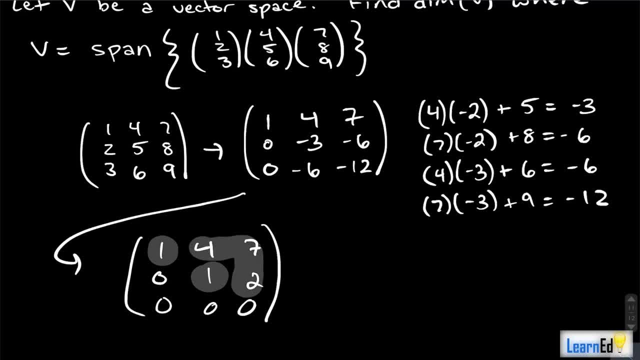 Okay, And everything else is we? we don't really care about that. We can just zero that out, Right, And and? and here's more of the intuition by why we can already assume that this is linearly independent. 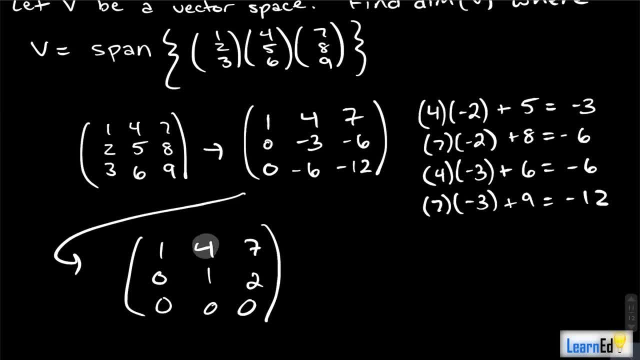 Okay, We can zero this value out, Right, And that won't change this, because this is a zero here. It will change this because it's a 2 here, Right, But that doesn't matter, because what's going to happen in the next step is once that's. 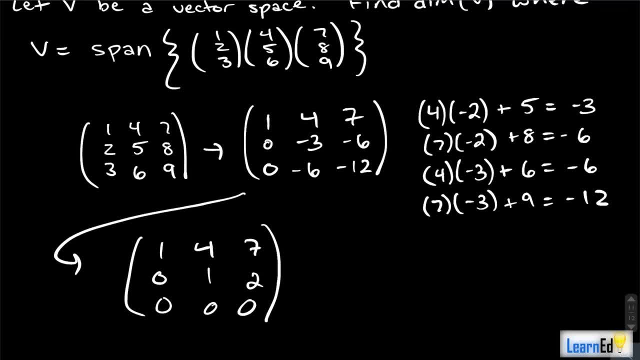 zeroed out. We can just. we just have a free column, Okay, This doesn't matter. None of these values matter here, because there's no pivot in that column. Okay, So it's just a free column, It doesn't matter. 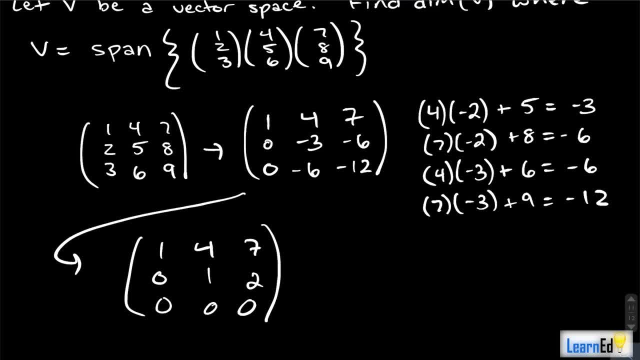 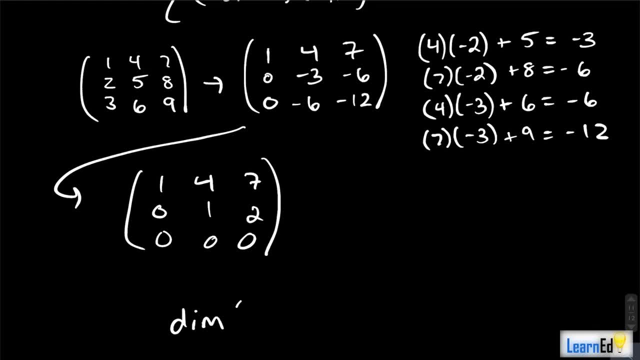 We can already see that this is in. since this is in row echelon form, we can say that these are linearly dependent and that we have two pivots. So the dimension of V is 2.. Moving on to problem 21.. 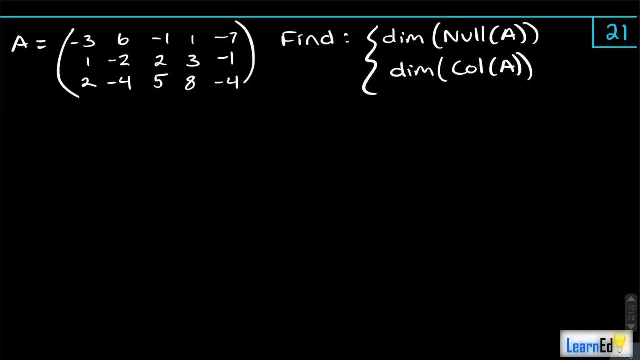 We have a 3 by 5 matrix A and we want to find the dimension of the null space of A and the dimension of the column space of A. Now, this is actually a matrix that we dealt with in problem 14.. Okay, 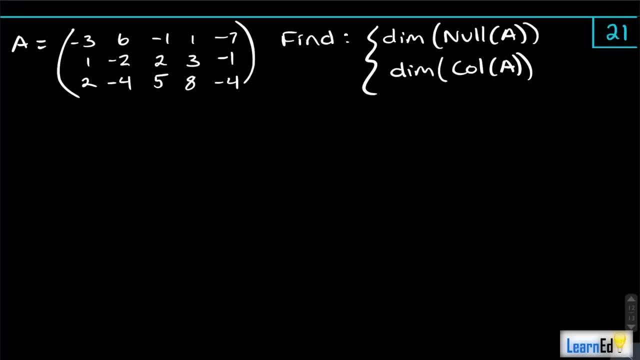 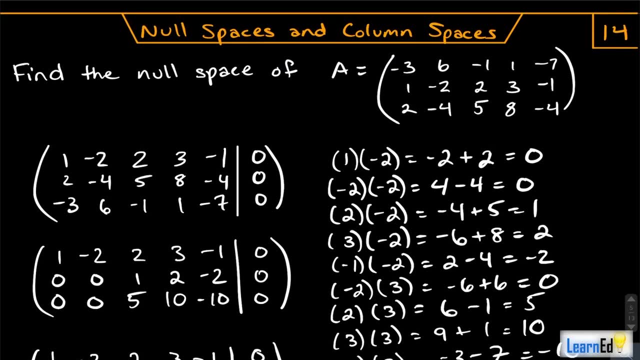 And so it may look familiar. I'll actually go back up and show you that right now. So we've already row reduced this and found the null space. Okay, That was this problem right here, where we had to find the null space of A. Okay. 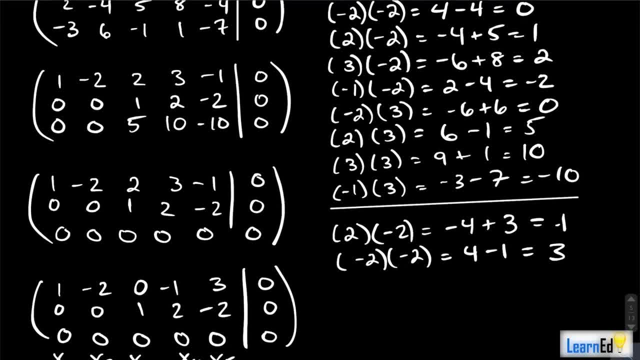 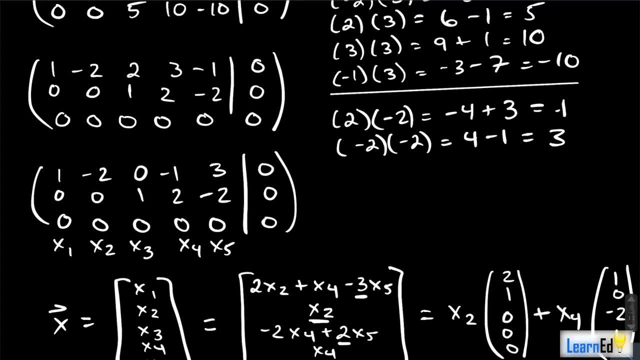 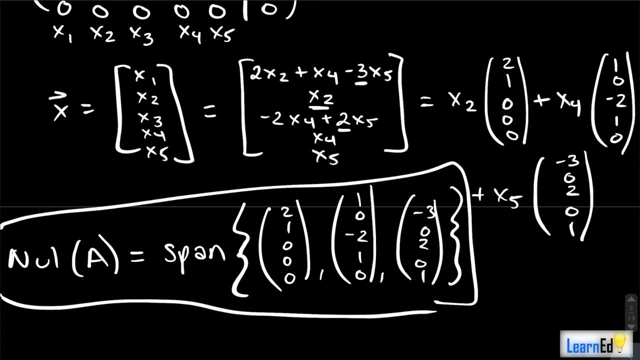 This is the same matrix here, and we row reduced it and we got to this point right here. Okay, Now we already saw what the dimension of the null space was. Okay, Spoiler alert, There's three vectors, Okay, And these are using this method. these are all linearly independent vectors. 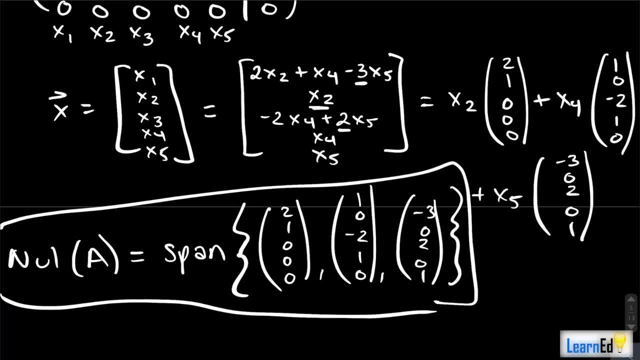 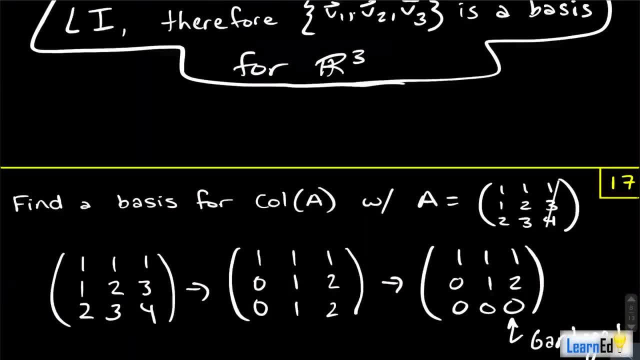 Okay, And you can verify that if you'd like. Okay, But we see that the dimension of the null space is 3.. Okay, But I'm going to, I'm going to show you this matrix anyway, so I can show you that. 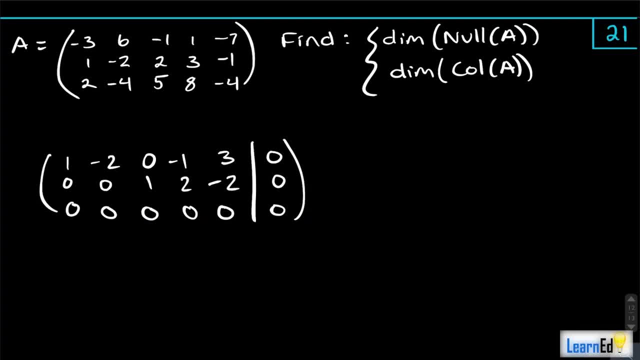 Okay, Here's something interesting- And we'll talk about this a little bit more with the rank theorem. Okay, What we have right here is we have two free columns, Okay, And we have- Sorry, no- Two non-free columns and three free columns. 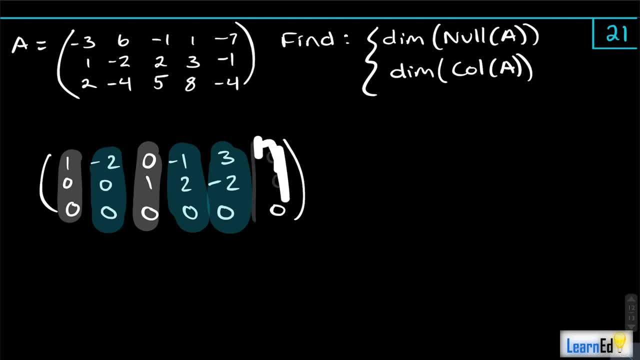 Okay, And we can kind of take away this augmentation with this, This augmentation with zero here, Because that doesn't matter. Okay, Now we have three free columns, So that means that the dimension of our null space is going to be. 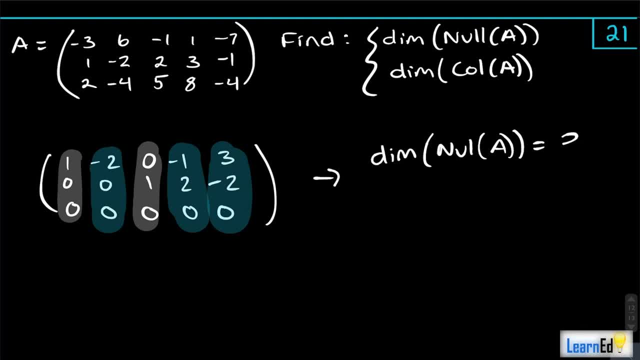 And this is usually only one L. That means that this is three, And since we only have two columns that aren't free, we get that the dimension of the column space is actually two, Right? So that goes back to when we found the basis for a column space. 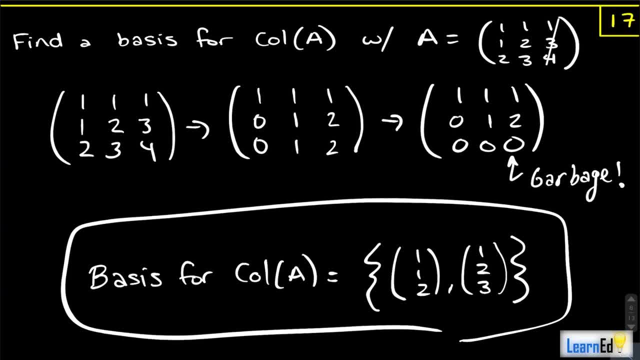 Right, We had a matrix A We row, reduced it. We found that one of these rows was free. It was a non-pivot column. Okay, And so basically, Or sorry, One of these columns was free. That's why I messed up. 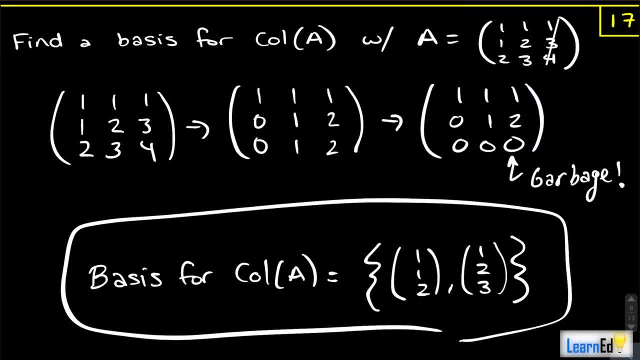 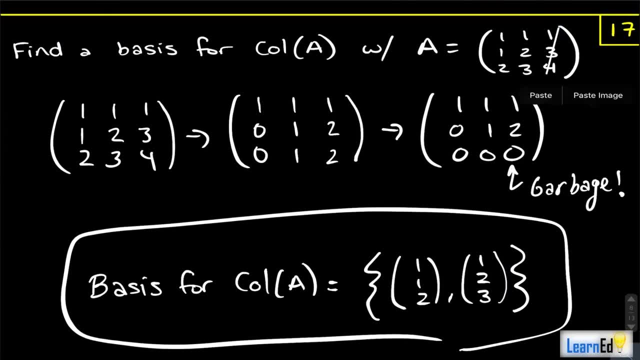 Yeah, One of these columns was free, And so we know that this basis only has two values. This basis only has two vectors in it, Right? The other vector is garbage, Okay, And so this dimension of, In this case as well, the dimension of the column space, is two. 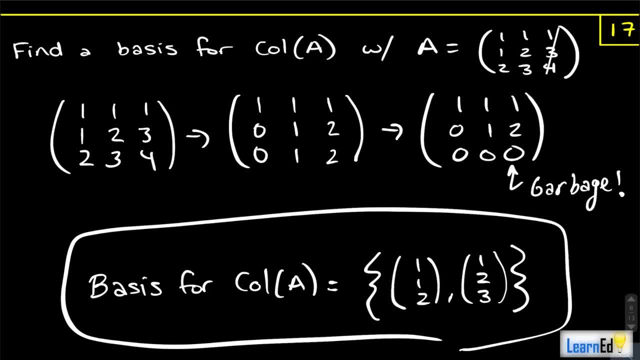 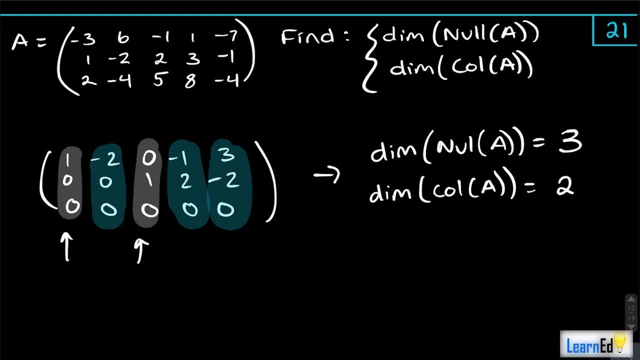 Right, It's how many vectors are in your basis. Okay, That's another way of putting it. So that's how we got this answer here. Okay, All right, So for problem 22.. Now we're going to be talking about rank. 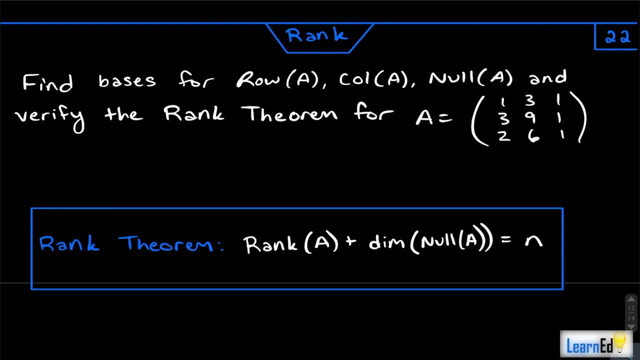 Okay, So we want to find basis for the row space of A, the column space of A, the null space of A, And we want to verify the rank theorem for a 3x3 matrix A. Now I have the rank theorem listed below, but we have a more pressing issue. 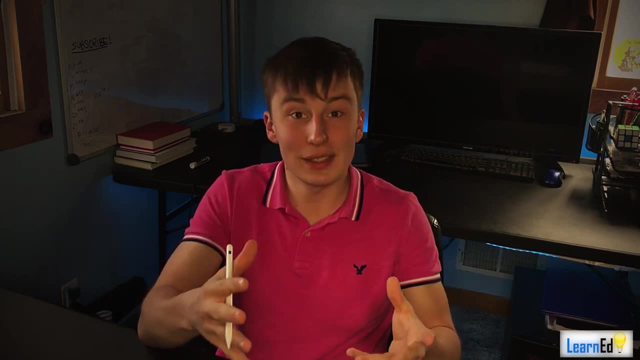 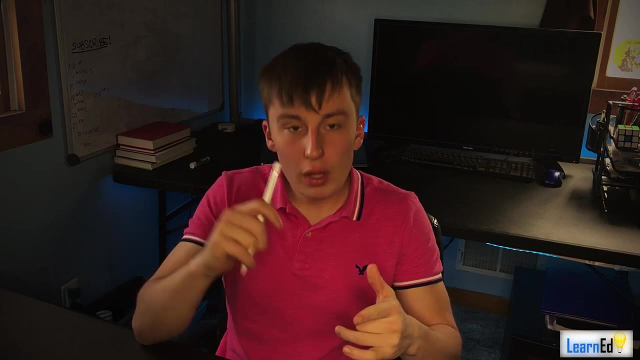 And that more pressing issue is: what the heck is the row space? We have the column space, the null space. Now we have a row space. What is going on, Right? So the row space of A is basically just all the possible linear combinations of the row. 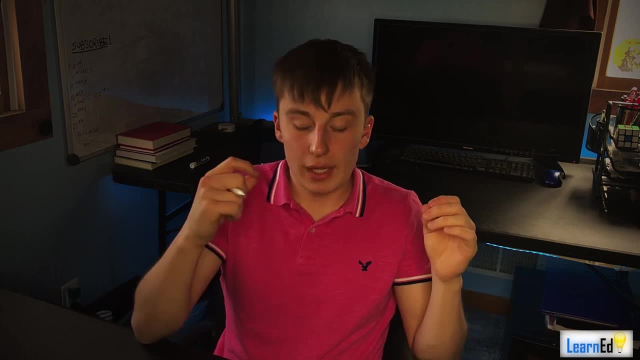 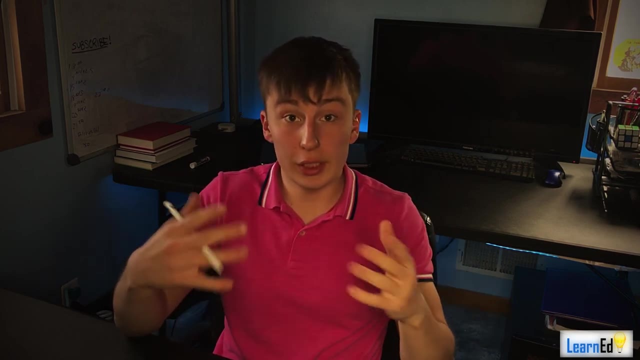 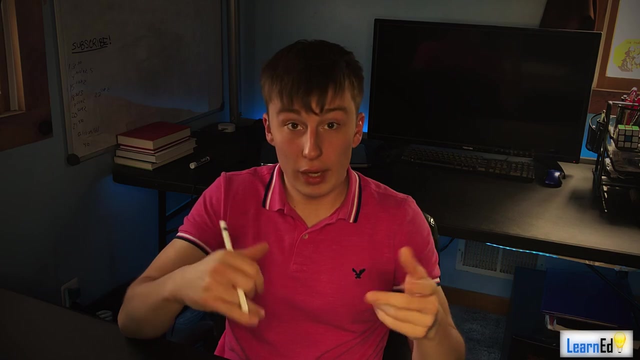 space of A. Okay, It's not the column space, but it's very close to the column space, which is all the possible linear combinations of the columns of A. Okay, So that is the idea there. Okay, So now let's just start row reducing this matrix, and the row space is just going to. 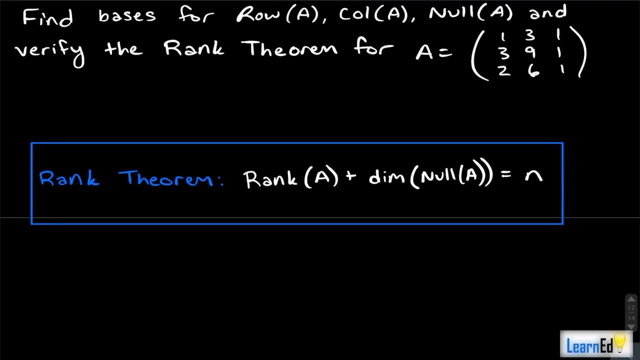 pop out. Okay, And well, we already have the row space of A Right. We can already find that here, Right. So, putting the columns, we span the rows of A Right And that's the row space. 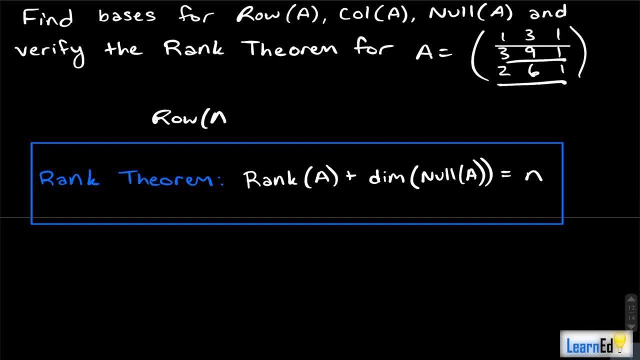 Right. So the row space of A here is just the span of you could do. you know 1, 3,, 1,, 3, 1, and you have 3, 9, 1, and you know, et cetera, et cetera. 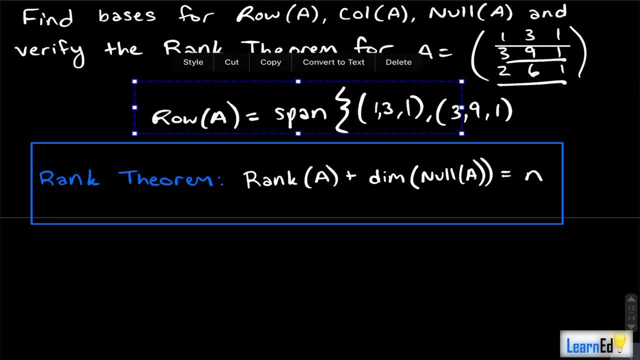 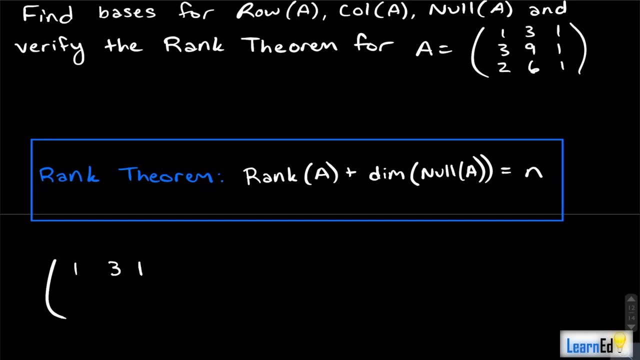 Right. So that's the row space, just to show you that, Right. But Now actually finding a basis for it, we need to see, okay. well, what rows are garbage? Okay, And that will also lead us to finding the, you know, the basis for the null space. and 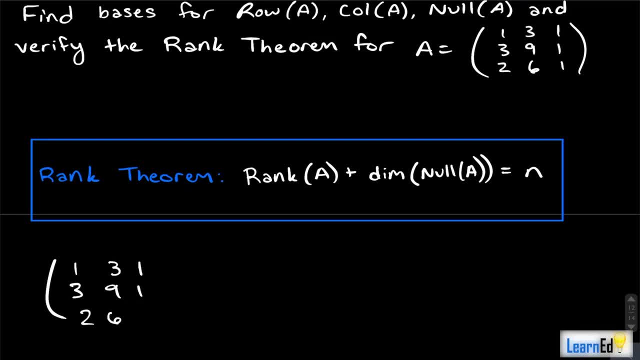 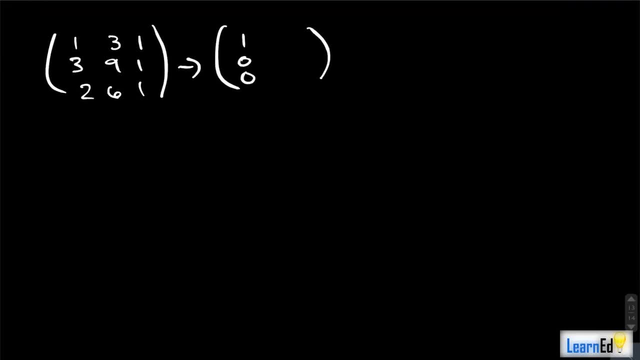 the column space as well. If we zero out the first two entries under the pivot, the first pivot we keep our first row and our second row. To get that zeroed out, we need to multiply the first row by negative 3 and add on. 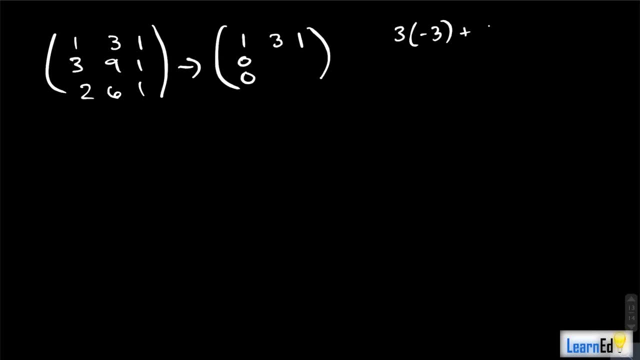 So we have a 3 times negative. 3 plus 9 is going to equal 0.. We have a 1 times negative- 3, that gives us negative. 3 plus 1 is negative 2.. We have a. to get our third row to have a zero in the first entry, we need to multiply. 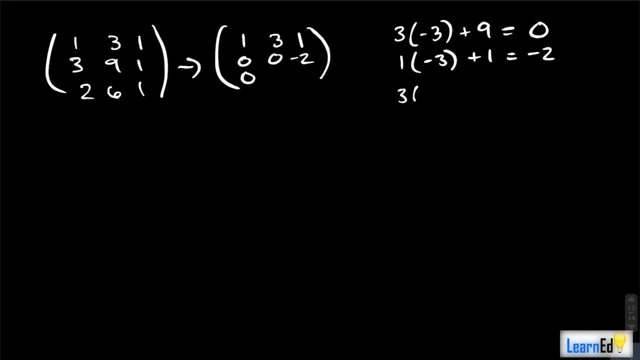 the first row by negative 2 and add on, So we have a: 3 times negative. 2 is negative 6.. Plus 6 is 0 and we have a 1 times negative. 2 is negative. 2 plus 1 is negative 1.. 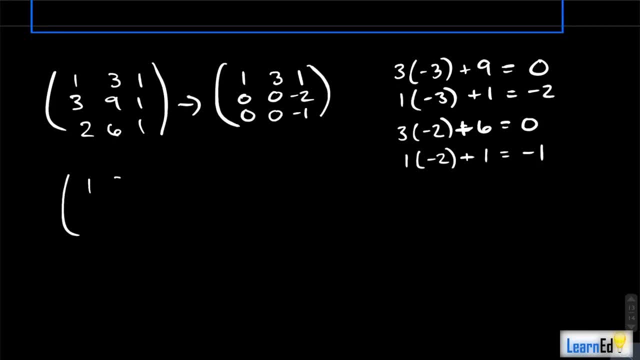 So now you can see that the second row and the third row are scalar multiples of each other, So we can just scale down the second row and zero out the third row. Okay, In which case We are sitting in row echelon form. 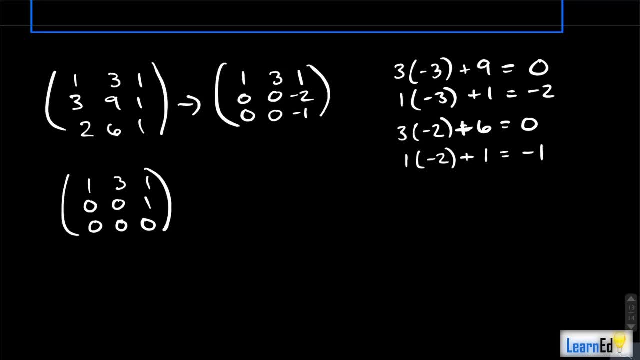 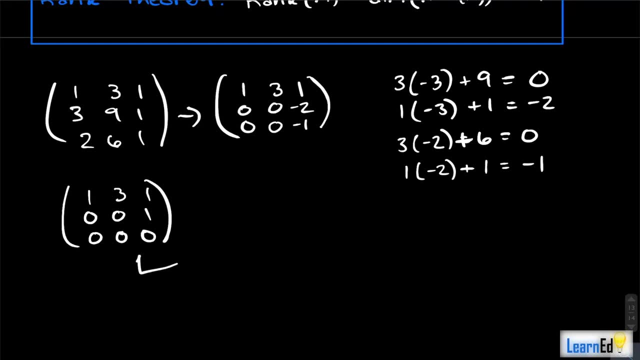 Okay, So we can now find the row space right- The basis for the row space, rather Okay, And we can actually use this matrix. We don't have to go back to this matrix like we did with the column space. 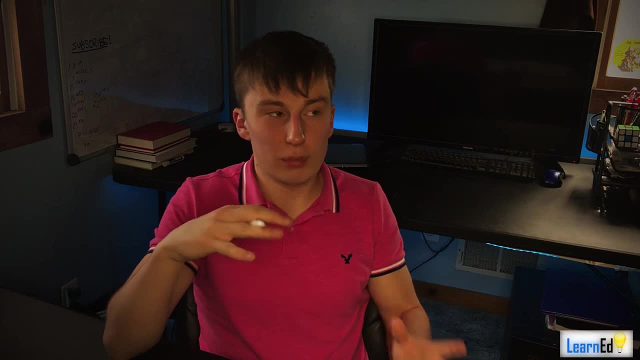 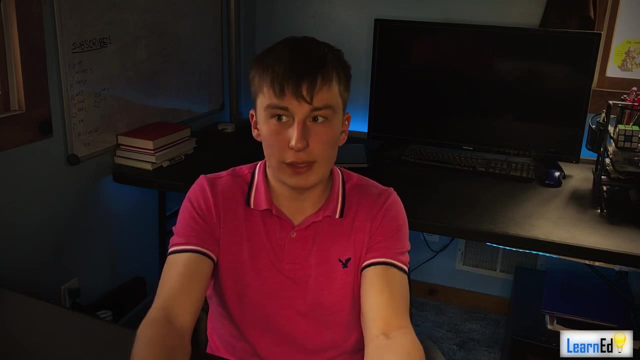 And there is like you can look at that stuff like more in depth if you want to, I'm sure you know you can look at like there's a theorem in your textbook- most likely if you, your textbook covers row space- which will tell you that you don't have to to find. 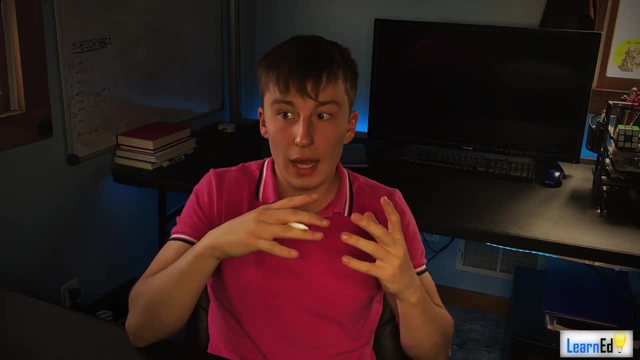 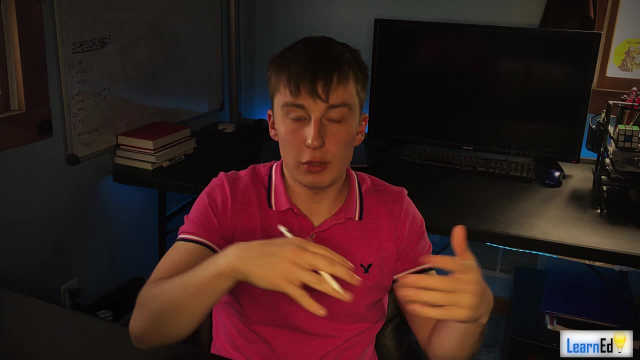 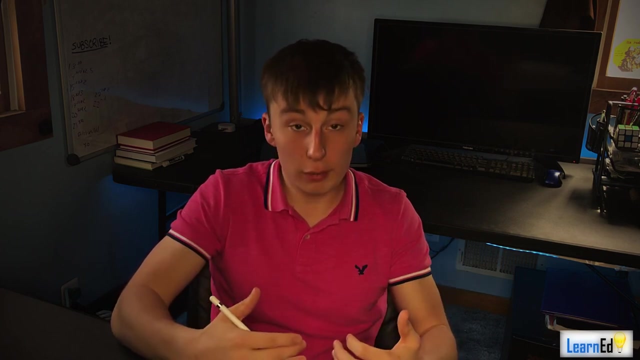 the basis of row space. You don't have to actually, you know, go through and go back to your original matrix and then use that original matrix. It's row equivalent to your, you know, if it's, if it's row equivalent to your final. 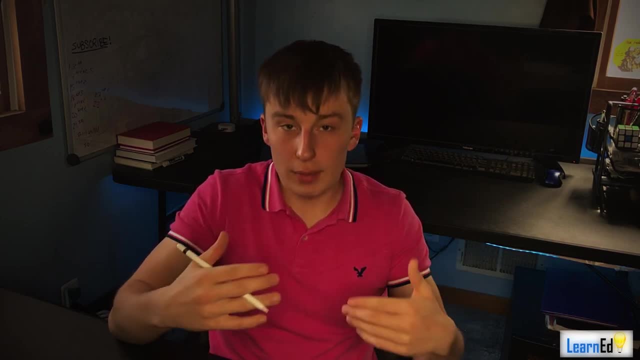 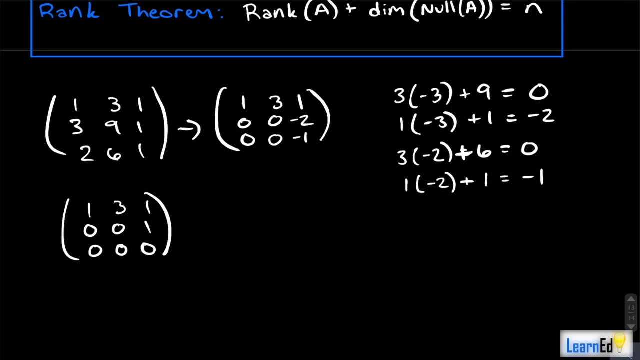 matrix. Okay, Which it is in this case. Right, That means that, okay, we can use this as a basis as well, and it's fine, It's the same thing, Okay, So. So we can say that a basis for the row space of A equals one, three, one one zero zero. 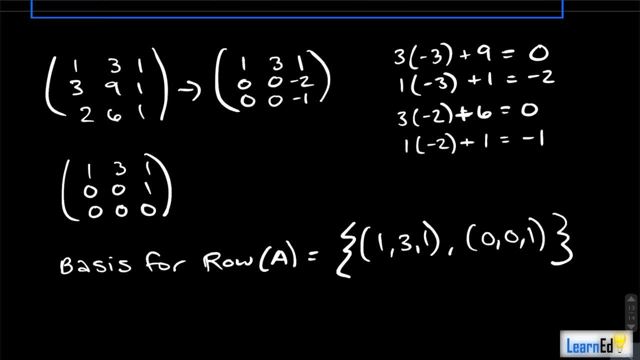 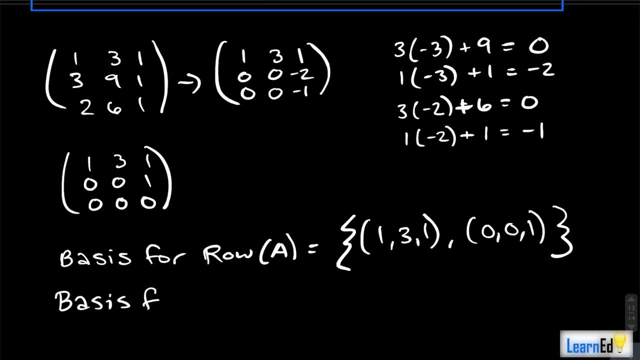 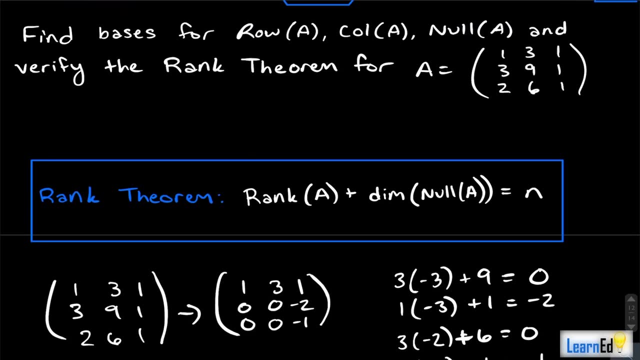 zero one. Okay, That's a basis for row A. Now a basis for the column space of A. Here we can still do the the basis for the column space of A, but we do have to go back up to the top and use this column and this column- because the middle column- we could. 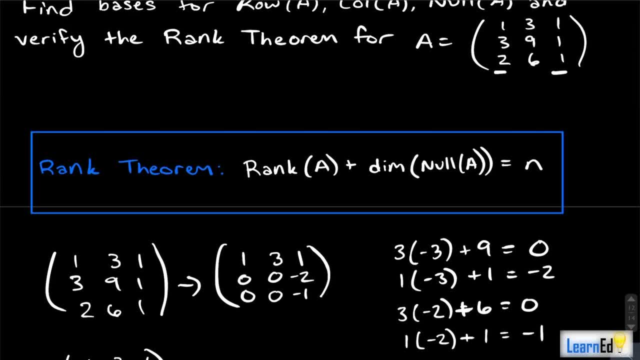 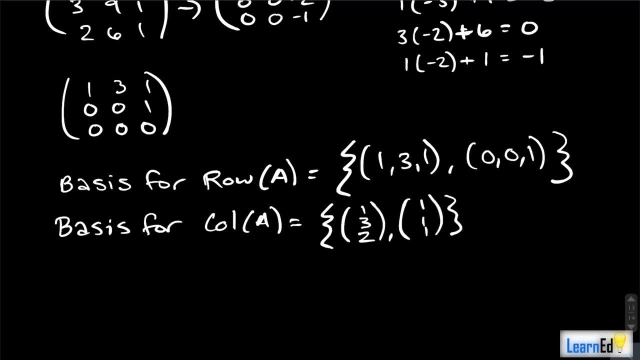 found out was linearly, was a free column. So we have one, three, two and one, one one. Okay, So we have a basis for the row space of A. We have a basis for the column space of A. 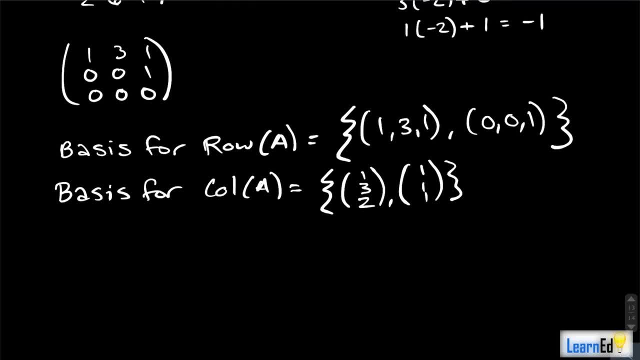 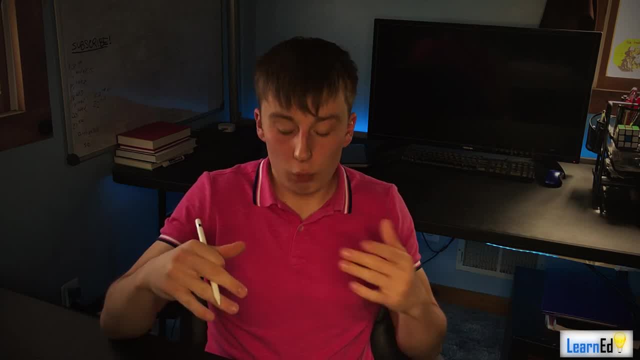 We need to find a basis for the null space of A, and that's going to require us to find the actual null space Right, Because The null space of A is well, how we're going to find it, using this method, the method that 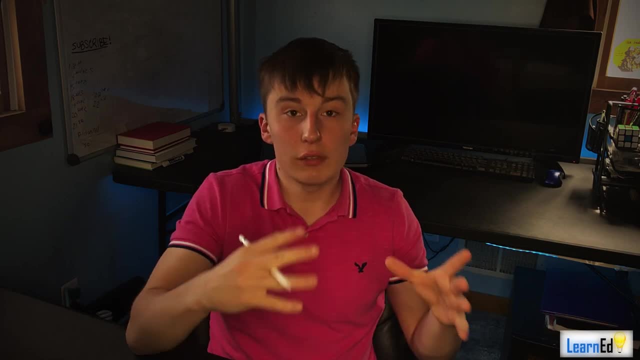 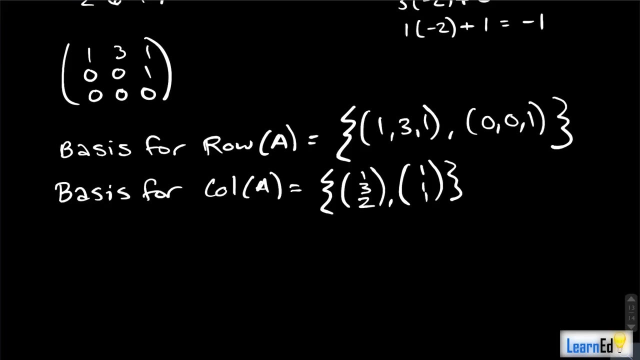 I used earlier as well. that gives us the basis Right, Because all of those vectors are linearly independent, and so it's a basis for the null space as well. None of those vectors are garbage, Okay. So what we have to do here, since we have this in a row, echelon form- is we just need: 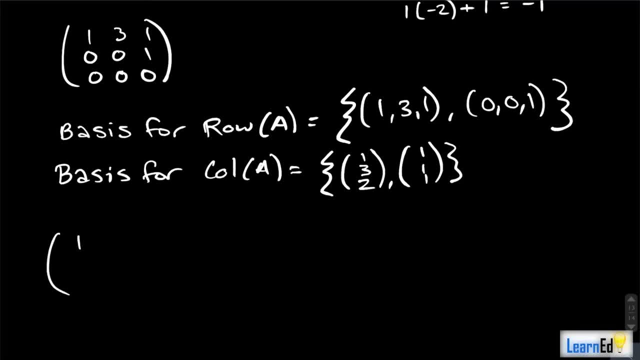 to get it into reduced row echelon form, And so we can zero this thing out without any effects. Okay, And so now we have that. your vector x- okay, will equal. well, x1 is just going to be negative. 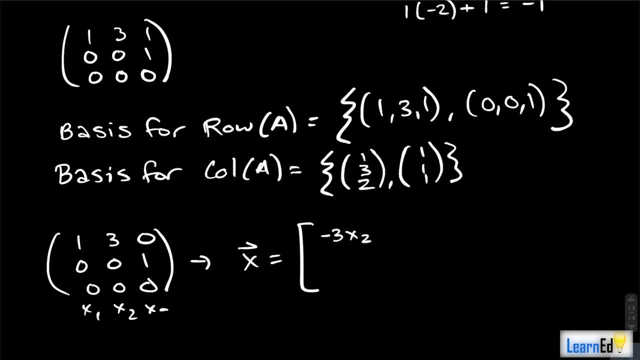 3x2.. Right, If we call this x1,, x2, and x3. You have your middle vector, which is free, and you have your last vector, which is just going to be Zero, I guess, Yeah, It would just be zero. 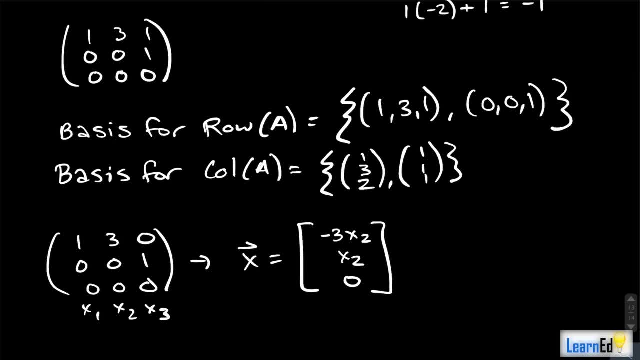 Right. So because? because here's why, Yeah, it's definitely zero. Here's why I was confused at first. but hang on, You augment this with zero to find the null space, And so here you just get the x3 equals zero. 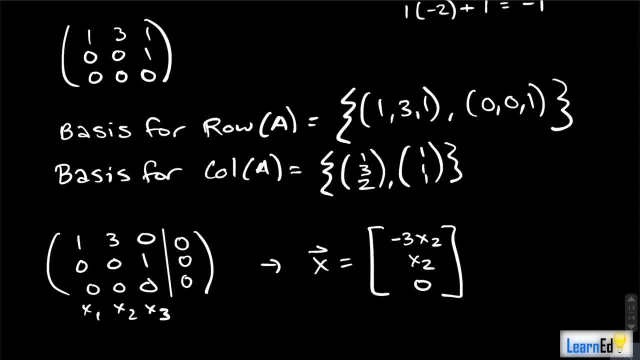 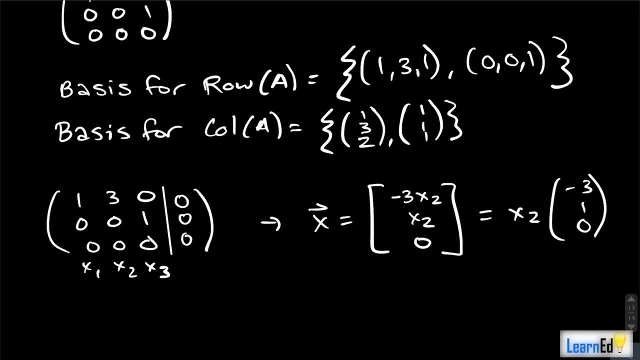 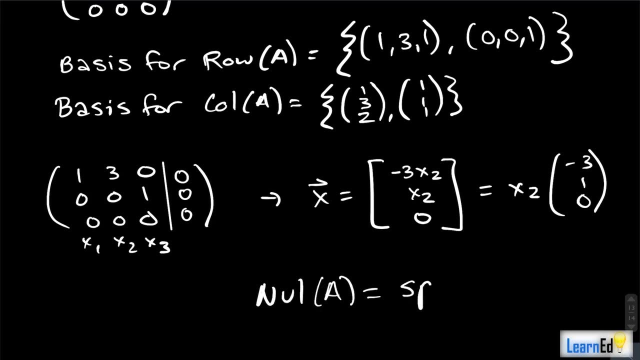 And that's what you just put it in here, Okay, So Here you just end up getting x2.. 10x2.. 10x 0.. And then that becomes so: the null of A equals the span of negative 3, 1, 0. 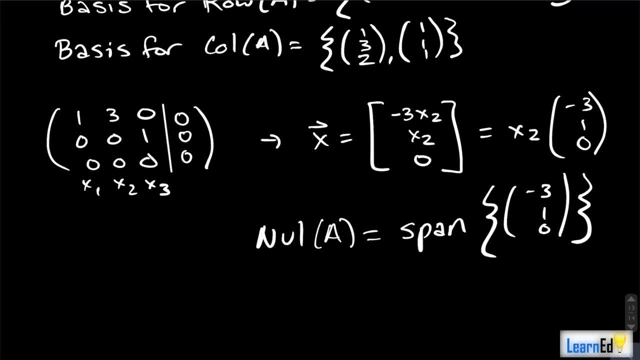 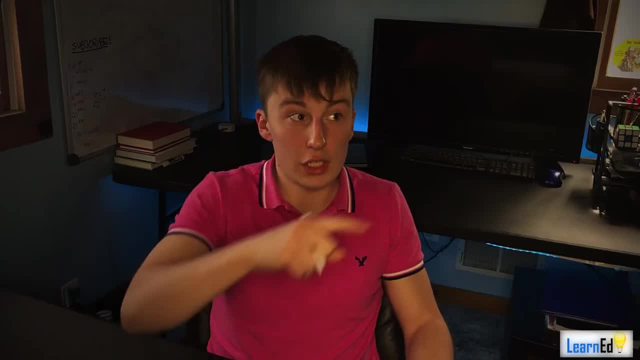 Right. So basically all the possible linear combinations that you can get by just multiplying that vector by stuff Or well, so it's not like a linear combination necessarily. You're just multiplying that by that vector by stuff and you just get a giant line. 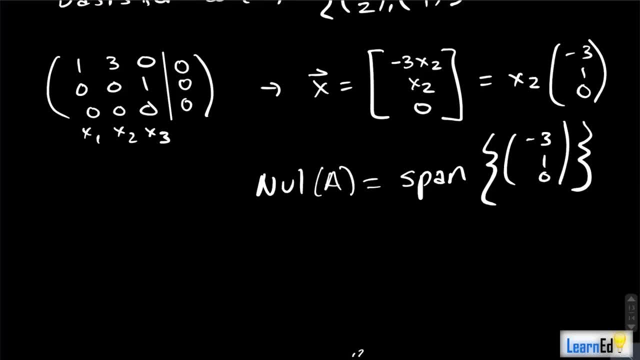 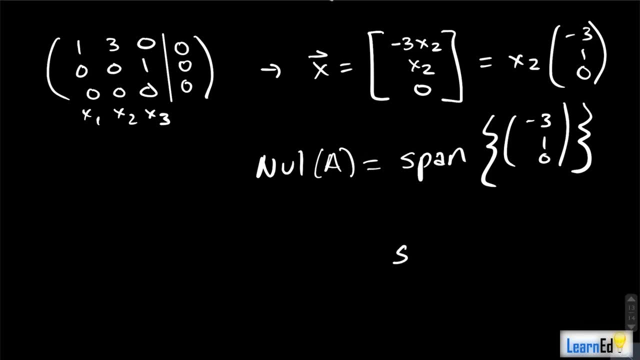 Okay, essentially what happens there. so that's kind of the span of this thing is just a line, right, like i talked about earlier in the video. so the span of one zero zero and i had like two zero zero and three zero zero, well, that just is the same thing as the span of one zero zero, which would 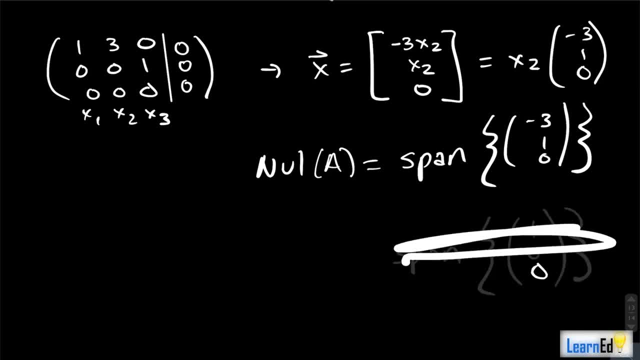 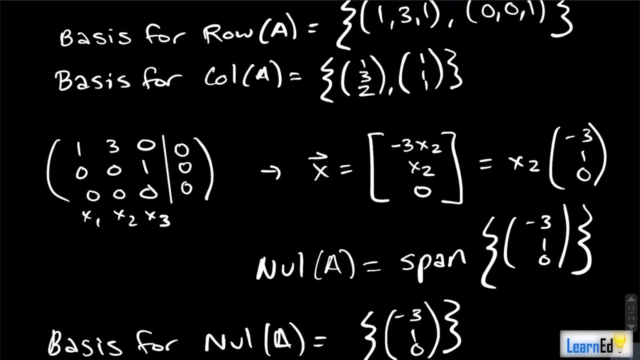 be a line, right? so, anyways, we can say that the basis for null a equals negative three, one, zero. okay, that can also serve as a basis. and so now we have the basis for the row space, the column space and the null space. what else do we have to do? we have to verify the rank theorem. 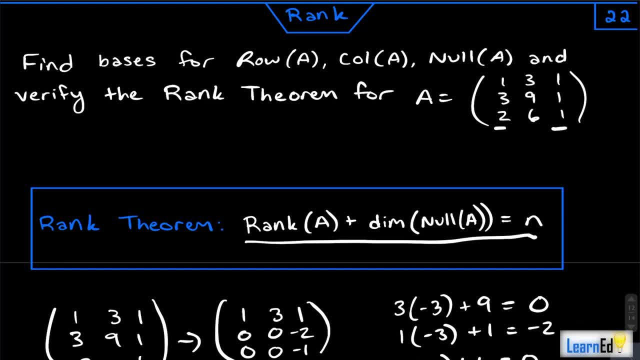 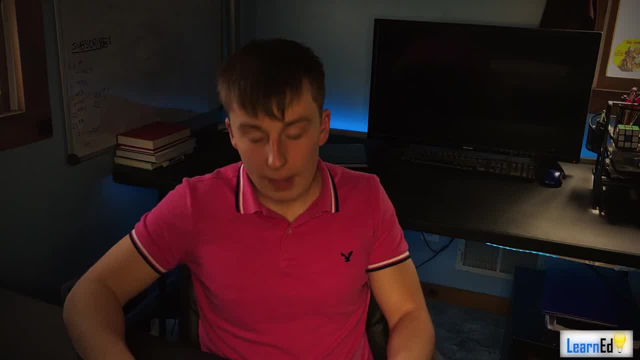 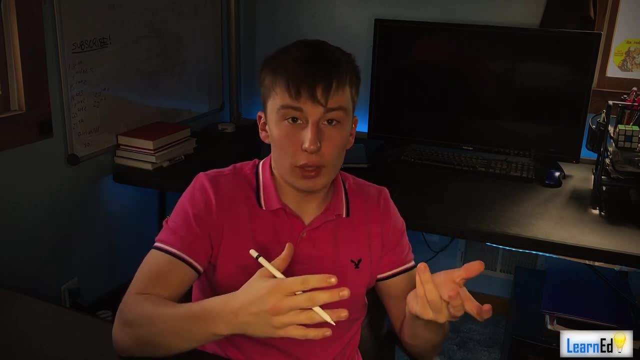 so we have that: the rank of a plus the dimension of the null space of a equals n, and that is the rank theorem. okay now, the rank of a, the rank of a, is the dimension of the column space of a. that's just, it's. it's like a fancy word for it in a way. okay, so we can, basically, if we, if we find the dimension, 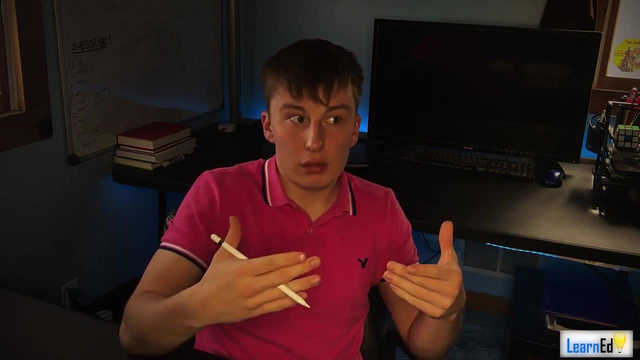 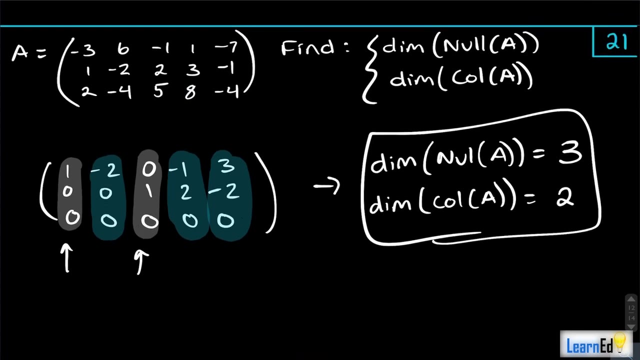 of the column space of a and the dimension of the null space of a add up to be n. we verified the rank theorem. okay, but if you remember, in the last problem it was exactly that right. here's n right. this is an m by n matrix. that's what's meant here. that's a terrible curly bracket, by the way, that's what i was trying. 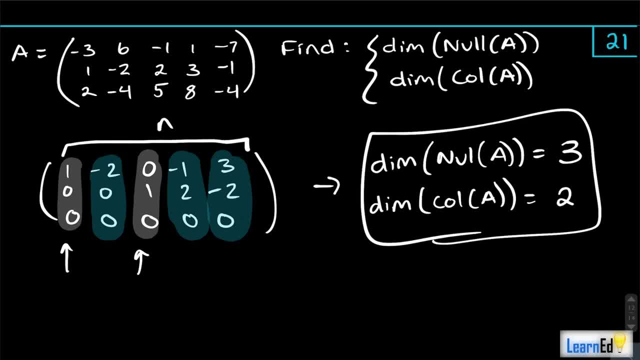 to do so. to stop embarrassing myself so much, i'll just do that. okay, here, the dimension of the null space of a is three. the dimension of the column space of a, aka the rank of a, is two, and that ends up, adds up to be five, which is what n equals here. 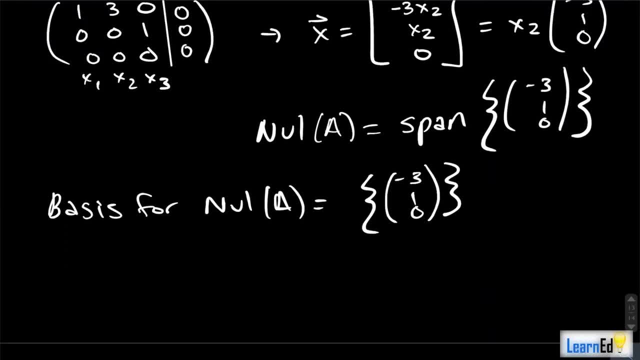 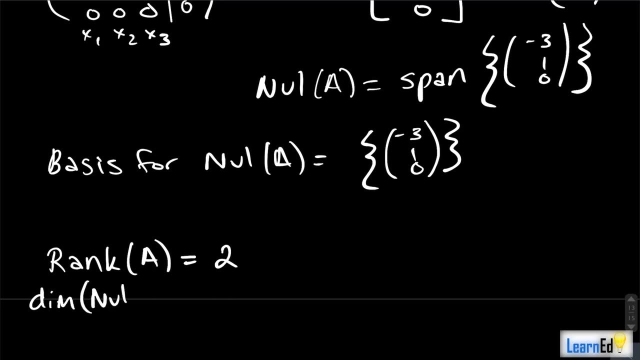 so all we're doing is we're doing the exact same thing here. the dimension of the column space of a. there's two vectors here, and that's also called the rank of a right. so that is two. the dimension of the null space of a, which apparently doesn't have a fancy. 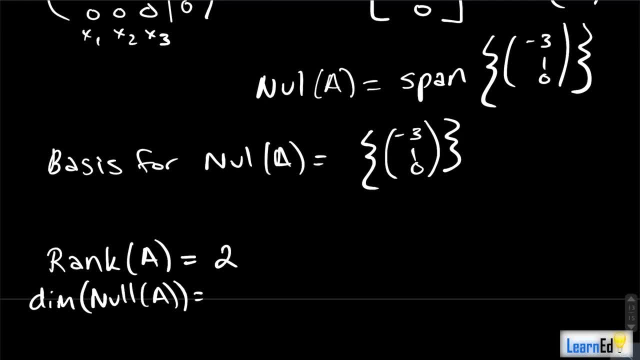 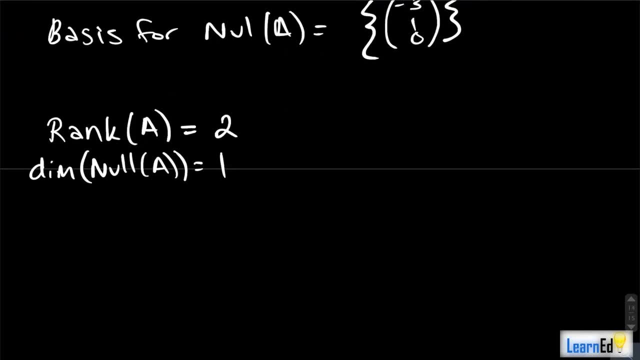 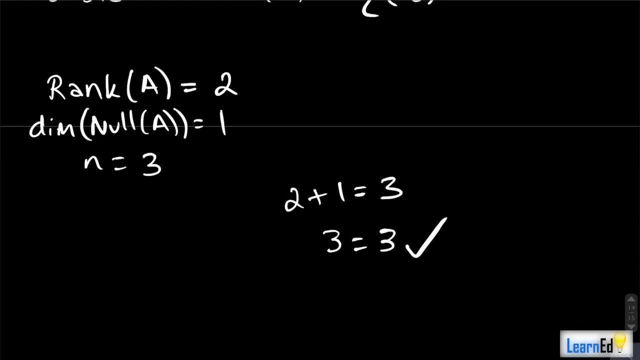 name, but the dimension of the column space does. whatever, this equals one. and well, how many columns are there in this? there are three. so you know, that's the rank of a and that's also called the rank of a, so that since n equals three, two plus one equals three, three equals three, bam, aren't rt. 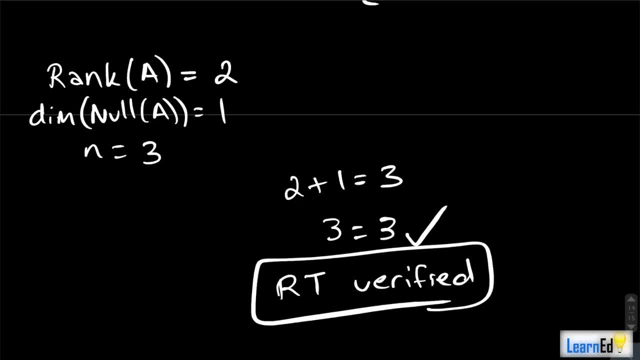 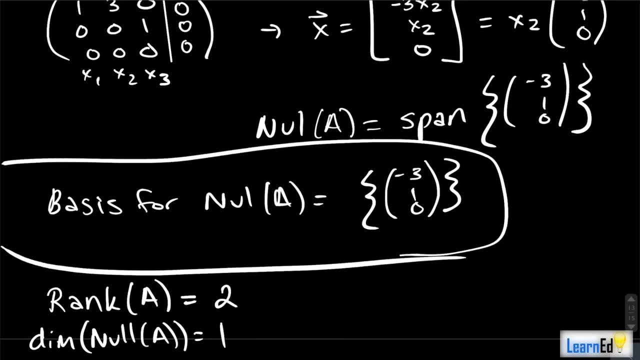 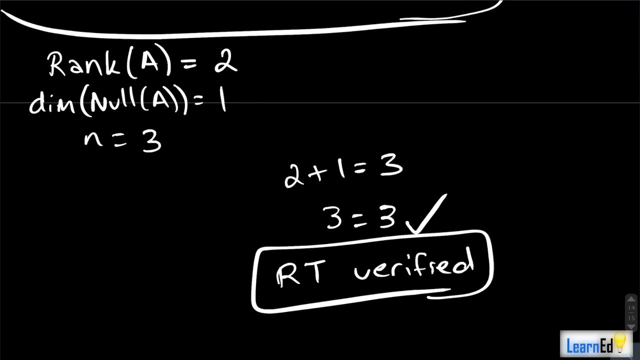 verified, okay, so we have all four things now. we can circle this and we can circle this and we have the rank theorem was verified, okay, so that is all for problem 22. so now we're going to move on to the final topic of the day. and we're going to move on to the final topic of the day and. 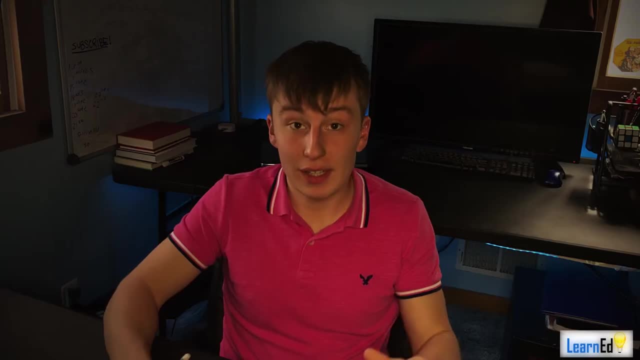 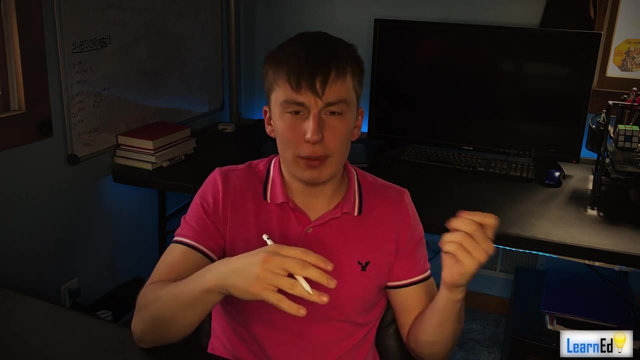 we're going to move on to the final topic for this video, and that is change of basis. now, this is something that i had so much more trouble with than i should have when i was in linear algebra because it, you know, while i said in, i believe i said in the beginning of the video that it was 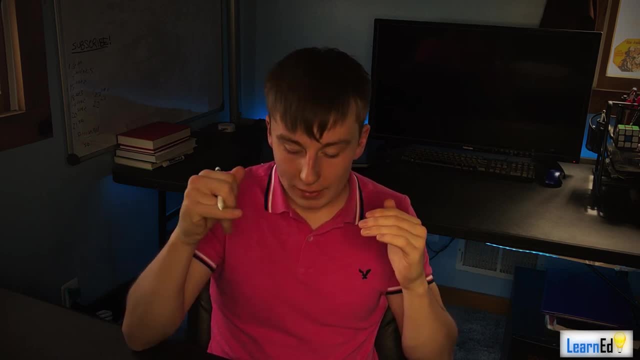 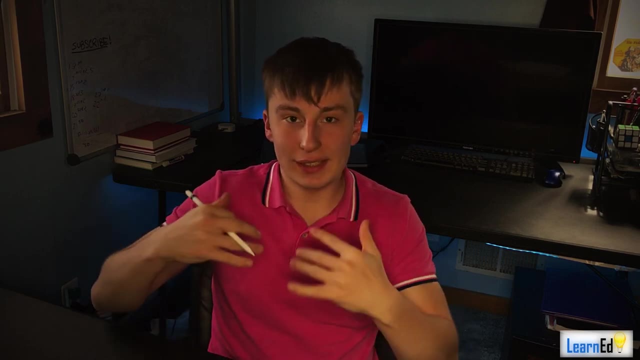 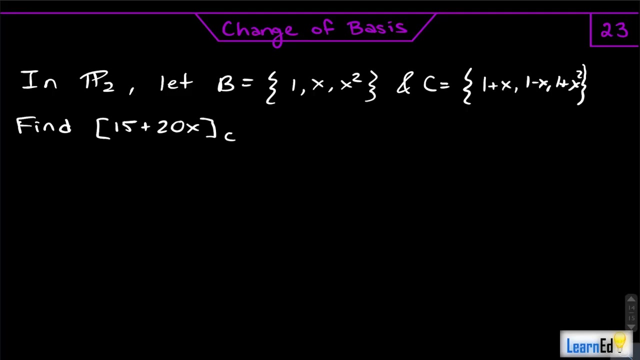 a difficult topic. it really is actually kind of straightforward when it comes down to it and it's just you know getting that right explanation, so it makes sense in your head. i think that's a big part. so anyways, let's get into problem 23.. so in p2, which it means you have a polynomial space with like up to degree two, okay, which. 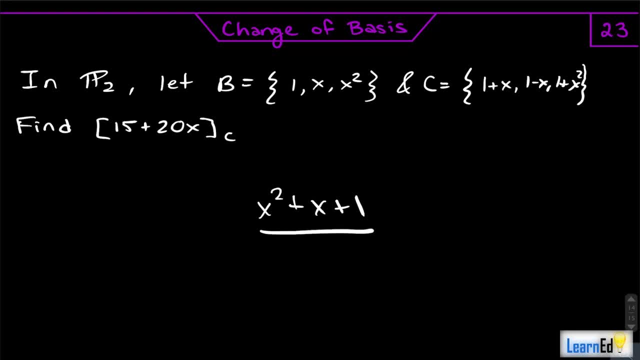 it's like x squared plus x plus one, right, that's in p2, all right. and you have b, a basis b, which is one x x squared, and you have a basis c, which is one plus x, one minus x, one plus x squared, and we want to find the coordinate vector of 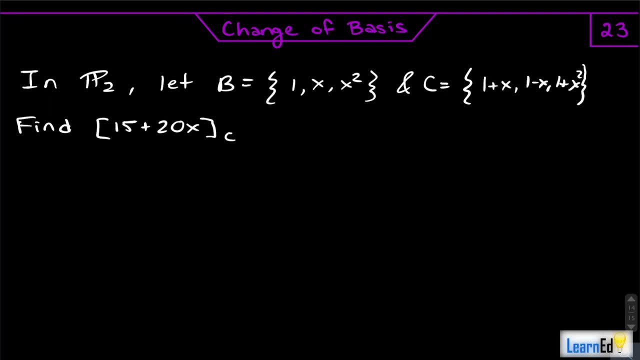 15 plus 20 x relative to c. okay, well, since this is basically, since b is a basis for p2, essentially right, one x x squared. this is going to be really easy to write: 15 plus 20 x in terms of of b, right? so we can say that. 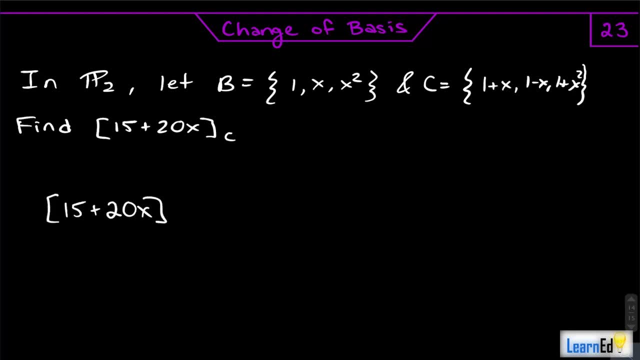 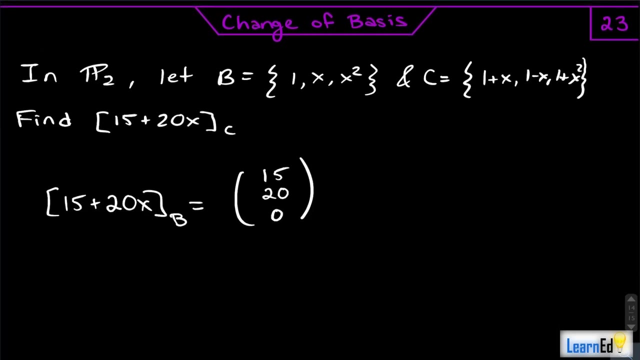 15 plus 20 x relative to b, is 15 20, 0. right, because there's no. there's no x squared part. okay, and well, there you go. that's not the hardest part of this problem, but it's, a you know, one of the hardest, because it's the. 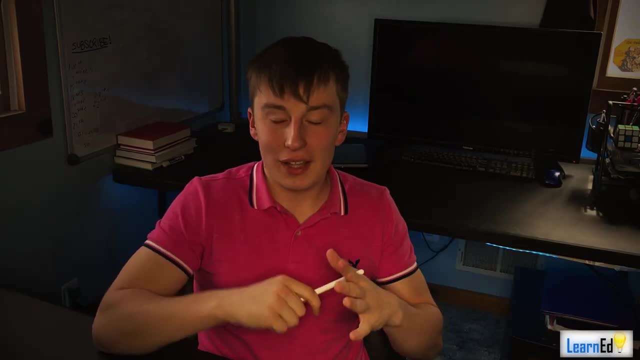 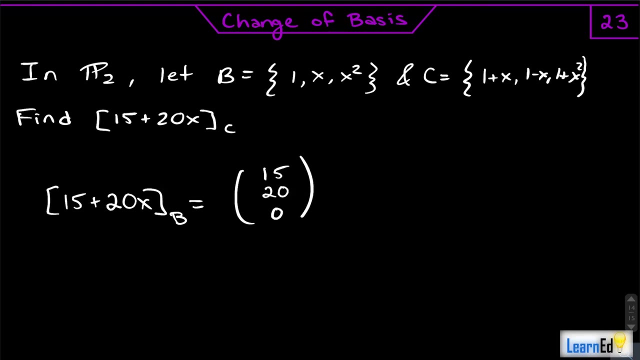 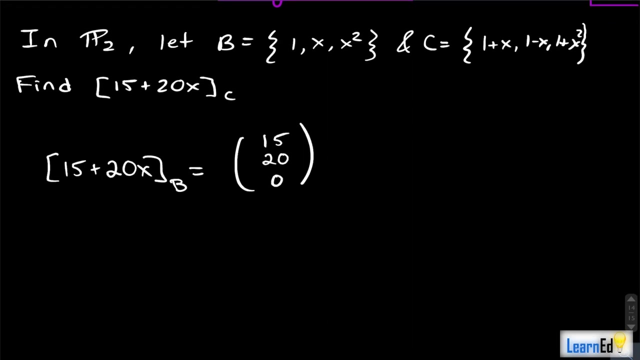 initial step right. starting the problem is always probably one of the hardest parts of the actual problem. right it's in? in most cases it is, but anyways, let's get back into this. enough of being just talking non-stop um. anyways, let's bring up that formula that we talked about in. 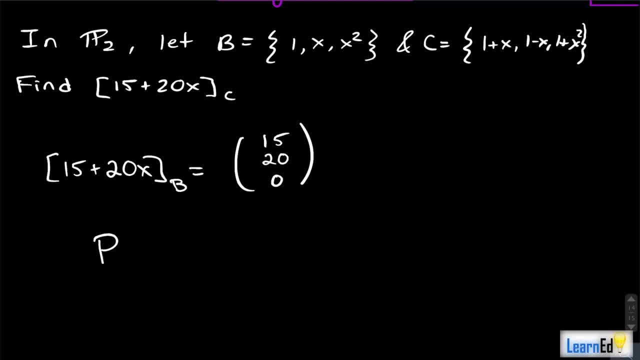 the change of coordinates section. we're going to have some change of coordinates matrix. we want to change coordinates of b to coordinates of c, relative to b to relative to c, and we're going to multiply that by a coordinate vector relative to b, because we're changing it to a. 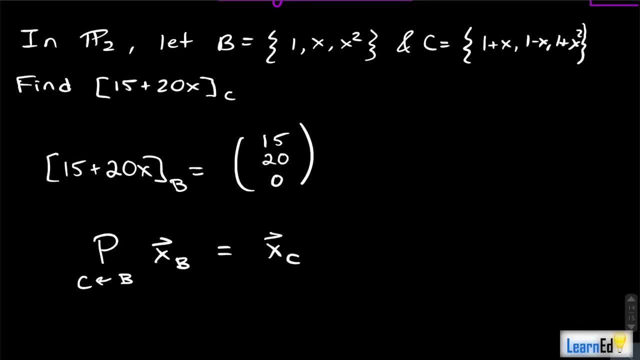 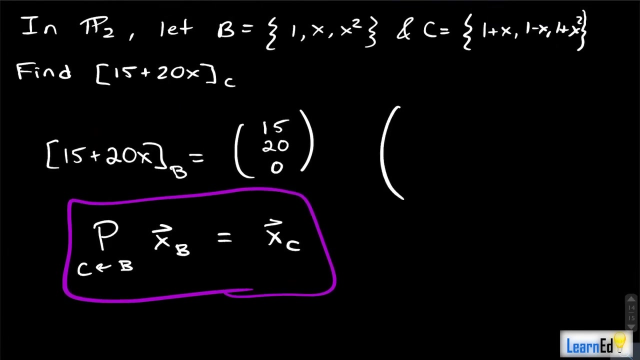 coordinate vector relative to c, right? so that's an easy way to kind of remember that. now we need to find this change of coordinates matrix, which is probably the hardest part of the problem. okay, because it's just. how do you actually go about doing that? well, here all you have to do actually is just have a matrix, okay, and you're. 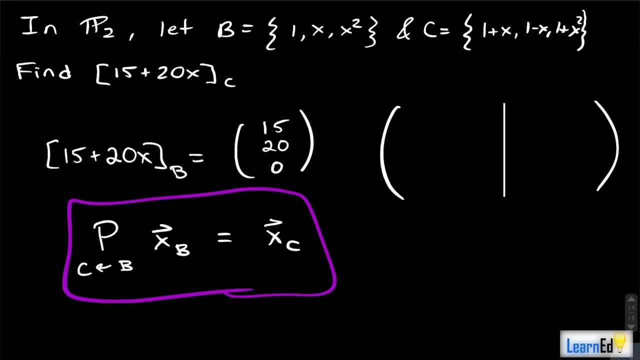 going to basically augment c with b. okay, and i'll i'll show you what i mean. so if we write c right, relative to the standard basis, we get one one zero right, that's one plus x. one minus x is one negative, one zero. and one plus x squared is one zero, one right. and if we write b on the other side, we get one zero. zero, zero, zero, zero, zero, zero, one. okay, and we're just going to start our step by presence error, right. so that makes one minus one, is one: zero, zero, zero, zero, zero. okay. and that makes one plus camera: one, zero, zero, zero, one. one, zero, zero, zero, one a plus. and then f equals b versus c times again. we pretend to be right and the inverse will yield 거의 one plus x, and josem pequeño is negative. there is a radish of a value of four plus f, so we can get oh right, and on the right here we want to get one zero. 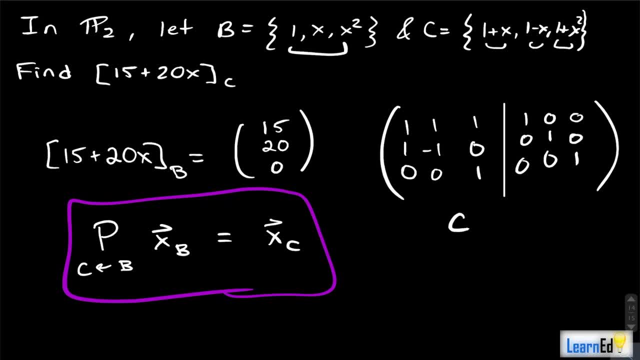 And the reason why I wrote those in this order is because now we have C to B- That's how I remember it right. So we're trying to find P of B to C, and so we write it that way in the matrix. 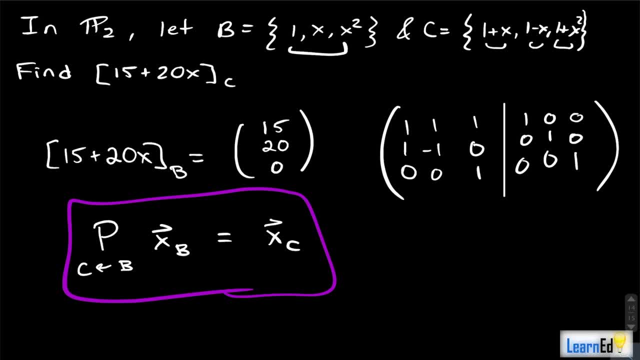 Okay, so here's the deal: When we get this thing to be an identity matrix, we will get P from B to C on this side. okay, Okay, that is the idea. okay, Right now, since we actually have the identity matrix. 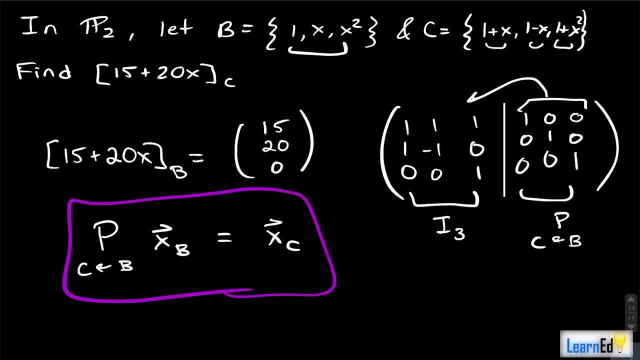 on this side. we have P from C to B on this side, which is kind of interesting, right? So we could actually take the inverse of this thing and then we would have our P from B to C. And how do we find the inverse? 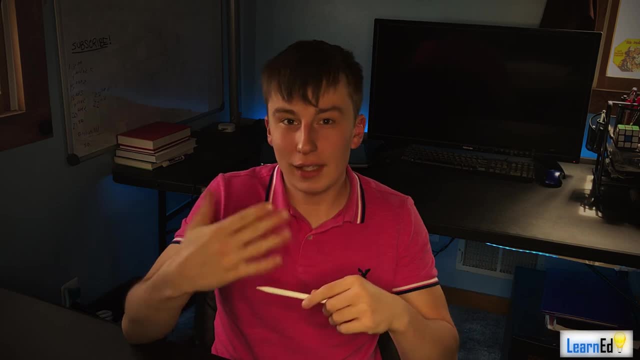 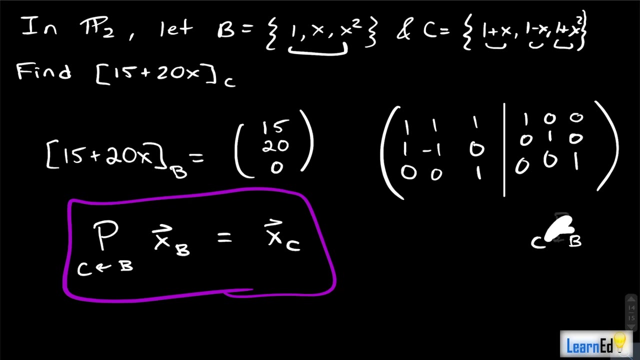 of a three-dimensional matrix. How do we find a three-by-three matrix? We do exactly this. Maybe that can start to ring a couple bells, okay, So it kind of is fitting that we do this. So now what we're gonna do is first off. 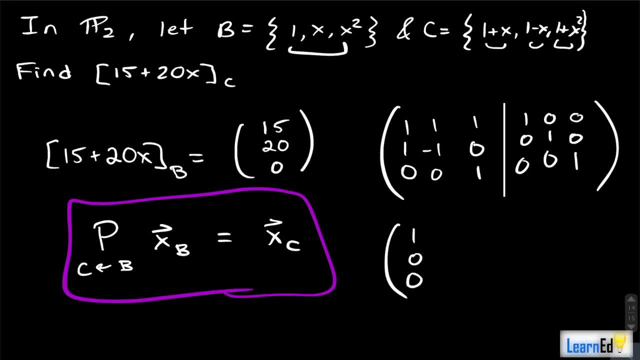 I'll zero off. make sure both entries are zeroed off below the first pivot. The first row stays the same and the third row will actually stay the same as well, because we don't have to make any changes to that To get the second row to be zero in the first column. 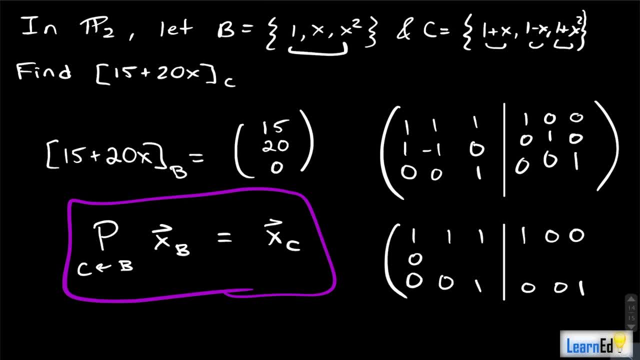 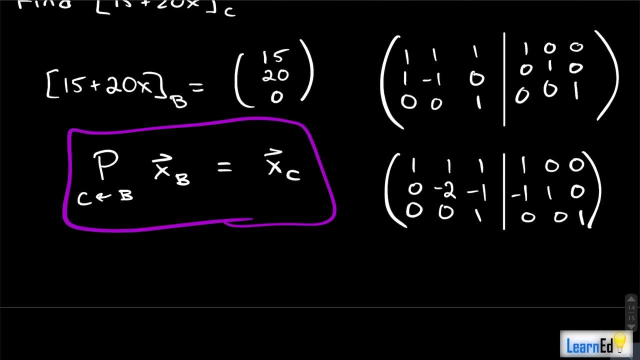 we need to multiply by negative one and add. So if we do that for the second row, we get a negative two here. We're going to get a negative one here. We get a negative one here. We will have just one and zero there. okay. 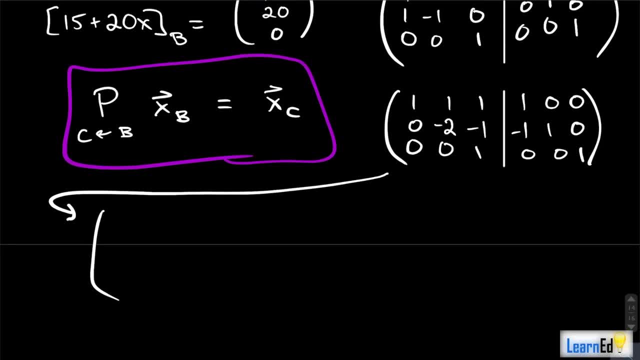 Hopefully you could follow along with that, If we now let's. so we have our three pivots located right. We have our one, negative two and one, So I guess what we could do here is just scale down that negative two to be a one. 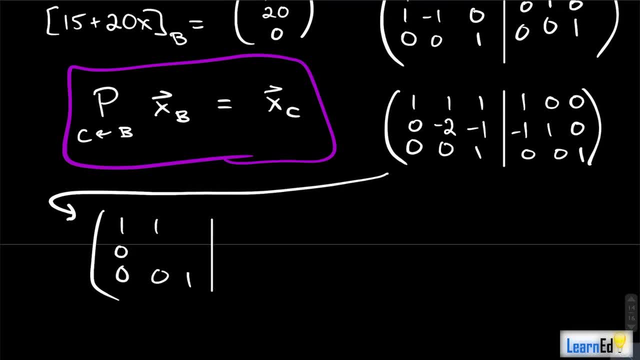 and get. well, let's actually just make sure that our third row stays the same in our first row- Great, So let's make this a one. That means that this is to become a one half. this is to become a one half. 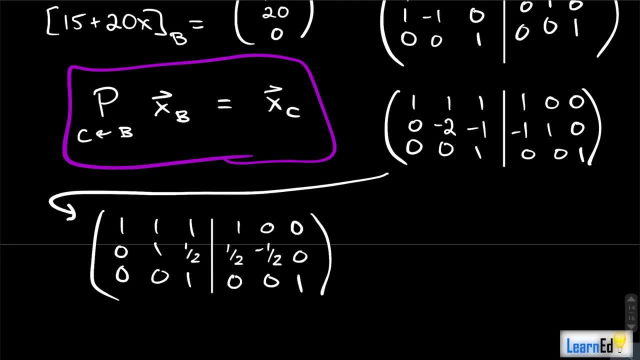 this is to be a negative one half, and this is to be a zero. Okay, so fractions, sadly, will come into play here. I know It sucks, but we're going to do this because we're champions. God, shut up. 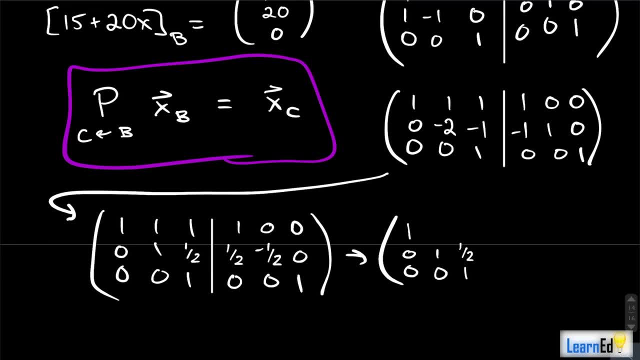 Stop talking. It's bad enough when you have to tell yourself to stop talking, but anyways, what we're going to do now is we're going to zero out this entry. So actually, in that case, I'm getting everything rid of. 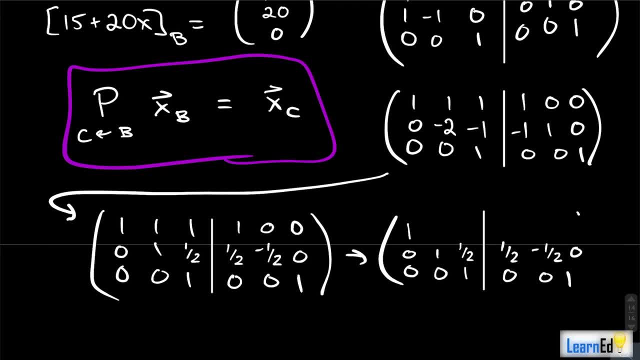 getting rid of everything there. I don't know what I'm doing anymore because I'm just talking about dumb stuff, But if we zero this out, we have to basically multiply row two by negative one and add, So we get a one half here. 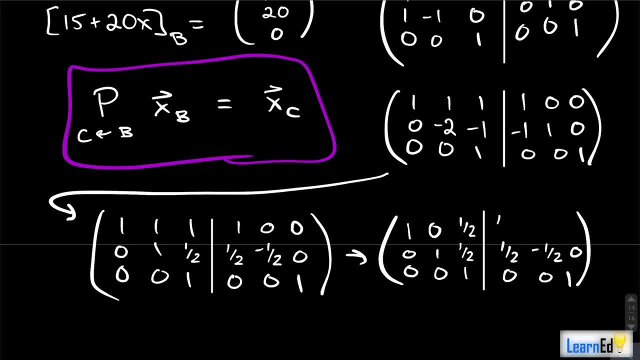 We get a one half here. We multiply this thing by a negative, so yeah, one half there, And then, multiplying this by a negative one, we get a one half, adding it on, And then we get a zero here. 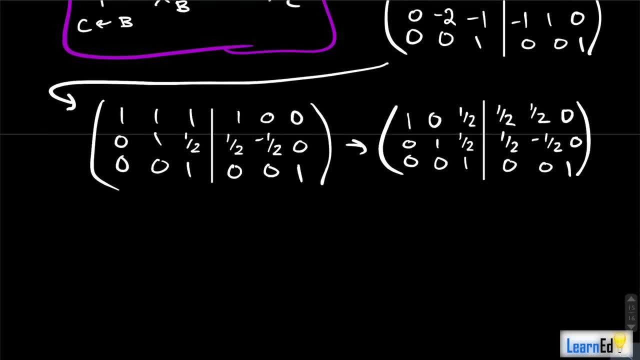 Okay, and the last thing to do is zero off the third column, except for the pivot. We get one zero, zero, zero one, zero, zero, zero one, And then we'll still have a zero, zero one here. 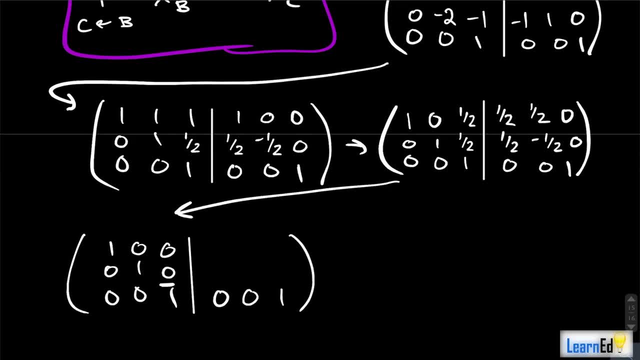 We will have to get this thing to be zero. we need to multiply this one by negative one half and add Okay, so that doesn't actually change anything in the two first columns in the augmented section. Again, because these things are zeros. 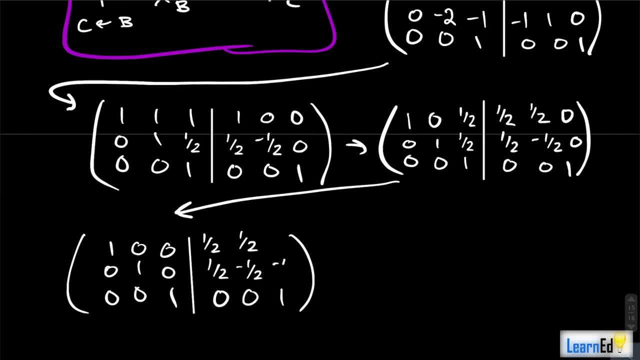 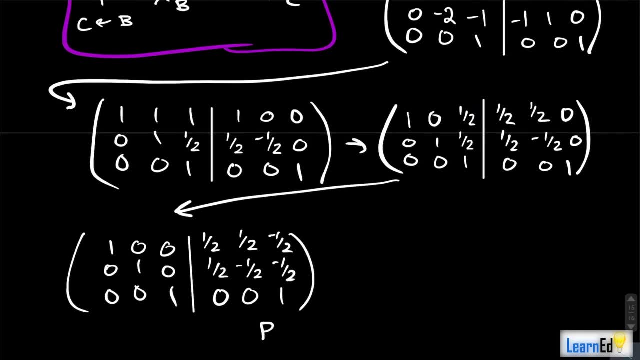 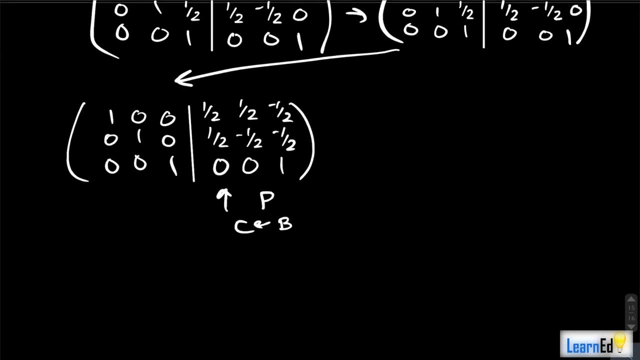 But then, multiplying one by negative one half, we'll get a negative one half here and a negative one half here. Okay, so we finally have P of B to C. Okay, it's that mess. So we're going to take that mess. 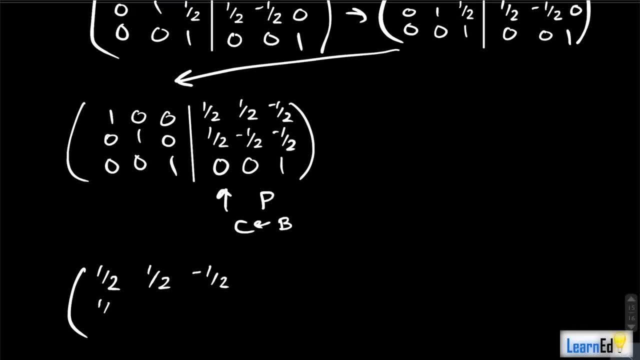 oh, that's not a two, don't know what that was. okay, we're gonna multiply by that vector. we had earlier 15, 20, 0, okay, so we have 15 times 1 half, 1 half 0, plus a 21 half negative 1 half. 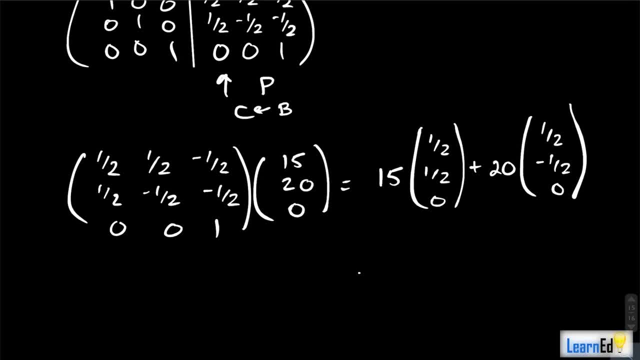 0, we don't need to worry about the other one because it was 0, so we get a 15. halves 15 have 0 plus a 20 times, so we get 8, 10, or we can actually just write this as a 20 over 2 negative. 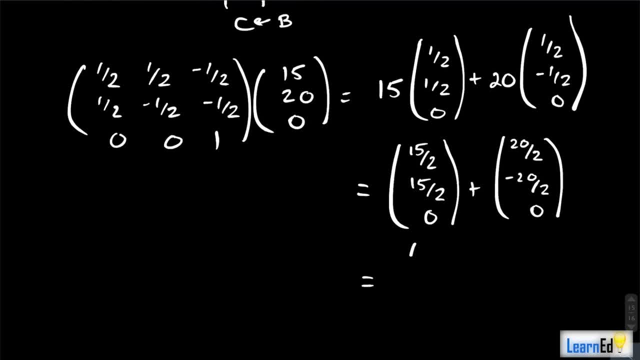 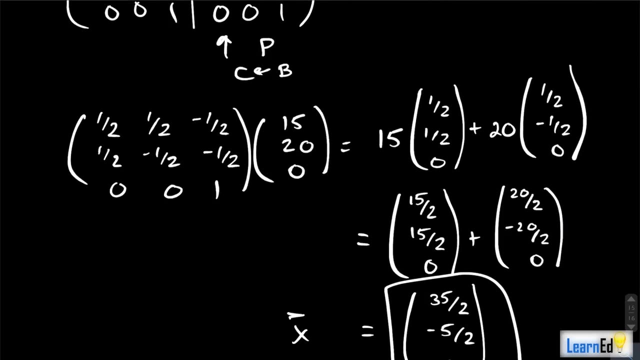 20 over 2, 0. okay. so we'll get a 35 over 2, we get a negative 5 over 2 and we get 0. there you go that right. there is your x vector or your x coordinate relative to C. okay, so you. 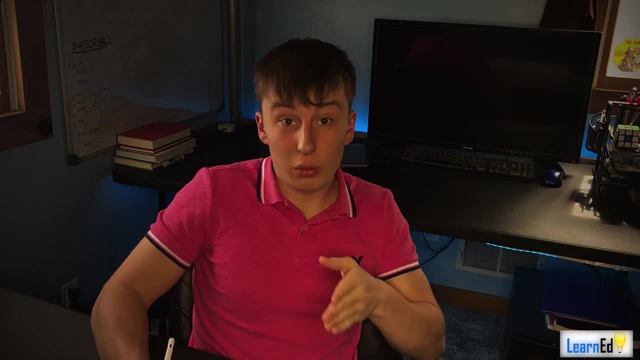 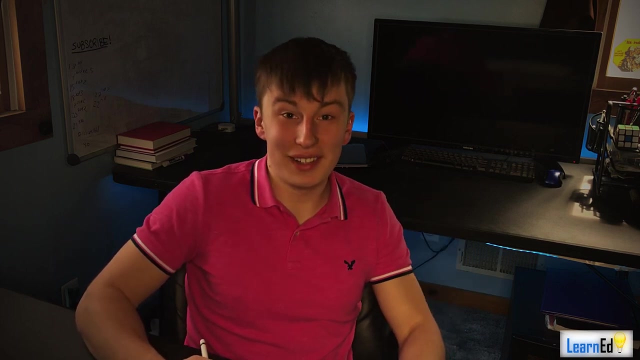 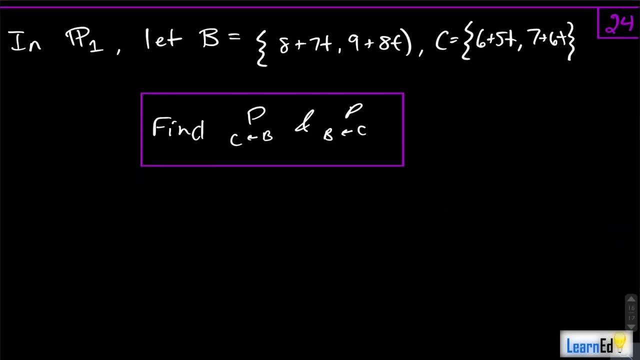 guess, yeah, all right. second to last problem we have in in P 1, let B be. this is a basis: 8 plus 7 T and 9 plus 8 T, and we have C, that's 6 plus 5 T and 7 plus 6 T. we want to find our change of. 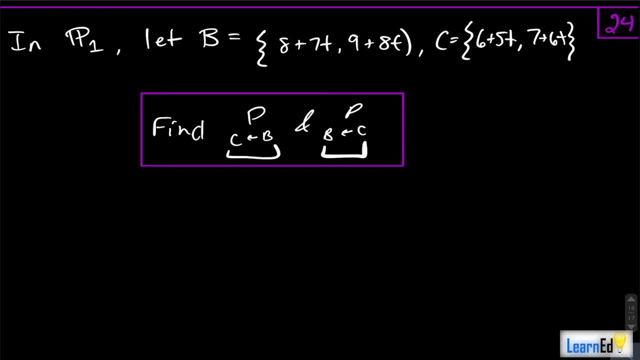 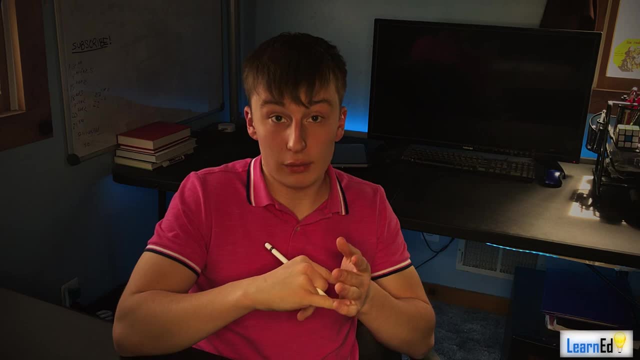 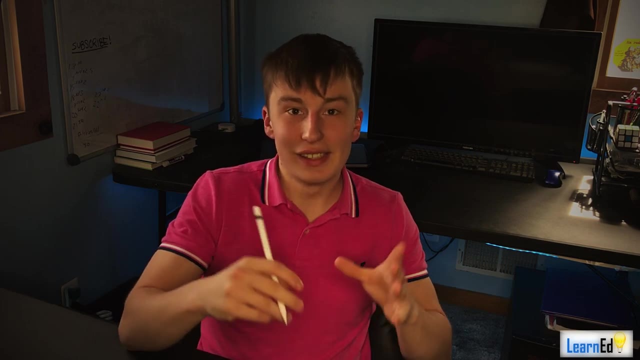 coordinates matrix from B to C and find the change of coordinates matrix from B, from C to B. so this is the exact same thing that we did in problem 23. okay, so now we're really just mastering getting out our change of coordinates matrix, just just just like that. all right, so what we're going to have? 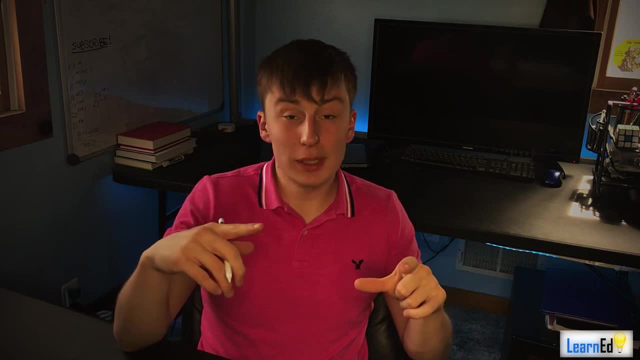 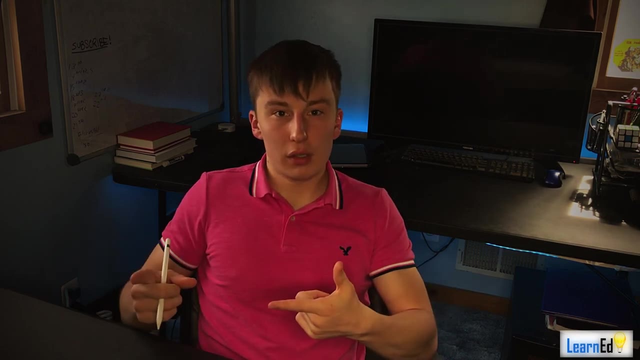 to do here and notice that our, our change of coordinates, matrix matrices are going to be two by two. and remember what I said about the inverse thing earlier: if we invert one, we'll get the other. so actually we're only going to have to find one of these and then it's. 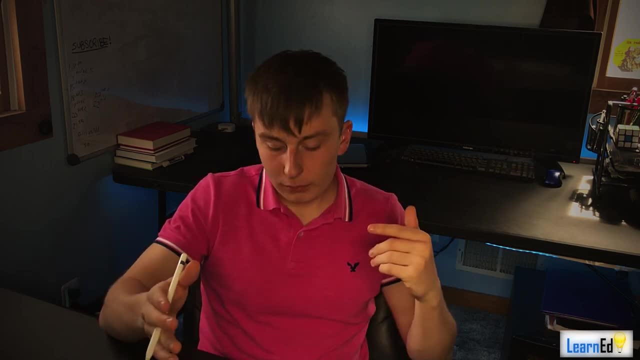 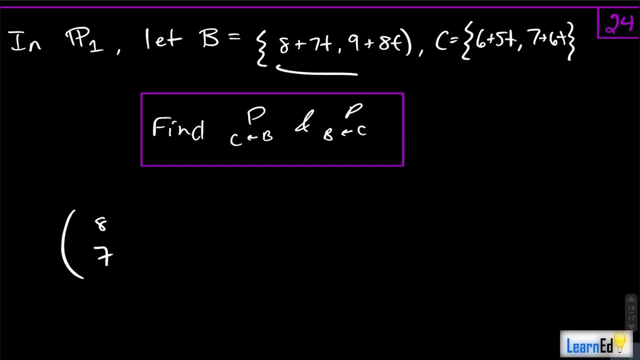 going to be pretty easy to find the other one, okay. so let's get started. so let's do our B matrix, okay, and that'll be nine, eight, we'll augment that with six, five, seven, six. this actually looks like it's going to be pretty nasty to to row reduce, right, but it actually won't be. 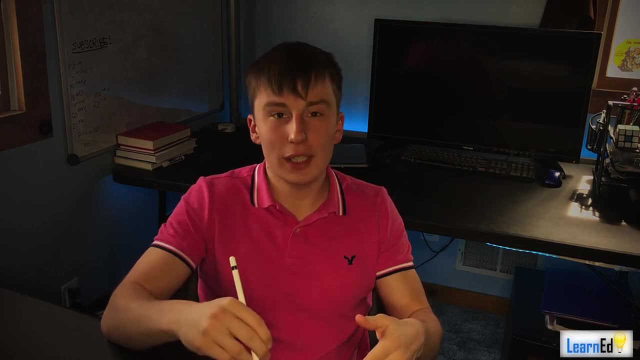 and it's it's kind of you know, if you get something like this, if you're given something like this on a test, I really don't think anybody's going to to give you something like that that you actually have to go through and do disgusting row reduction to get, unless 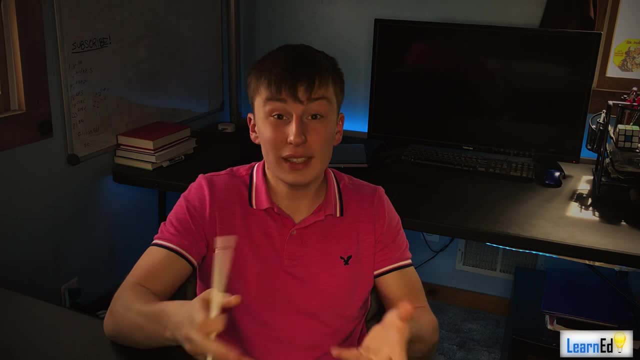 you're given like a calculator or something and still I think it's a pretty harsh problem because it's really tedious and it doesn't test you on any linear algebra stuff. so get kind of suspicious when you have something like this, because there's a much easier way to do that. 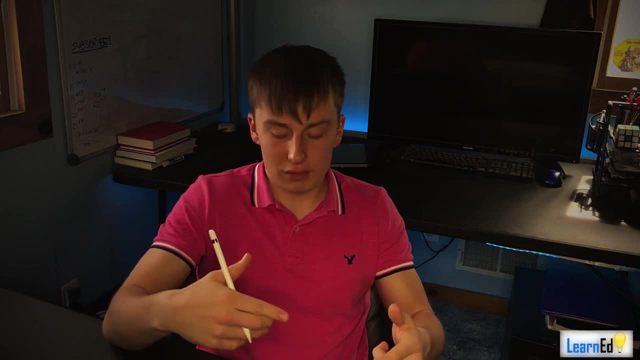 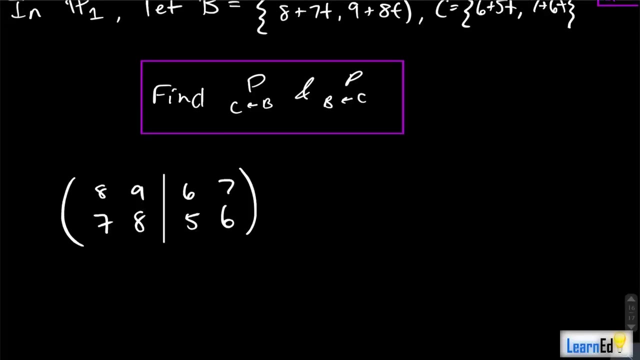 than to do this, than like going through and doing: okay, how do I zero out seven with eight? you know, that's not what we have to do here. what we do have to do here is we can just subtract these, this, the second row from the first row. okay, so if we do that, right, if R2 now. 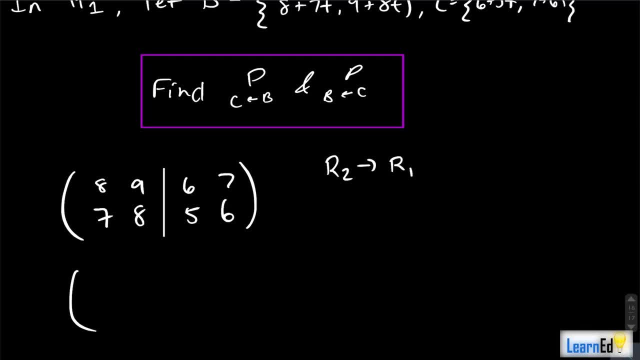 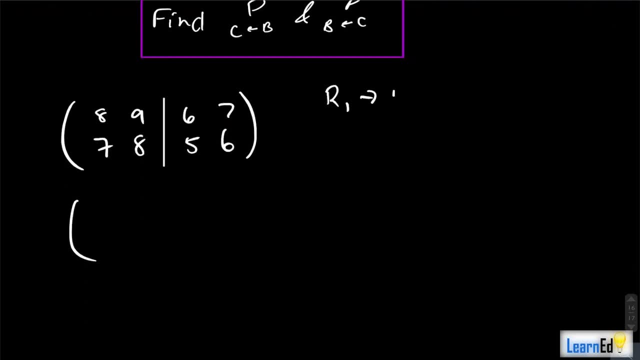 becomes R1, and actually that's not what we can't replace like that. we'd have to do R1 equaling R1 minus R2. there we go. that's something that we can do, okay, and so if that happens, well, what what's eight minus seven? it's one nine minus eight. 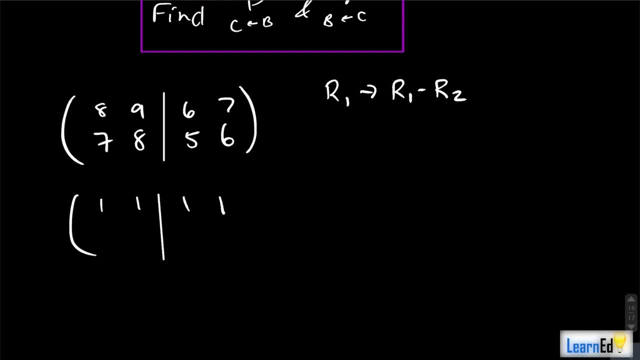 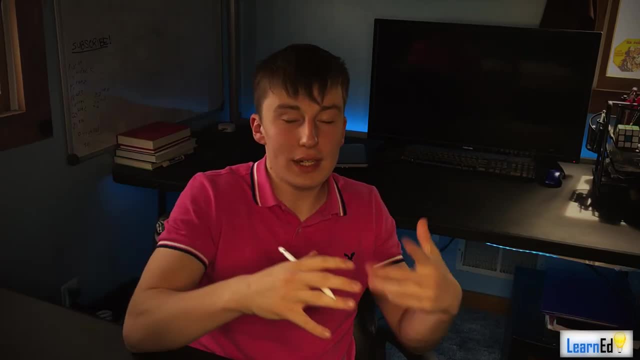 one, six minus five one, seven minus six, one, and then we have seven, eight, five, six on the bottom. so you can row reduce to make something nicer. you don't have to necessarily like zero something out when you row reduce. so it's an interesting tactic and I really. that's why I really wanted. 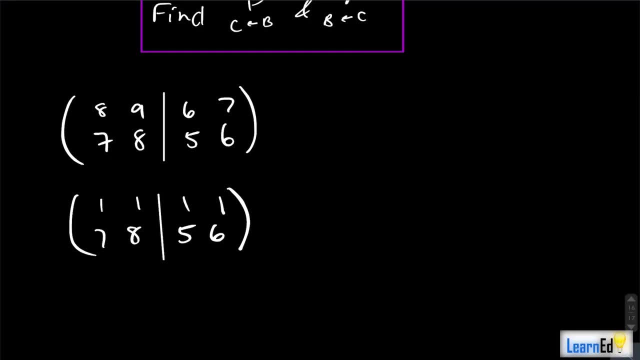 to show you guys this. okay, so anyways, I don't know why I just erased that, because that's important, but we're going to actually start to row reduce now, which will make it all. it's going to be a lot easier now than it would have been before. if we want to zero this seven out, multiply this top row by negative. 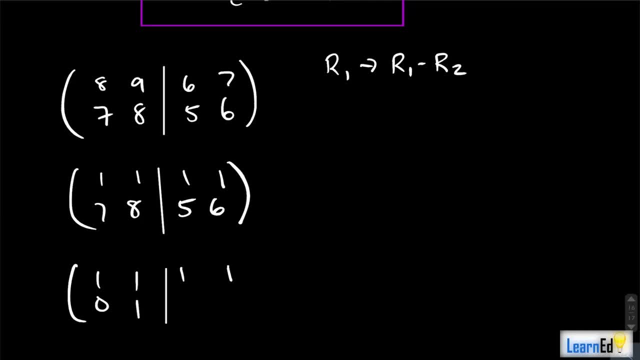 seven and add. so we would get a one here, we would get a, we would get a negative. this would be negative two, and this will be a negative one. okay, and then this thing would become a one zero. we to zero that thing out. that's not a six, that's a zero. geez. 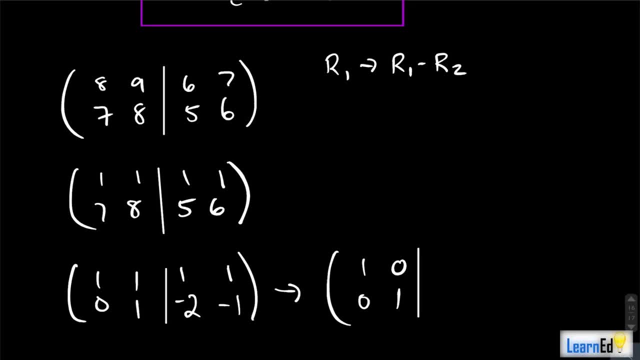 yeah, learn to write God. so this is negative two, negative one. what goes here? well, to zero this thing out, you have to multiply by negative one and add. so, multiplying this negative two by negative one, you get a two, add, you get a three and you would end up getting a two here. okay, 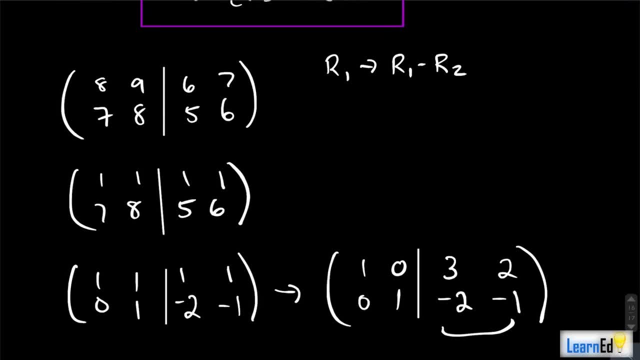 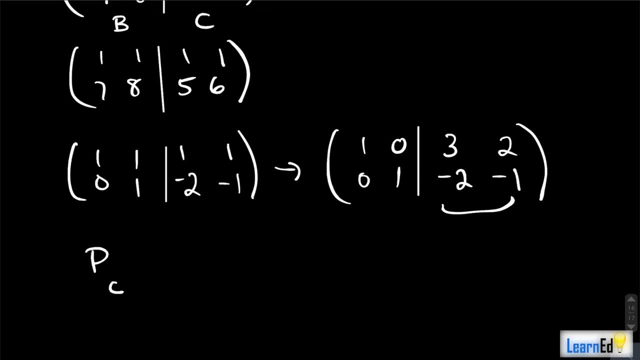 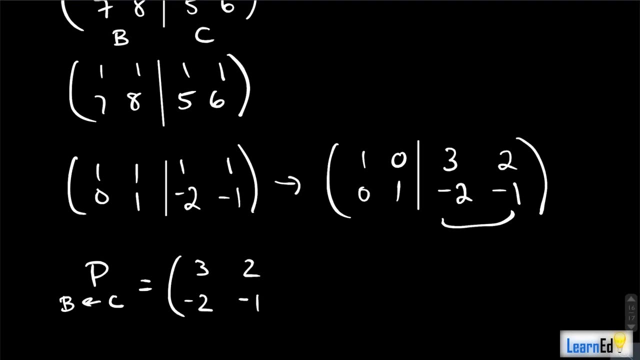 so what did we just find on this side? well, we had B on this side and C on this side. okay, found a change of coordinates matrix from C to B. okay, and that was 3, 2 negative, 2 negative, 1. now we can find the change of coordinates matrix. 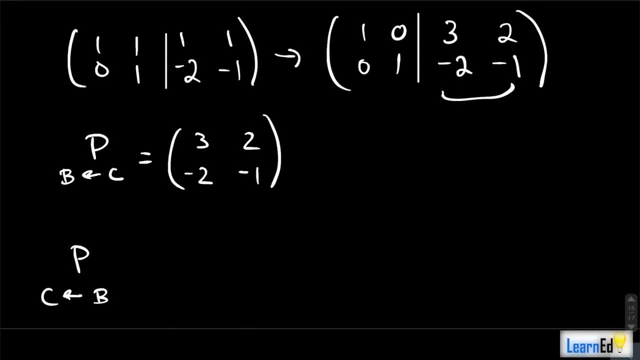 actually I'll write like this- I could. we can find this by just taking the inverse of the change of coordinates, a matrix from C to B. okay, this will just be negative. 1, 3. we switch those two and then we negate the others. okay, so we found this. now, oops, I'll circle the whole thing. found this, found. 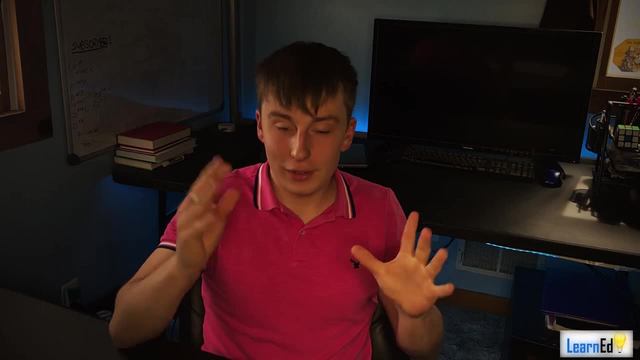 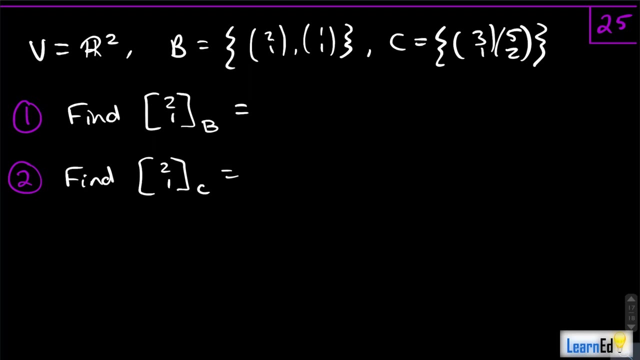 this, we're done, okay, now let's move on to our final problem for this problem. now let's move on to our final problem for this video. all right, so last problem here, problem 25: we have a vector space that is in R 2. okay, vector space V is equal to R 2 and we have two bases. we have B. 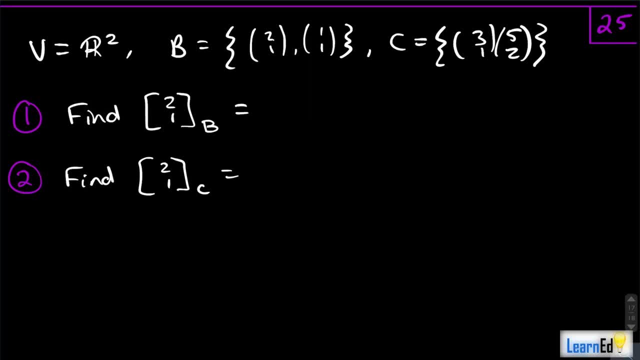 and C and B is defined by 2: 1 and 1: 1, and then we have C, which is defined as 3: 1 and B- 2 and 5: 2. I don't know why I call that a- B. okay, so we're asked two. 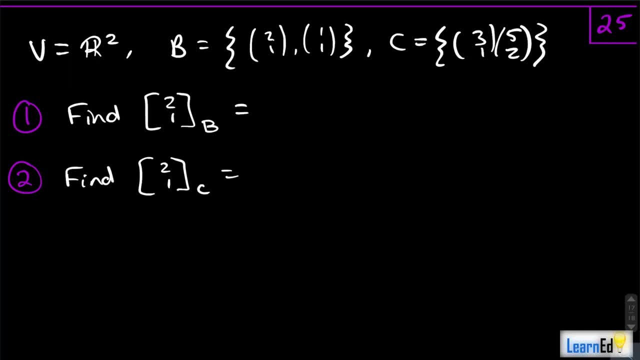 things. we're asked to find 2: 1 relative to B and 2: 1 relative to C. to find 2: 1 relative to B, it's actually pretty easy because there's a 2: 1 right in the in, in the basis B, so you can actually just write this as well. one of these and 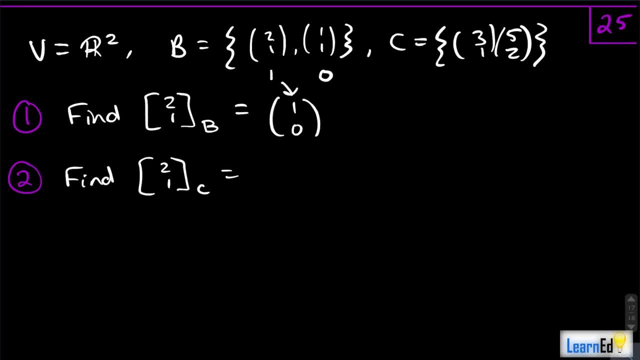 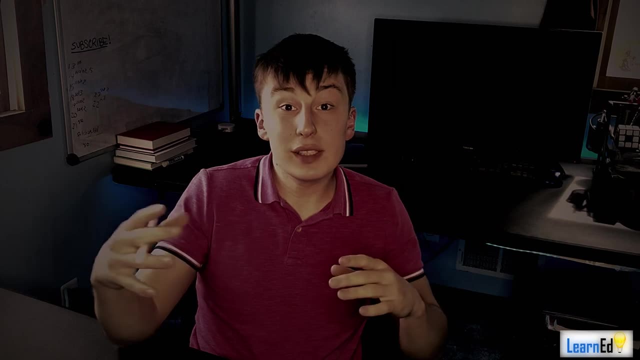 zero of these, so you can put the 1 there and the 0 here, okay, so it actually works out really nice. but for 2, 1 relative to C, how do you do it? well, you could go through that basis B, right, but I mean, like neither of these, these bases are. 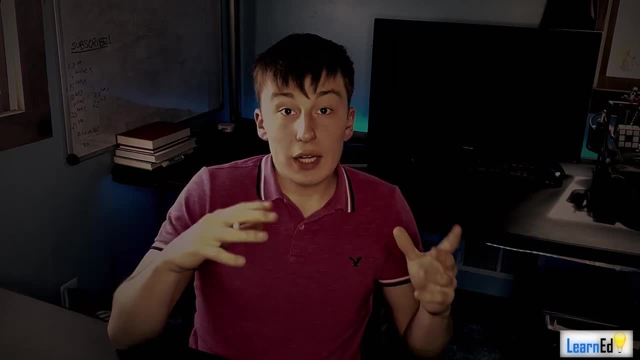 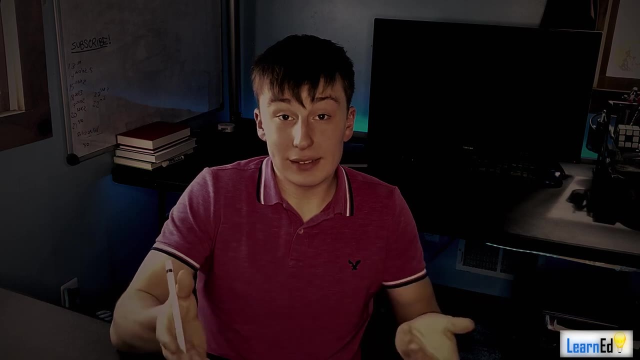 the standard basis. so So you can go through basis B, but what I would do, because it's going to be easier, is go through basis the standard basis anyway. okay, What I would do is, well, 2, 1 relative to C. 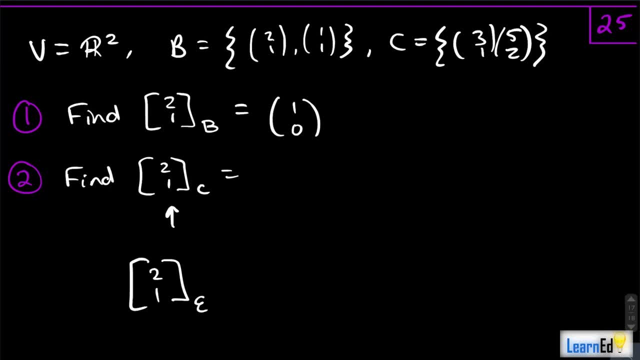 2, 1 itself is relative to E, right? Because you're trying to find what 2, 1 is relative to C. You're trying to find this, But you know that 2, 1, these are coordinates of the standard relative to the standard basis, right? 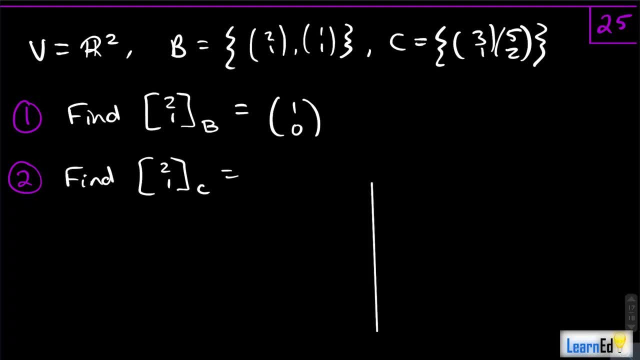 So you're trying to- I mean, let me even graph this out to hammer that point home even more- You're going over 2, and you're going up 1, and you have a vector here And you want to find what this vector is pointing to relative to C. right, 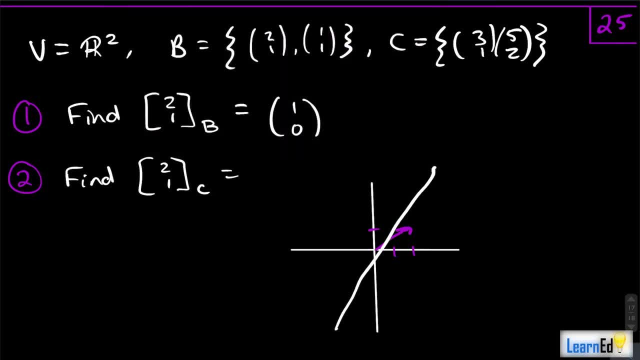 So you know, maybe with C your y-axis is doing something like this, And now everything is different. What we need to do here? we can establish a change of coordinates matrix, right, Because we know here that, since these two vectors here are relative to the standard basis, right? 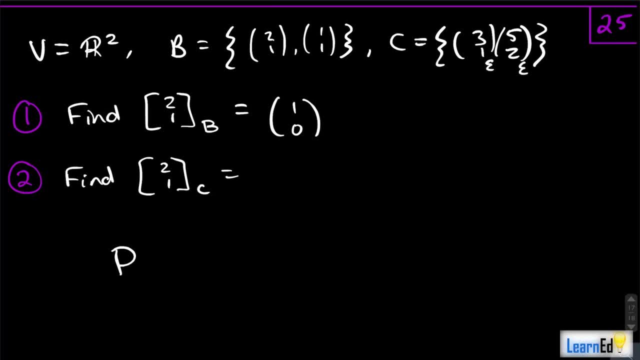 That's how we're defining our new basis. That's how you're always going to see the new basis defined. most likely We know that, and from the change of coordinates section as well, that this is the standard matrix from C to E right. 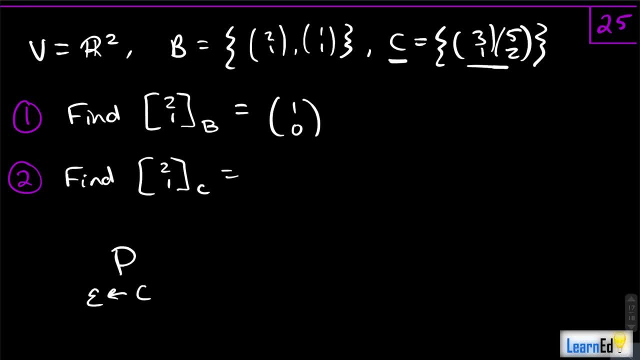 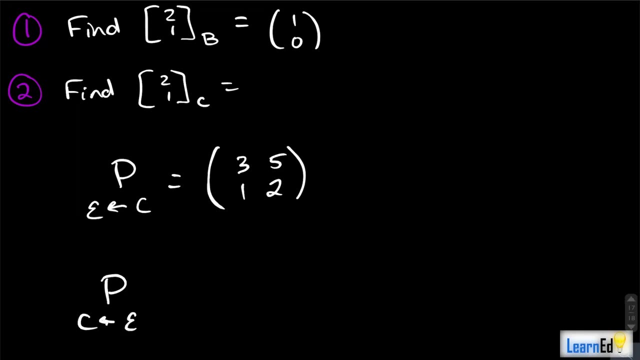 Right, This is how you get C from E. That's kind of essentially what this is saying. So this would be 3, 1,, 5, 2.. But that's not what we want here, because we want the change of coordinates matrix from E to C. okay, 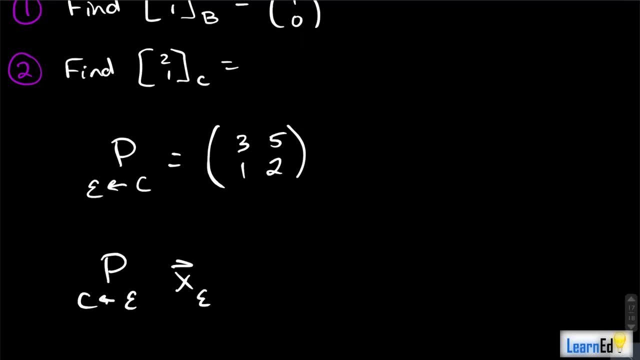 And the reason why is because we can multiply by that change of coordinates vector relative to, or sorry, the coordinate vector relative to E, and we get the coordinate vector relative to C. right, We get 2, 1, C. Okay. 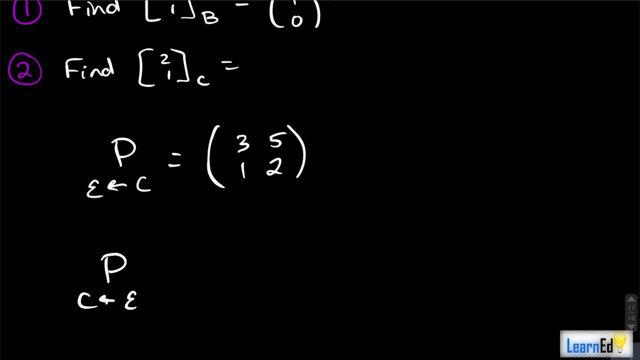 So how do we find the change of coordinates matrix from E to C? Well, what we do is this is just the inverse of this matrix, so we invert it. We have a 2,, a 3, and this is negative. So we just multiply this by 2.. 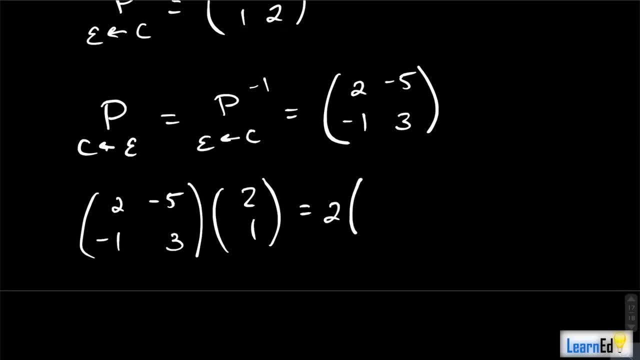 We have a 2, 1, and we'll get our answer. So we have 2 times 2, negative 1, and then we have a 1 times 5, negative 3. And this is equal to we have a 4,. this will become a 4, minus 5 is negative 1,. 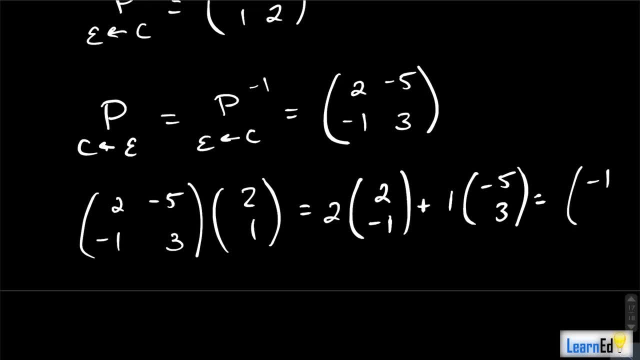 and we have a 2 times negative. 1 is negative, 1, plus a 3 is, let's see, negative. 2 plus 3, sorry, Negative. 2 plus 3 gives us a 1, and there you go.